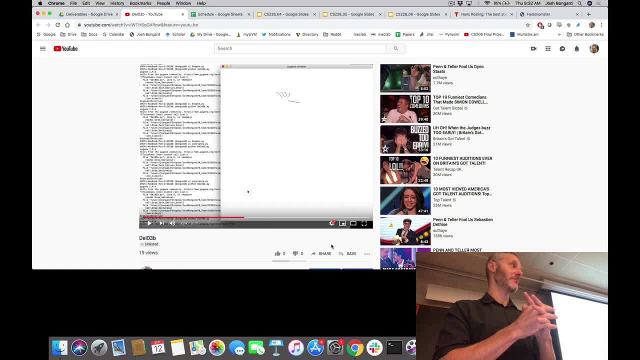 Yes, Yes, Yes, Yes, Yes. At the end of week 10, we're going to have 59 instances of digits, 0 through 9.. And hopefully there's enough diversity in this class that when you have a new user come along and sign one of the digits between 0 and 9, your machine learning algorithm will recognize it. 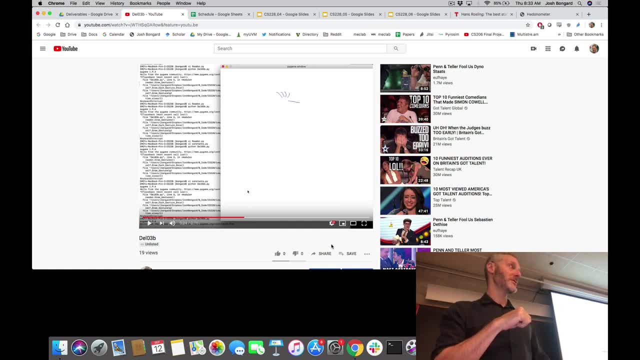 If only you are recording other gestures and someone else uses your system, it's going to be much harder for the machine learning algorithm to recognize that gesture. Okay, You can try it if you want. It could be an interesting experiment. Okay, I think actually part of the confusion about this is: are we asking you to capture X and Y or X and Z, right? 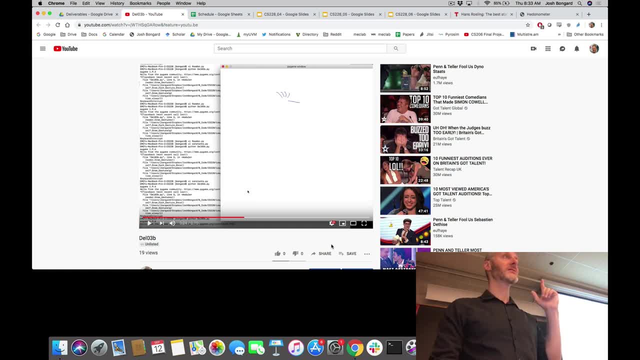 I don't remember offhand from what's in the instructions. Does it say explicitly whether we want X and Y or X and Z? You said X and Z in the second order but X and Y in the third. Okay, X and Z in the second deliverable and X and Y in the third. 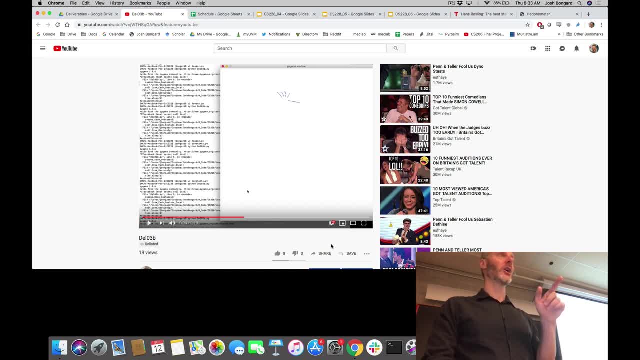 Okay, Okay, three. that's what goes, because deliverable three is where you're starting to record data. so if it's x and y and deliverable three, that's what you're capturing. if you have a look and it's ambiguous, send me a note. i'll update the deliverable and send around an announcement on blackboard. but for 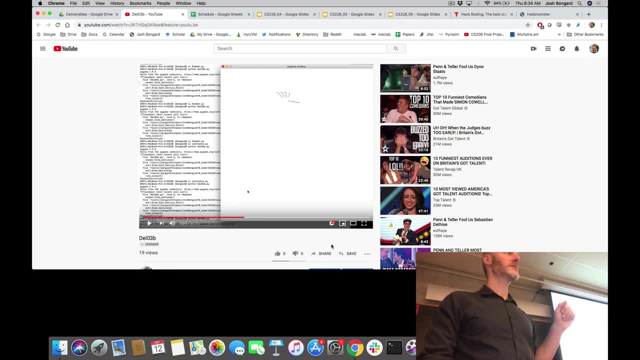 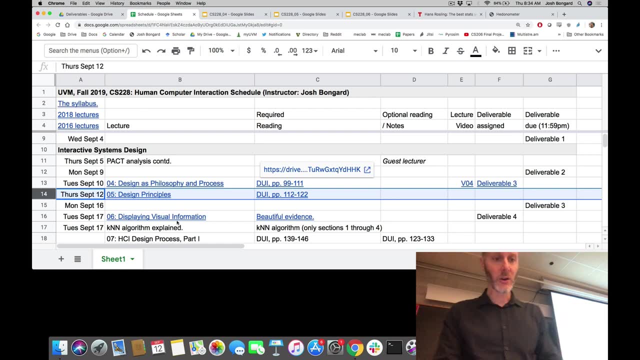 now x and y. any other questions? all good, okay. okay, thanks for that clarification. that was useful, okay, so back to the lecture material. we're working our way through hci design and last time we looked at design in lots of different domains of human endeavor, starting with very subjective domains. 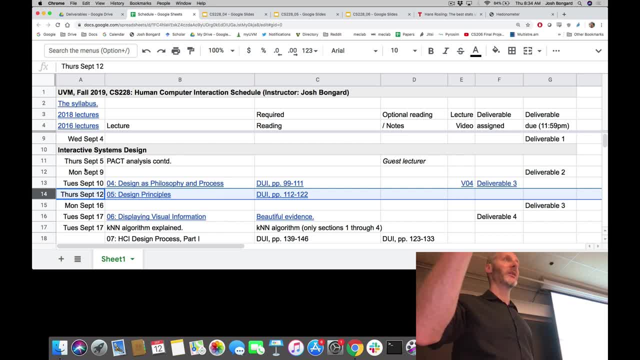 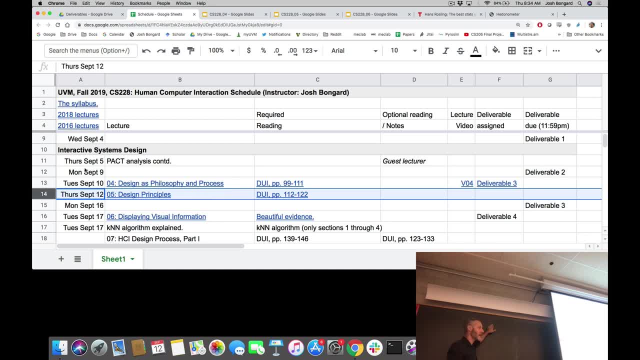 oriented. we're going to try and, in the first step of design, write a description of the system: what it should and shouldn't do. that description is usually made up of functional requirements. we need to describe, when we build the hardware and software, what exactly should it do and what? 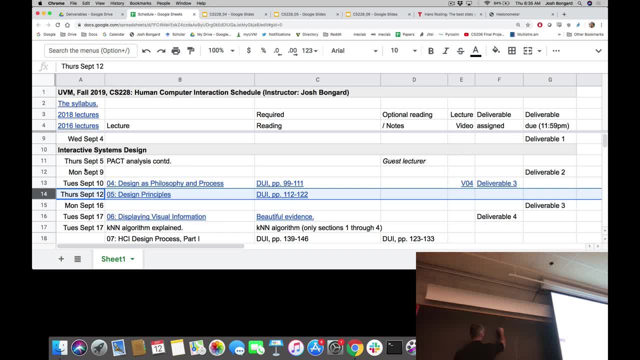 shouldn't it do? last time, we introduced this idea of non-functional requirements, so these are requirements that the system should have but aren't directly about the function itself. what were some of the non-functional requirements we talked about last time? we introduced four of them and we started to move along through them. 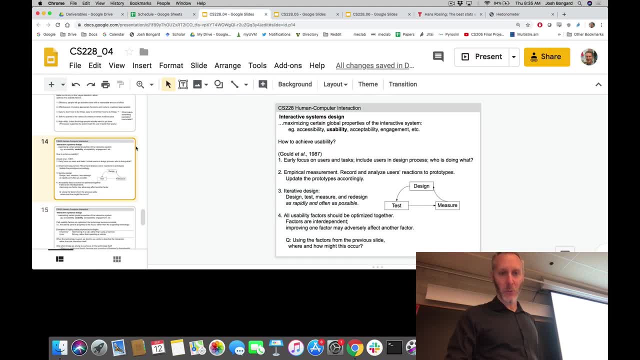 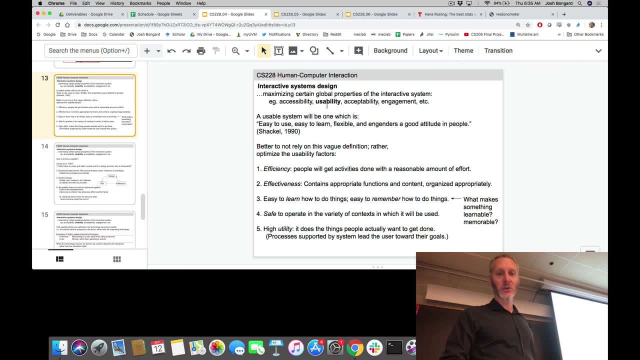 efficiency and effectiveness. those were parts of what we were talking about last time. i'll just back up. we were talking about efficiency and effectiveness, which are sort of again a deeper level underneath usability. so we were looking at these four general classes of non-functional requirements. 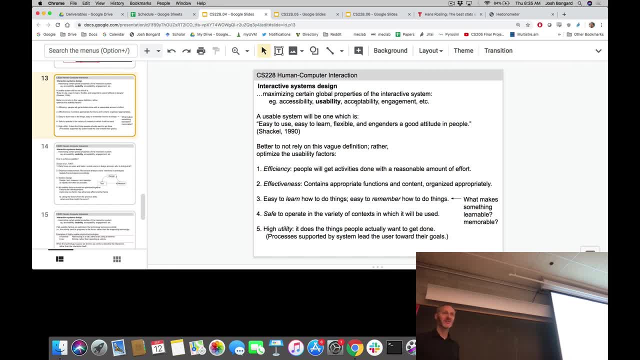 accessibility, who can use the system and who may be unintentionally excluded from using the system. we finished last time by talking about various factors of usability: how easy is the system to use? how efficient is it? does it have high utility? can i use the system? if yo're gonna use it, 사�listing aRYOju knife in my hands, i think you're lost in your сistemy. i was kinda same question. quick, find a tool and find one without one. try to find one instruction: click the sign up icon on the non-functional requirements, otherwise you would use it, help it problem-fician. use the system and get your san�� i. i could have only a use-faction. issues that any to us and unit menteوق t. 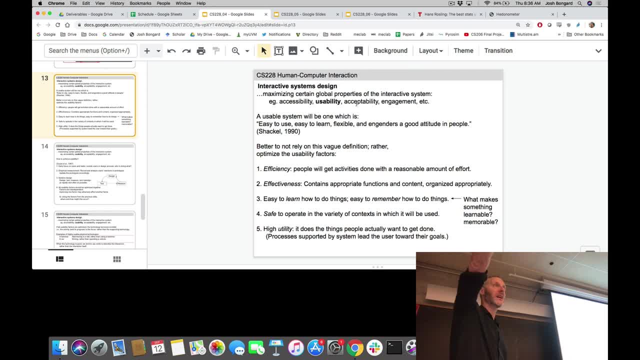 the system I'm trying to get to point B. can I use the system to get to point B, or is this system not designed very well so it actually kind of takes me to B primes- not quite what I wanted to do, but pretty close. we'll talk more about. 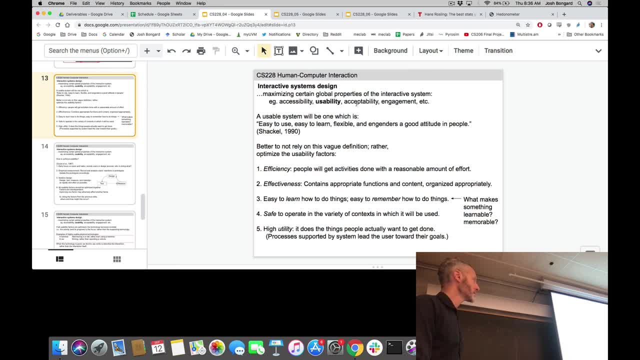 learnability and memorability in a little bit. safety is important, and we'll talk shortly, in a moment, about acceptability. and, finally, the most sort of subjective aspect of non-functional requirements, which is engagement. we'll talk about that in a moment. okay, okay, so we're taking these very general vague. 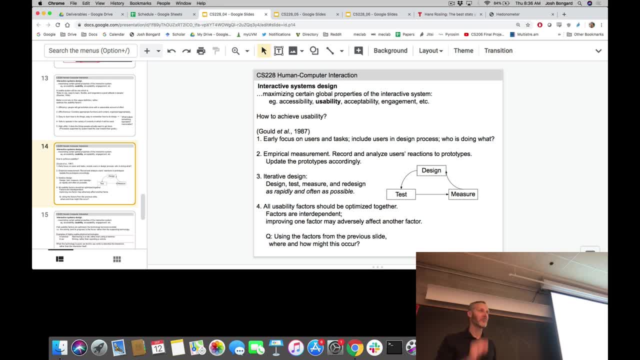 concepts and iteratively unpacking them into more and more specific descriptors, and we're trying to march down to a level of specificity where we can finally start to measure these things. so we'll spend a fair bit of time when we talk about user testing, about empirical measurements. what sorts of measurements? 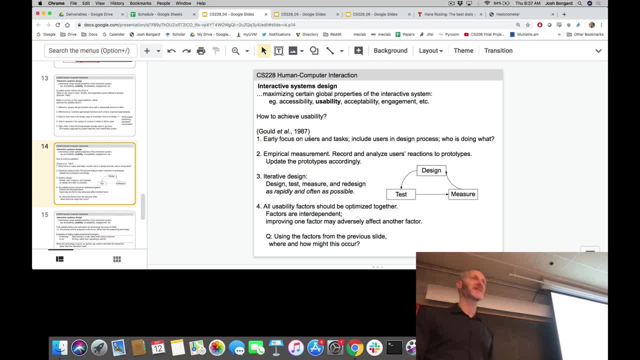 might we use to decide whether a system is accessible? we hope that our system can be used by large numbers of people. we're not sure. we deploy our system out into the world as an app and people download it on their phones. we start to collect data back. what aspect of the 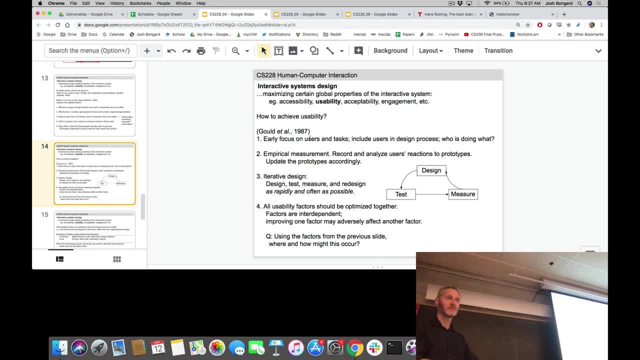 data could we look at to measure accessibility. you could look at your demographics, right, assuming people are willing to share that information with you, which they may or may not, be absolutely right. so we're going from something very vague down to something very specific that we can measure. okay, I think I've already. 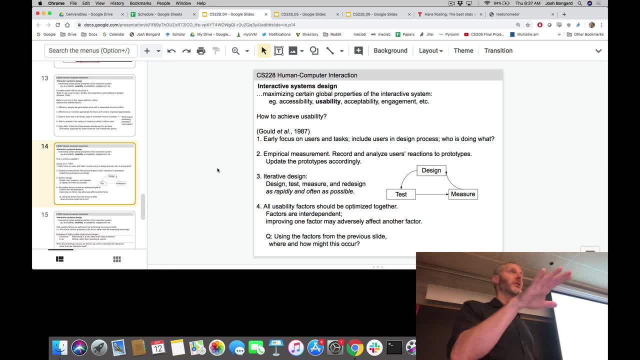 mentioned this several times now. in the Leap Motion project we're going to be collecting data from 59 hands, but among that data set of 59 hands there are going to be some minority subsets of data. what are those minority subsets? lefties, what else? there's another important one. 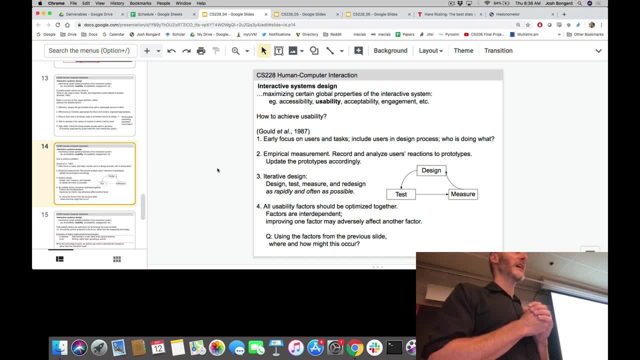 that you will definitely come up against next week, in the week after, when you're trying to train your machine learning algorithm on this data set. male and female, we're going to have a minority of small hands and a majority of larger hands. if you have a minority in your data set, if it's biased- and this is a 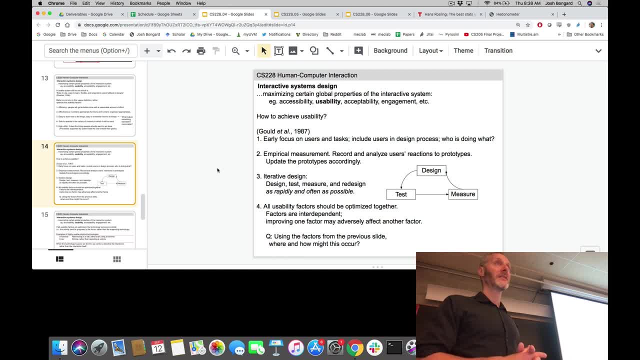 big topic now. in AI you have a biased data set through no fault of the machine learning algorithm. it's going to have a hard time recognizing, dealing with classifying the minority data set. so we may end up excluding some users from your system unless we compensate for that bias in the data when you deploy your ASL educational software to 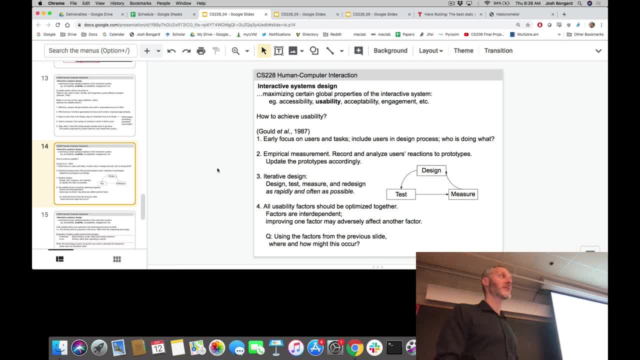 your friends and family. in week 11, females are going to have a harder time using the system than males. okay, we're going to. we finished last time by talking about the fact that some of these factors are sort of they play against one another. they're antagonistic. if we're trying to make the system 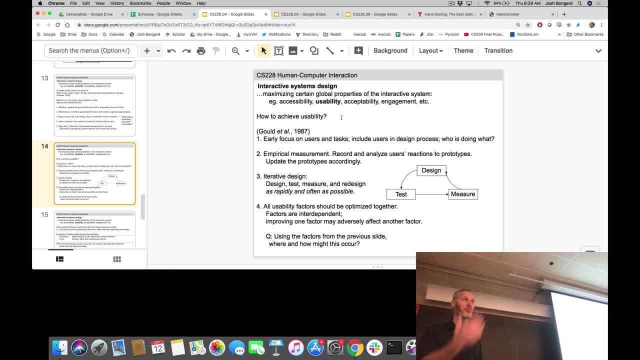 accessible as possible. we want to measure that through demographic information. we're asking people for gender data right, so now maybe it's not acceptable to people because they don't want to share that kind of information. a lot of these factors, even if we can nail them down to specific measurable items. 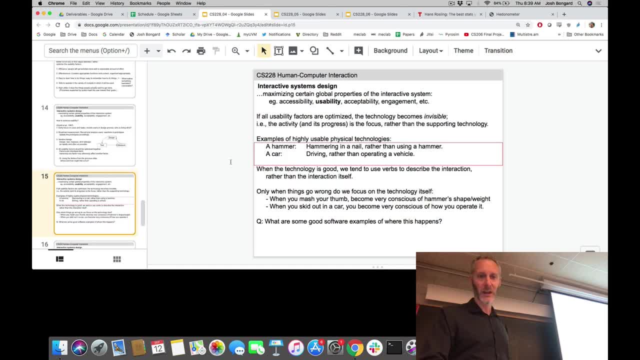 they are antagonistic. okay, how do you know whether your system is usable? sometimes we're collecting statistical data from users using our system. sometimes we're collecting statistical data from user. Sometimes we're asking them to just talk about the system. If we ask them outright whether you like the system or not, they'll say yeah, it was okay. 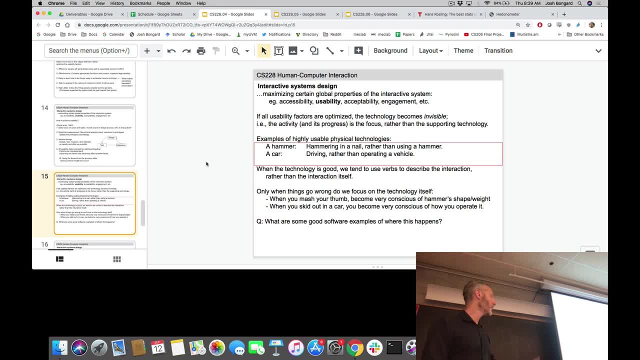 or no. it was kind of frustrating. That's not very useful data. You might step back and say: tell me about your interaction with our system And there's hints in the way people use language to get a feel for whether they enjoy the system. 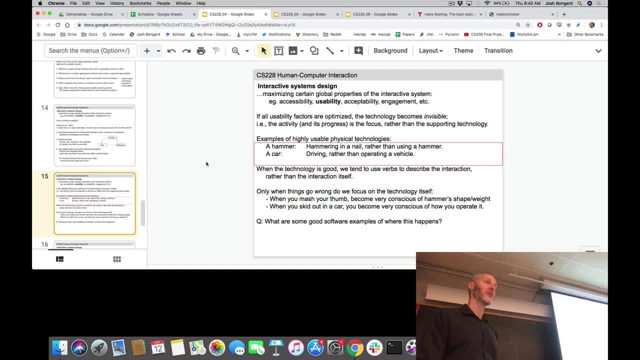 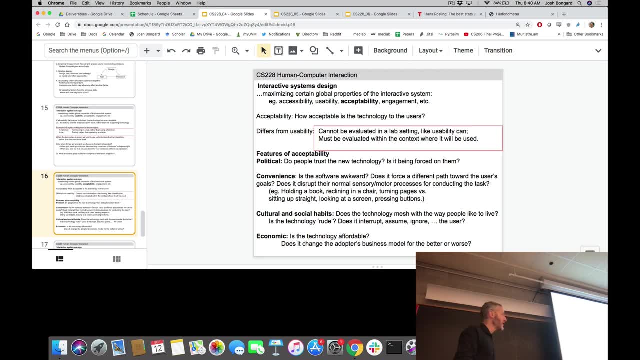 whether it's actually working for them, are they frustrated, and so on. So we're now going to talk about acceptability and engagement. These ones are harder to measure because they're a little bit more subjective. As I've mentioned several times now, in HCI, we're often trying to play this balancing. 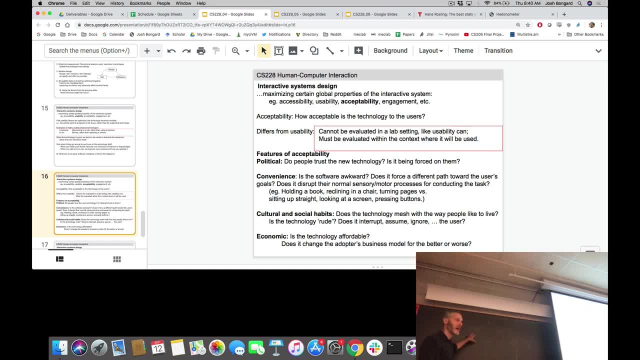 act between meeting our objective goals, making sure that our system conforms to what we want it to do- the actual functional part of the system- with other sort of subjective aspects of them, And acceptability is one of them. You may have a system. 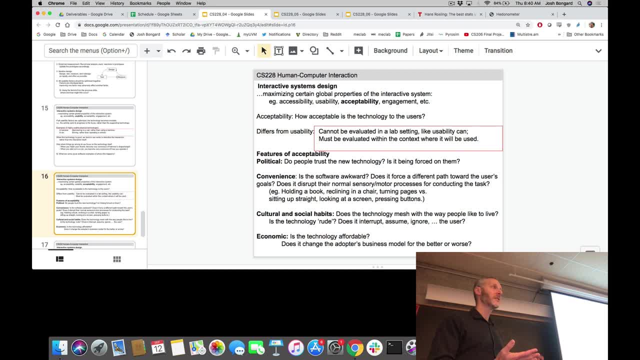 That is perfectly usable. It's efficient, high utility. People can do exactly what they want to get done, but people don't use it. It's not acceptable. So one of the reasons that makes this difficult is it's difficult to alpha test or beta test. 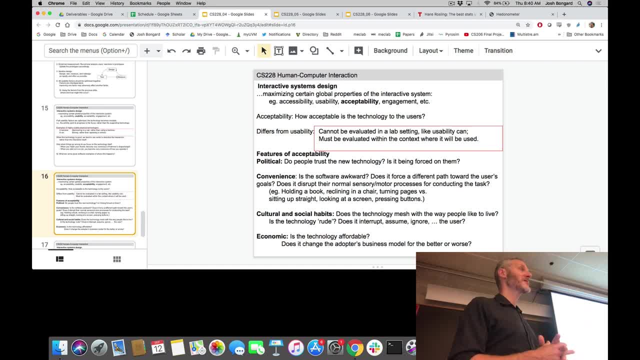 your system in a controlled setting to measure acceptable? because people aren't using your system in a controlled laboratory setting. They're running your app on their phone While they're walking around outside talking with friends driving a car. they're using it in a particular context and it may be that your system is not acceptable in that. 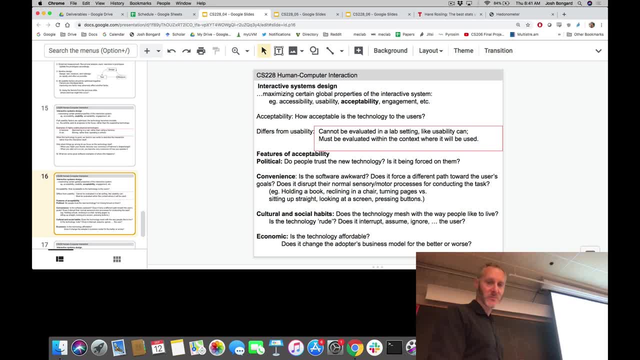 context, You can imagine some various features of acceptability. Do they trust the technology? Are there things going on in the greater context of the technology itself that you may not wish to trust the system? 05.. I'm sure those of you that have the great fortune of using PeopleSoft, which is the 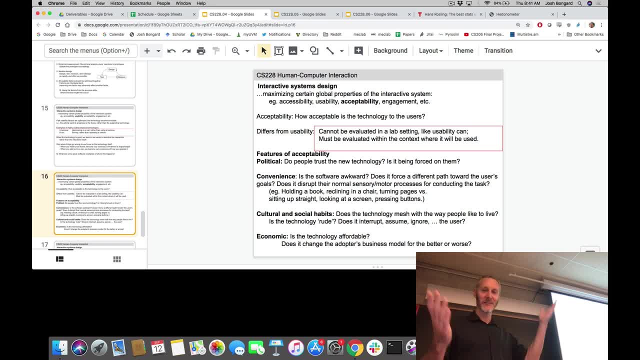 HR software system for UVM- some people are laughing already, you'll know. Not necessarily very usable either, but definitely not very acceptable For us poor faculty. we have no choice. So even if the system works well, there is already a baseline of resistance against this. 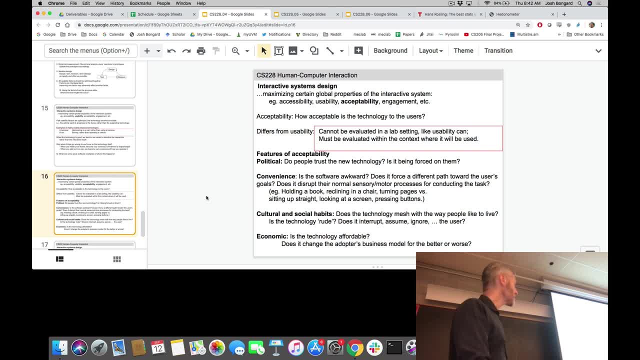 system 06.. Okay, Is this system awkward? 07. Does it force a different path? 08. Does it force a different path from A to B than the user is used to? Before you deploy your technology, the user may have a particular way of getting from. 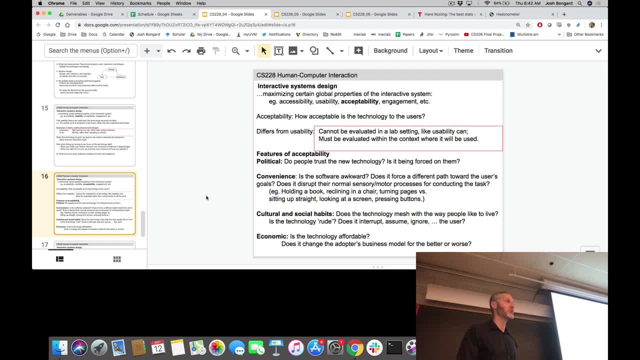 point A to point B. You introduce your system. it's perfectly usable, perfectly efficient, bug-free. It gets them from point A to point B faster, but it's not acceptable 09.. A common example of this in the history of HCI is e-books. 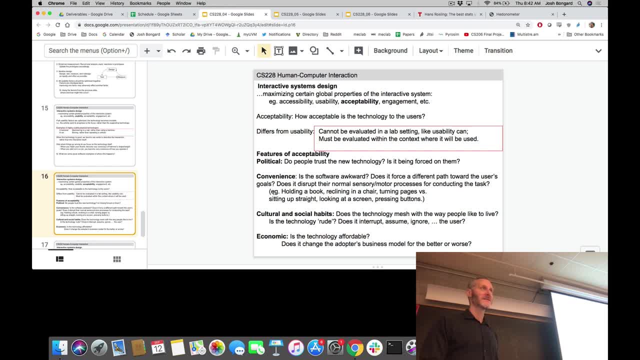 It took a long time to get this right. 10. Next time you're on a flight, look around How many people are reading paper books and how many people are reading e-books. From my count, these days it's more e-books than books. 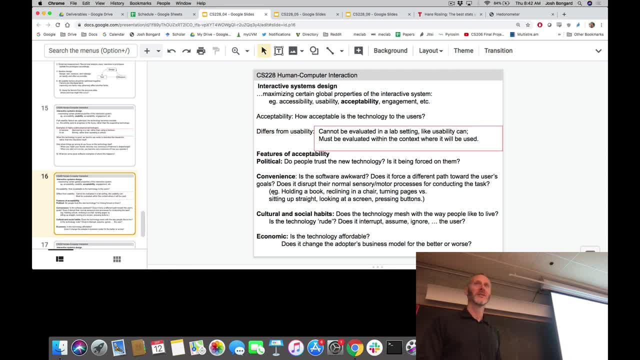 So e-books are finally starting to become acceptable, But it took a long time to get to this point. Why 10.? I think the efficiency and convenience of books has never been considered a design resistance. Profitability is the first factor. What was profitability? 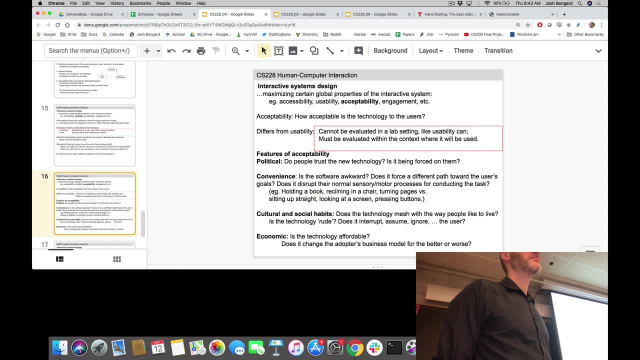 Profitability. Okay, Who's they? Any company trying to make a profit? Oh, I see Adobe actually created a free system. Ah, okay, They were creating secure documents, kind of between point A and point B. Okay, And so they already had the advantage. 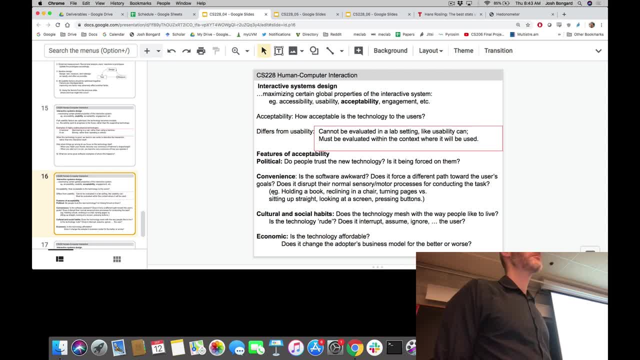 Who had the advantage? Adobe, because it was free. Yeah, They had the freedom to market their brand image. Okay, They used a population that was trying to anyone who was trying to penetrate the market. So there was an economic advantage, An economic advantage for the user. for e-books it might have been cheaper than actually. 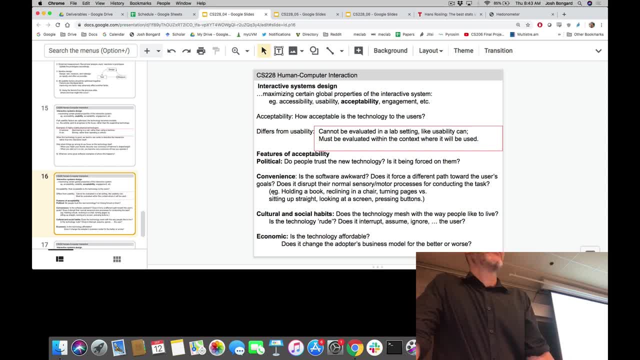 buying the physical book? Right, But it meant medium. It was one that was focused on profit and one that was focused on just promoting the brand, Right? Okay, So we're focusing here on usability. What is it about? or sorry, acceptability. 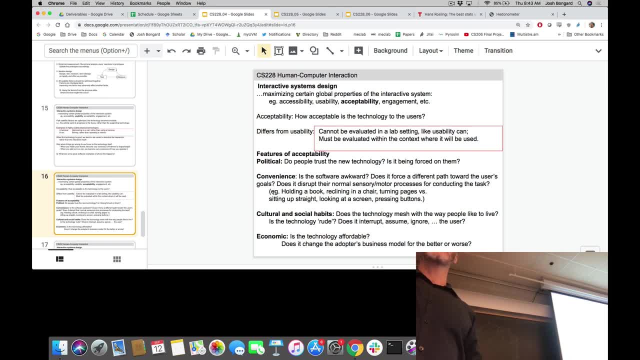 What is it about e-books? that was particularly difficult from an acceptability point of view. Yeah, For reading off of Mac is really Yeah. So what was it about the old tablets that made it not as comfortable as reading a physical book? It was the light, right. 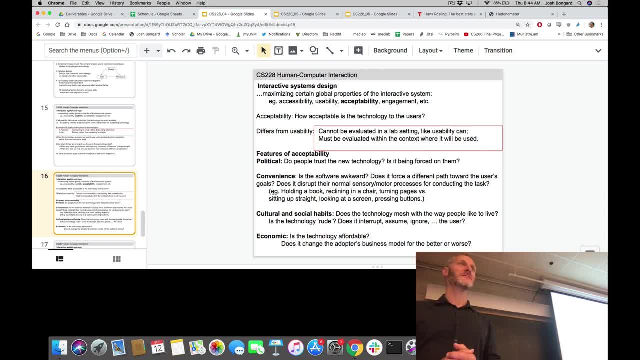 So the page is emitting light at you, So that's kind of been solved. What else? It seems like a detail on the surface, right, But it's extremely important And I don't know if this still exists, but a lot of e-book apps they actually create. 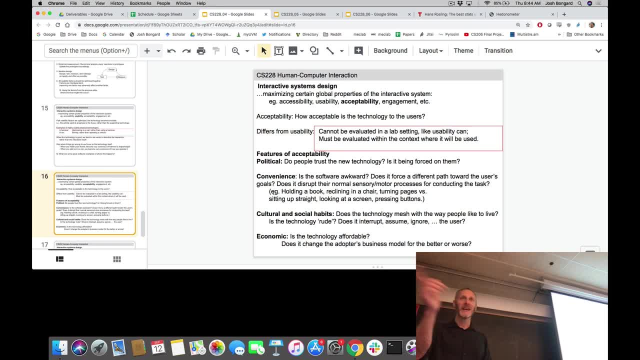 the illusion now of turning a page, And for some people, that's what makes the difference between picking up an e-book and picking up a book. Right, That's an acceptability issue. It's your book, right? Yeah Yeah. 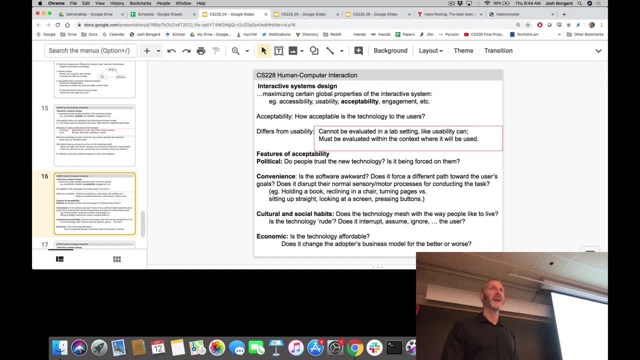 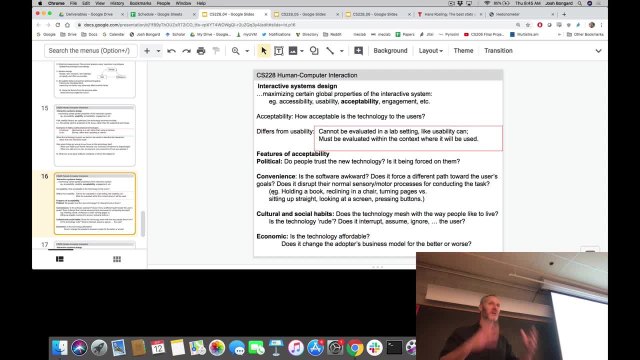 Yeah, Yep, yep, Yeah. ya, It's not generic. It'll need for difficult detail to help it. It's difficult, It's hard to remember everything about them. to be clear is it At least for people that love to read. right, there is a large number of these. 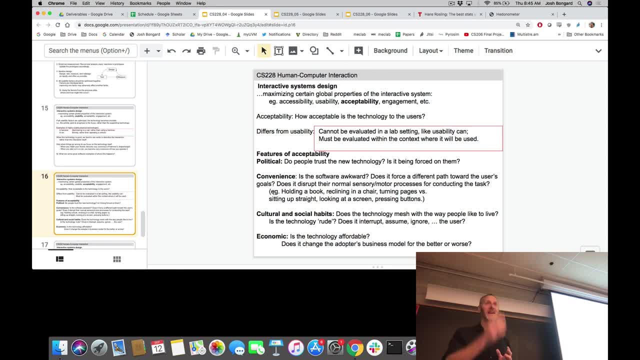 subtle details which are still not incorporated into e-books and may never be Right. Think about your favorite book. You probably had it for a long time. You know that that scuff mark on the book was from when you read it seven years ago. 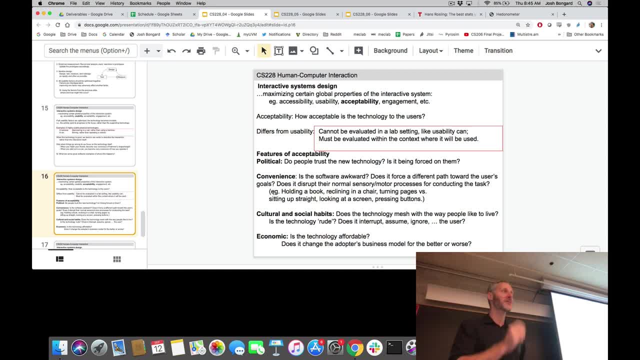 at the beach. and this mark on the book is from not just about the reading experience itself. right, it's. there's something larger that is extremely difficult to get in write in ebooks. so some of the obvious things up front, like lighting and turning a page, those have been solved. but there are still these subtle issues. 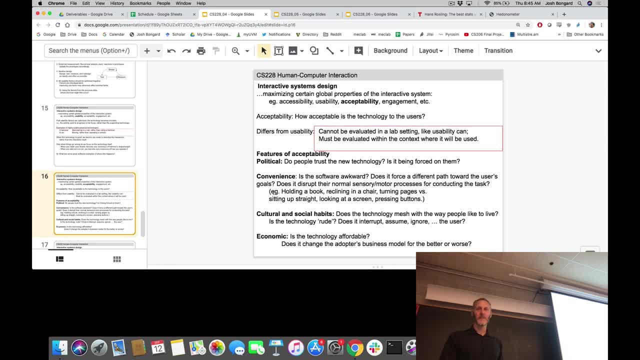 especially for technical books or books that have, um, really great, uh quality graphics, like a photography book or something that sure, if you have a favorite photographer and he goes like strong bookstore, you can in new york you can see really nice prints of close perhaps, but i wouldn't necessarily want that in an ebook, exactly right. so if you're looking at an art book or 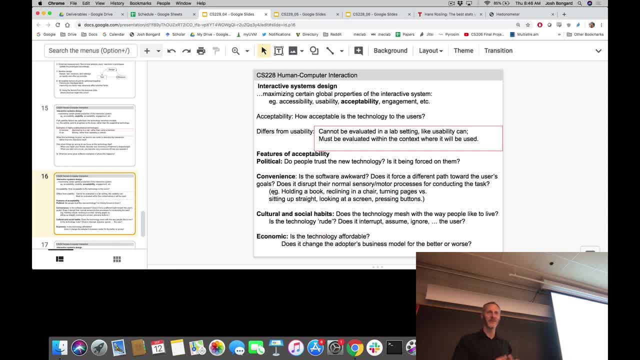 photography book where the quality of the prints is extremely important. there's something also about the physical experience and the aesthetic experience about opening a folio and looking at fine scale prints. that's difficult to get right in a digital medium. the better for worse. people often increase the font files, but that also increases. 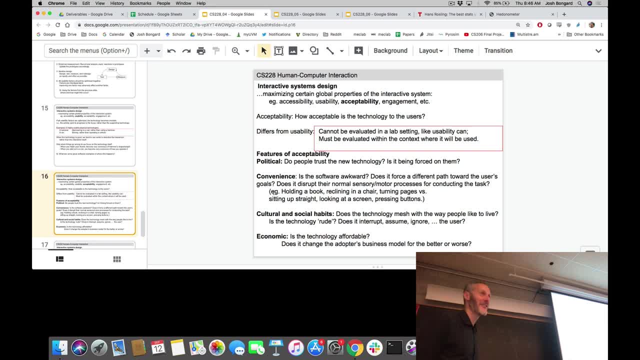 that's a great example, right? so, in terms of accessibility, easily being able to change the font size is really important, right? something you can't do with physical books. that was something that ebooks got right, right, it actually made reading- or at least quick and easy reading- more accessible than physical books, but it also changes some of the acceptability issues, right. 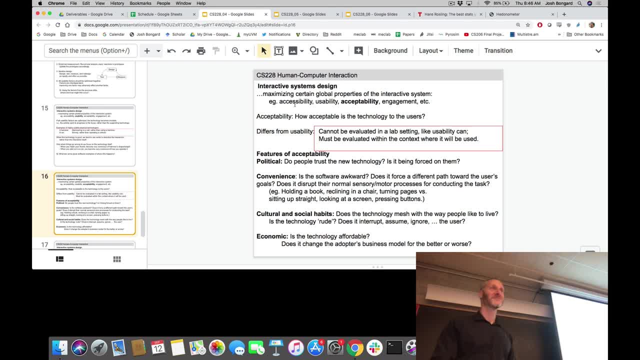 now the pages. the book is 1200 pages long, exactly, so a lot of physical context comes into play when thinking about acceptability. one good thing that ebooks do have is um for code. okay, so in physical books you can't click on the code sample and copy and paste it into a rough. okay, so copying and pasting code is a good thing. 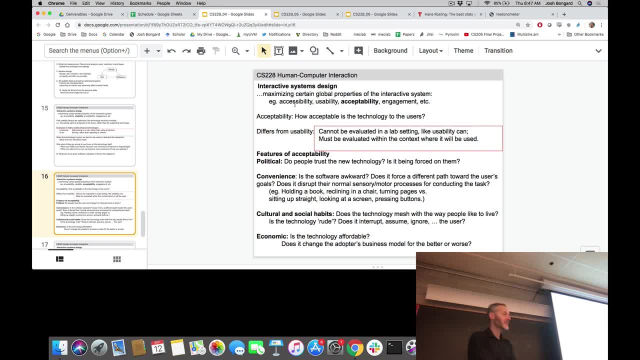 absolutely right. so when we sit down to spec out an ebook, it's what actually is the activity. is it reading a novel? is it looking at an art book? is it consulting a technical manual? those are all very different activities which usually are grouped under the same heading of reading a book. what? 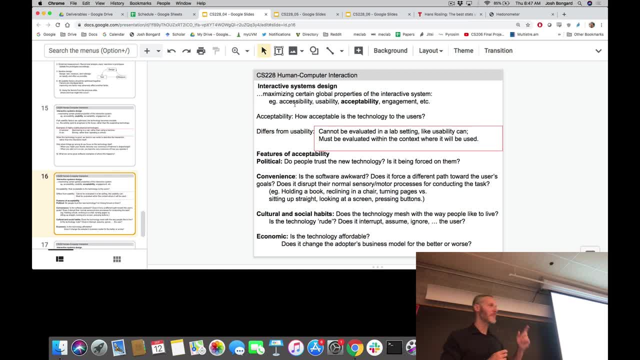 are some other examples besides ebooks, where acceptability is particularly challenging: cameras, okay, how so? i mean, as soon as you digitize, the method and it's easily portable, yep, okay. so the the fear, the fact that suddenly it's so easy, right, okay, okay, photography is a good one. 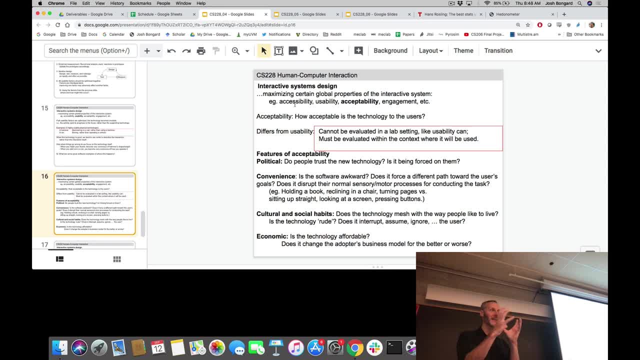 right. if you're a fan of photography, there's something about the physical act of the camera itself, like reading a book that's lost. when you suddenly have this book and you're like, oh my god, it's black rectangle and all you have to do is press the button and it does all the rest it makes. 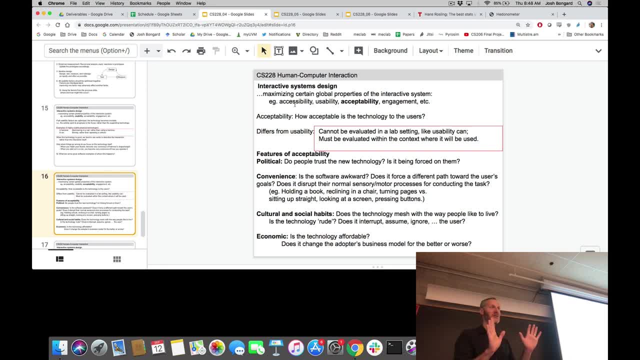 things easier to take a good photo again, depending on your definition of good, but that the very ease itself actually militates against acceptability for a lot of fans of photography. yes, okay, okay, that's a great example, right, right. the acceptability of touchscreens? okay, there's a great example. yeah, absolutely. 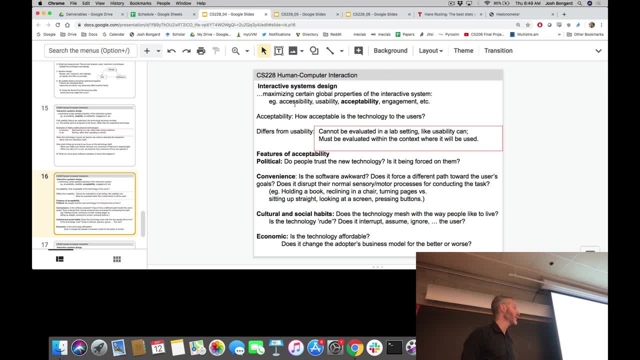 the act of driving. it would be interesting to see what happens when, when there's large-scale uptake of autonomous driving. that's a great example. an interesting recent example of this is a particular type of technology in which the better it becomes, the less acceptable it's becoming could be. maybe there's many examples. 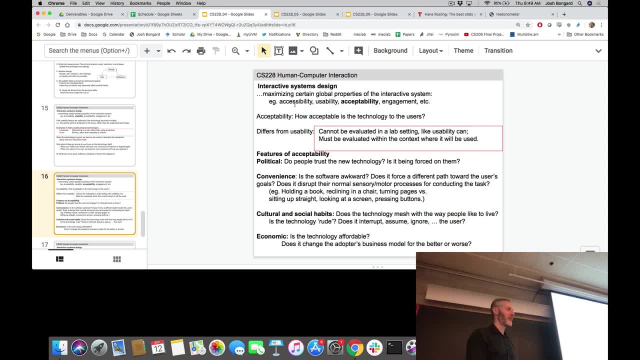 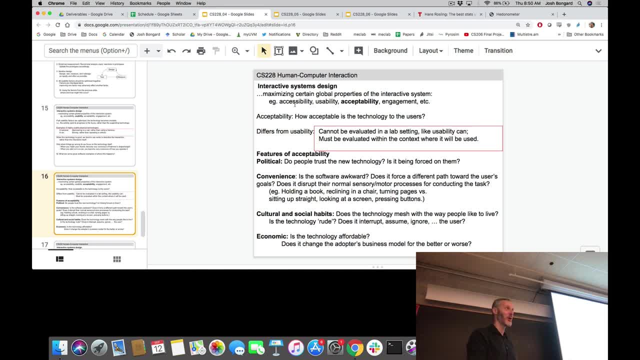 networks right, which are now addictive. networks right, which are now addictive- we've discovered right. the better they we've discovered right. the better they we've discovered right, the better they are. the longer Facebook holds you on are, the longer Facebook holds you on are. the longer Facebook holds you on Facebook, the less acceptable it is to the 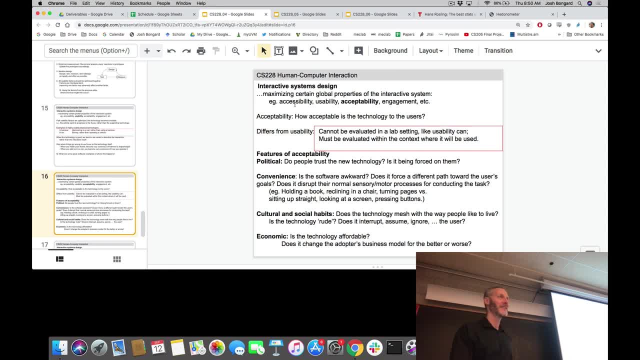 Facebook. the less acceptable it is to the Facebook, the less acceptable it is to the general public. right, we're all still general public right, we're all still general public, right, we're all still using it. but somehow we're it's not okay using it, but somehow we're it's not okay. 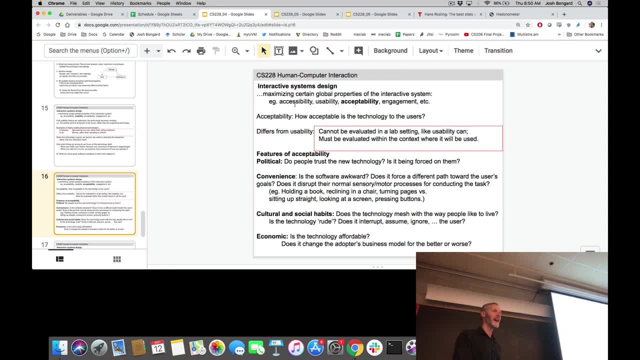 using it, but somehow we're: it's not okay anymore. right, it's same thing with AI anymore. right, it's same thing with AI anymore. right, it's same thing with AI. that the scary fact about how easy it's. that the scary fact about how easy it's. 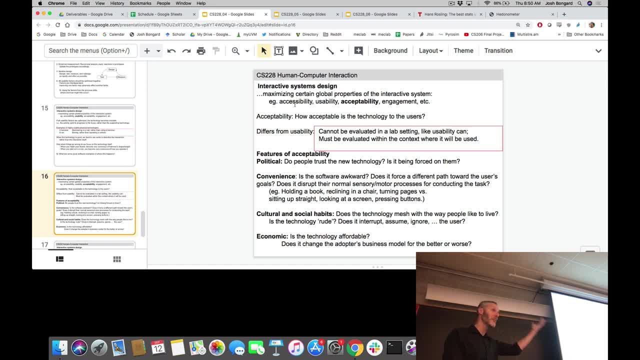 that the scary fact about how easy it's getting to use it to code it up, to getting to use it to code it up, to getting to use it to code it up to deploy it for a government to deploy it, deploy it for a government to deploy it. 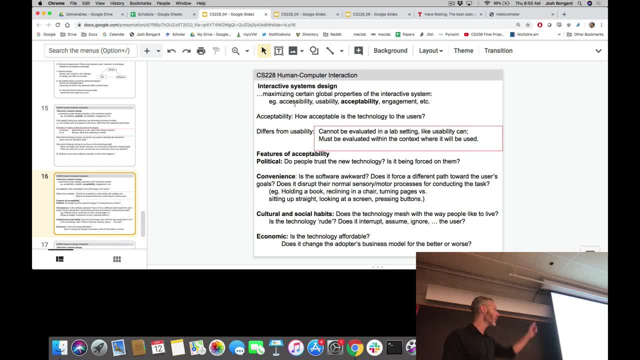 deploy it, for a government to deploy it, making the technology less acceptable. making the technology less acceptable. making the technology less acceptable. the more usable it becomes in that, the more usable it becomes in that, the more usable it becomes in that class of technologies, the less acceptable. class of technologies, the less acceptable. 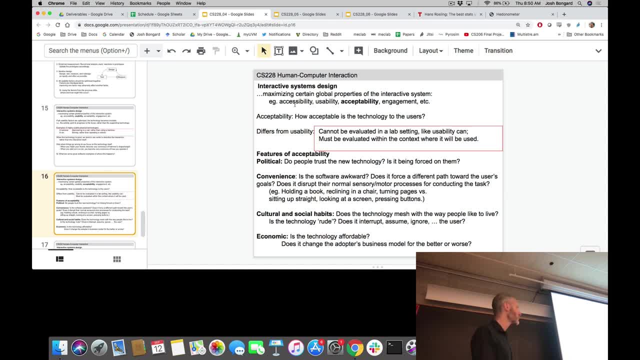 class of technologies, the less acceptable. that might not continue forever, but you, that might not continue forever. but you, that might not continue forever, but you can see these interesting social, can see these interesting social, can see these interesting social responses to large-scale technology. responses to large-scale technology. 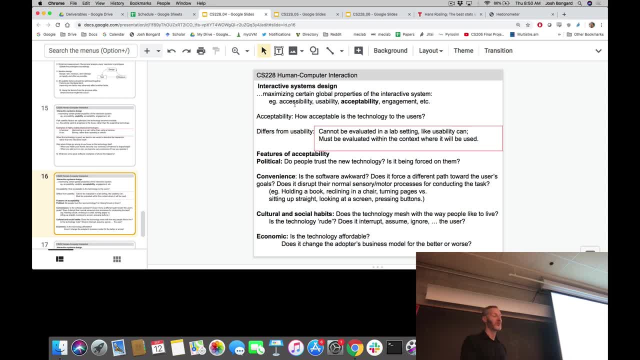 responses to large-scale technology. these have nothing really to do with the. these have nothing really to do with the. these have nothing really to do with the technology itself. maybe with the technology itself. maybe with the technology itself, maybe with the exception of AI. there are some exception of AI. there are some. 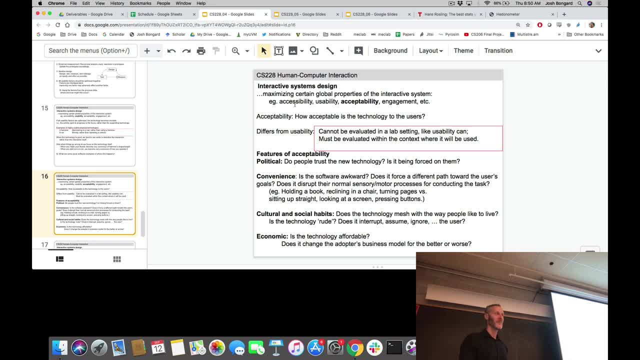 exception of AI. there are some technical challenges that needed to be technical challenges that needed to be technical challenges that needed to be worked out to get it to work. but it worked out to get it to work, but it worked out to get it to work. but it works. it's good, there's nothing wrong. 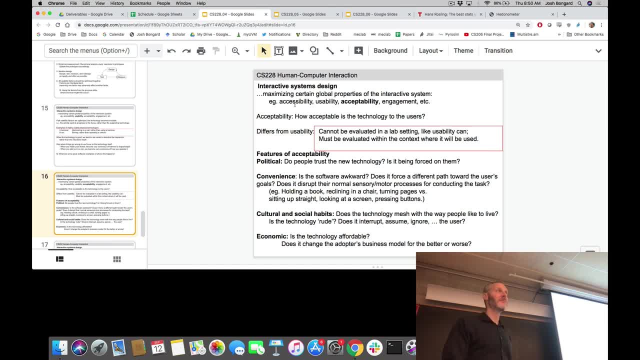 works, it's good. there's nothing wrong. works, it's good. there's nothing wrong with the functional requirements. right with the functional requirements. right with the functional requirements. right, it's something else. that's where the HCI it's something else. that's where the HCI it's something else. that's where the HCI aspect of this comes into play. okay. 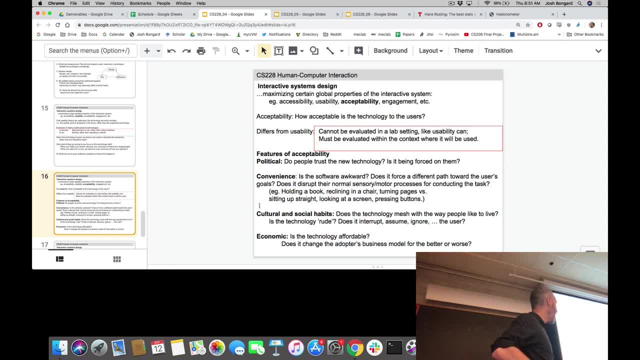 aspect of this comes into play. okay, aspect of this comes into play. okay, let's carry on. you'll notice a common. let's carry on. you'll notice a common. let's carry on. you'll notice a common pattern throughout this course, some of pattern throughout this course. some of 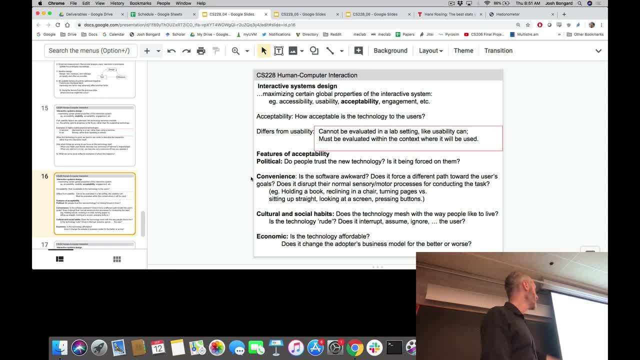 pattern throughout this course. some of these features of acceptability are kind. these features of acceptability are kind. these features of acceptability are kind of obvious right. PeopleSoft is being of obvious right. PeopleSoft is being of obvious right. PeopleSoft is being forced on faculty and staff at UVM. so 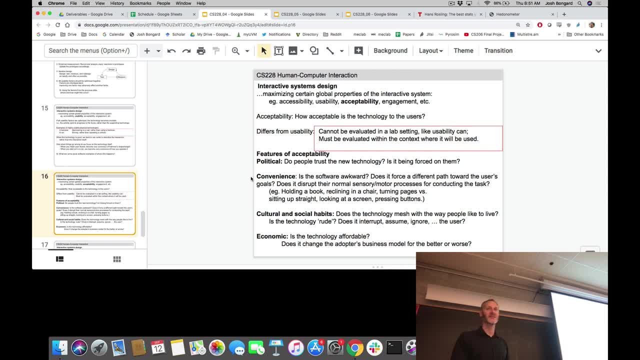 forced on faculty and staff at UVM. so forced on faculty and staff at UVM. so anyone could guess if they thought about. anyone could guess if they thought about. anyone could guess if they thought about it. there's going to be pushback to the it. there's going to be pushback to the. 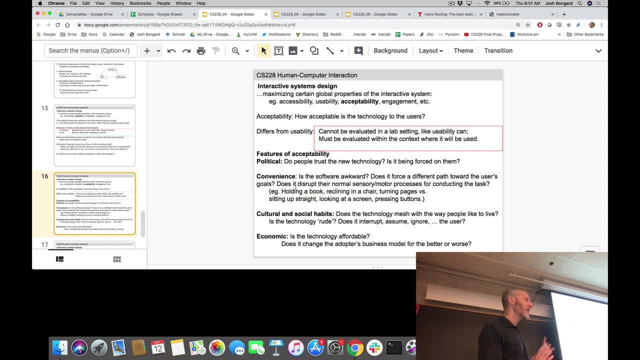 it. there's going to be pushback to the system, that one's kind of obvious system, that one's kind of obvious system, that one's kind of obvious convenience. you know the convenience of convenience. you know the convenience of convenience, you know the convenience of reading a book. there are some things. 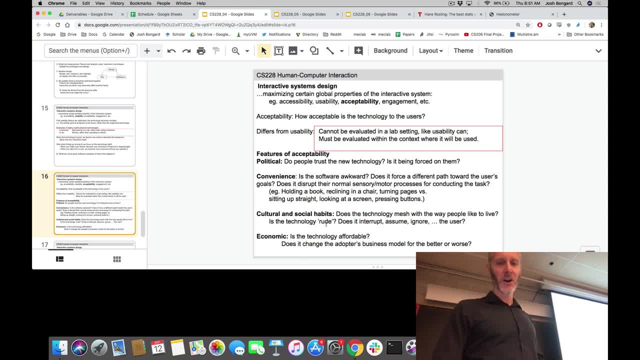 reading a book. there are some things reading a book. there are some things there that are obvious and not so there that are obvious and not so there that are obvious and not so obvious. cultural and social habits come obvious. cultural and social habits come obvious. cultural and social habits come into play here. is it affordable? is it? 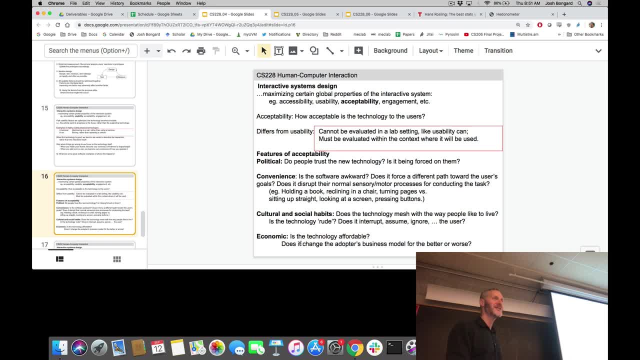 into play here? is it affordable? is it into play here? is it affordable? is it affordable to whom? the fact that affordable to whom? the fact that affordable to whom? the fact that sometimes the technology is cheaper, sometimes the technology is cheaper, sometimes the technology is cheaper easier is actually worse, works against. 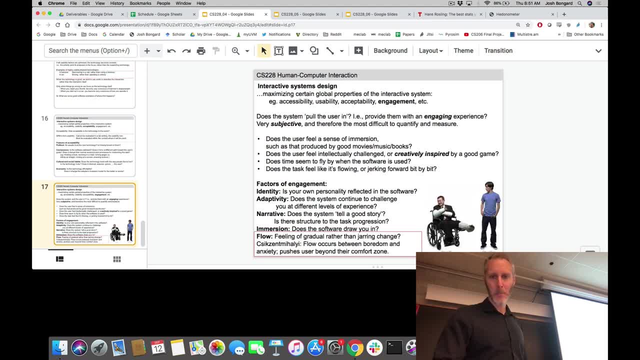 easier is actually worse, works against. easier is actually worse, works against acceptability. okay, let's move on to the acceptability. okay, let's move on to the acceptability. okay, let's move on to the most subjective aspect of these, most subjective aspect of these, most subjective aspect of these non-functional requirements, which is: 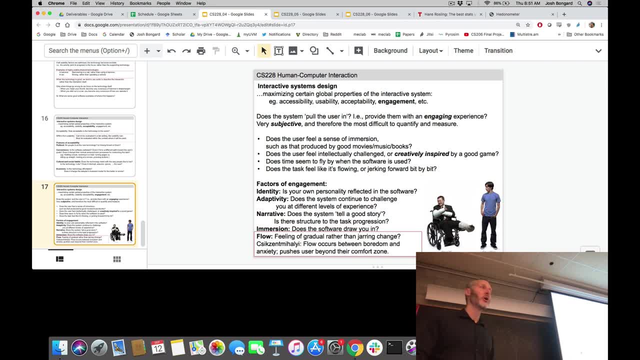 non-functional requirements. which is non-functional requirements, which is engagement. this is the most objective in engagement. this is the most subjective in engagement. this is the most subjective in the sense of we're trying to measure the sense of. we're trying to measure the sense of. we're trying to measure how much the technology pulls the user. 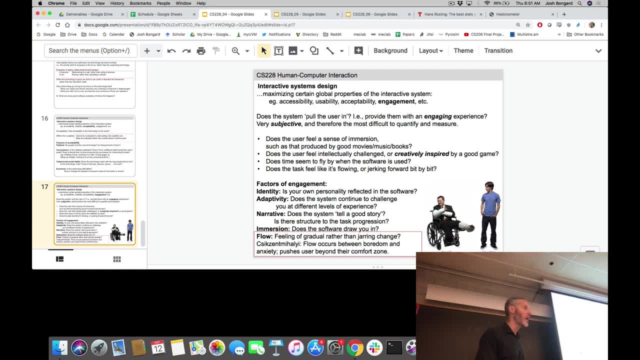 how much the technology pulls the user. how much the technology pulls the user in, this is sort of the primary in. this is sort of the primary in. this is sort of the primary non-functional requirement for most non-functional requirement for most non-functional requirement for most computer games, as you could imagine very 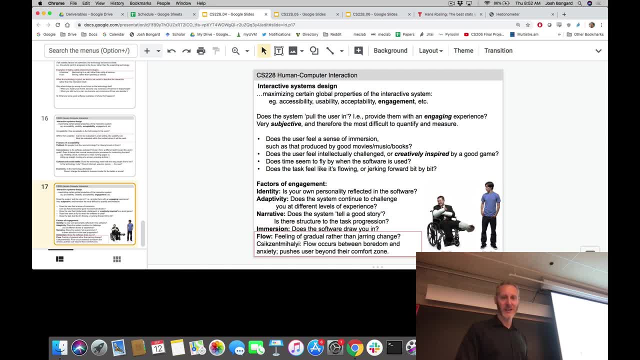 computer games, as you could imagine, very computer games, as you could imagine very hard to nail this one down and measure hard to nail this one down and measure hard to nail this one down and measure it objectively, what we're trying to, it objectively, what we're trying to. 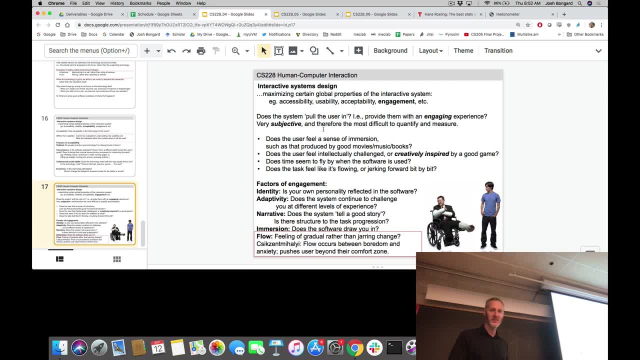 it objectively, what we're trying to figure out is: does it pull the user in? figure out is: does it pull the user in? figure out is: does it pull the user in? does it create a positive subjective? does it create a positive subjective? does it create a positive subjective experience for them? do they feel a sense? 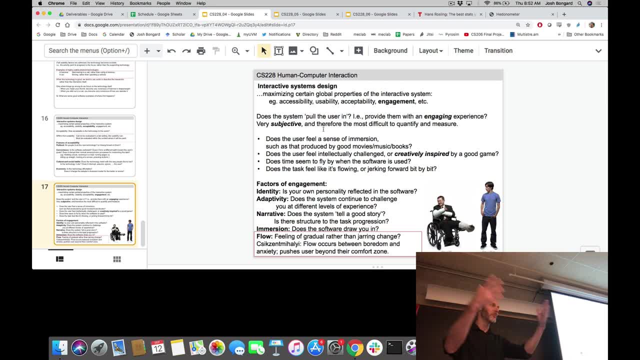 experience for them? do they feel a sense experience for them? do they feel a sense of immersion? do they fall into the game of immersion? do they fall into the game of immersion? do they fall into the game or the software, whatever it is that, or the software, whatever it is that? 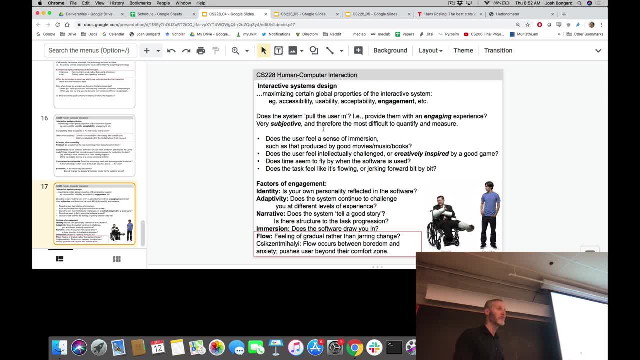 or the software, whatever it is- that we're trying to build for them in the. we're trying to build for them in the. we're trying to build for them in the same way that people talk about good, same way that people talk about good, same way that people talk about good movies and good books. right, I got lost. 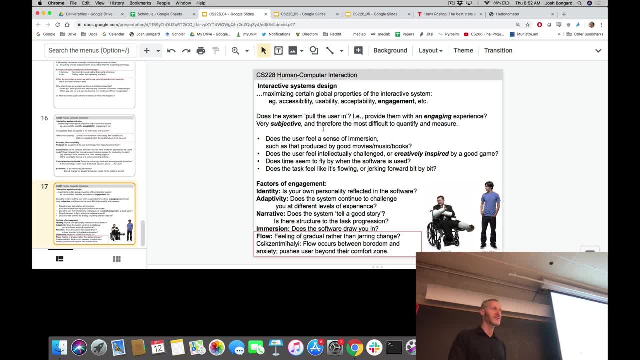 movies and good books- right, I got lost. movies and good books, right, I got lost in a good book. that kind of language in a good book, that kind of language in a good book, that kind of language again gives you a hint about whether, again gives you a hint about whether. 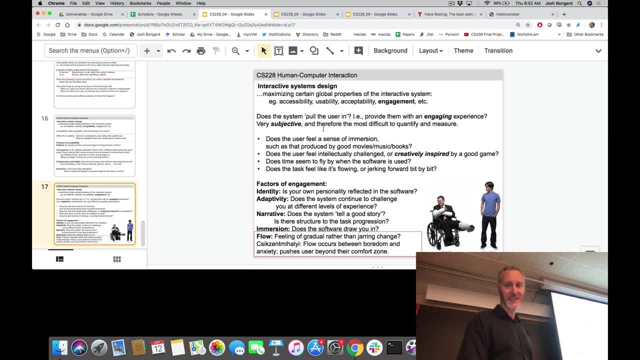 again gives you a hint about whether the system or the book or the software, the system or the book or the software, the system or the book or the software is engaging, are they challenged or is engaging? are they challenged or is engaging? are they challenged or creatively inspired? for a lot of 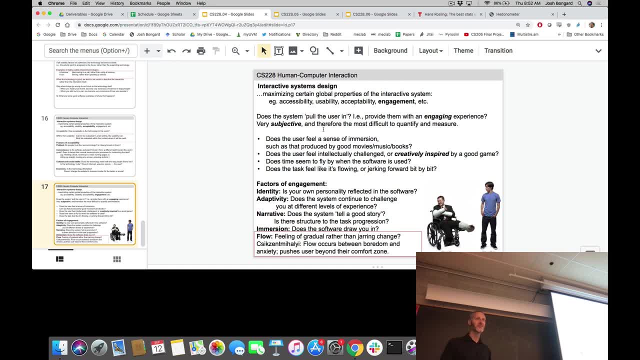 creatively inspired for a lot of creatively inspired, for a lot of technology. we want the user to think as technology. we want the user to think as technology. we want the user to think as little as possible. we want the system to little as possible. we want the system to. 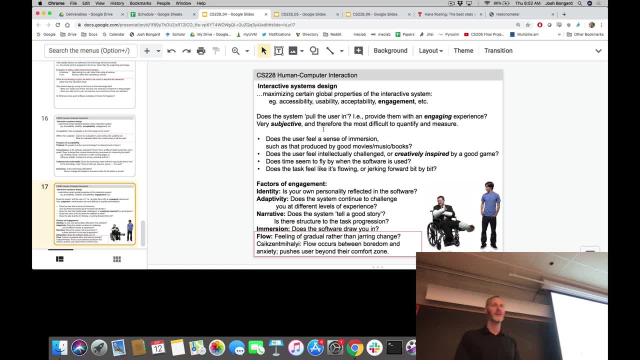 little as possible. we want the system to be as easy for them to use. we don't want be as easy for them to use. we don't want be as easy for them to use. we don't want them to think or feel challenged, but in them. to think or feel challenged, but in. 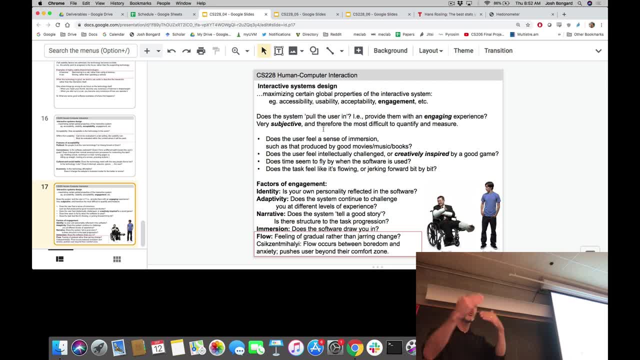 them to think or feel challenged. but in some cases- like games or educational, some cases like games or educational, some cases like games or educational software, we want to bring them to the software, we want to bring them to the software, we want to bring them to the edge of expertise. right, we want it. we. 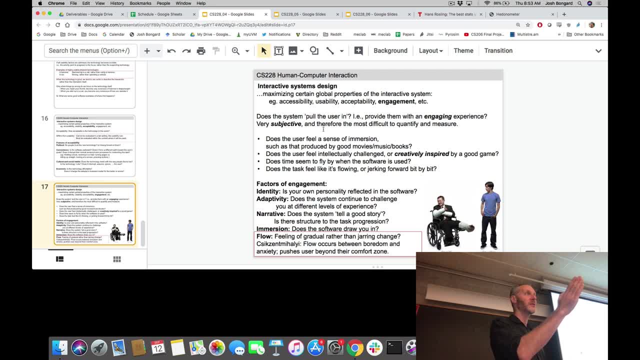 edge of expertise: right, we want it. we edge of expertise: right, we want it. we want to try and detect and bring them to want to try and detect and bring them to want to try and detect and bring them to that sweet spot between frustration and that sweet spot between frustration and. 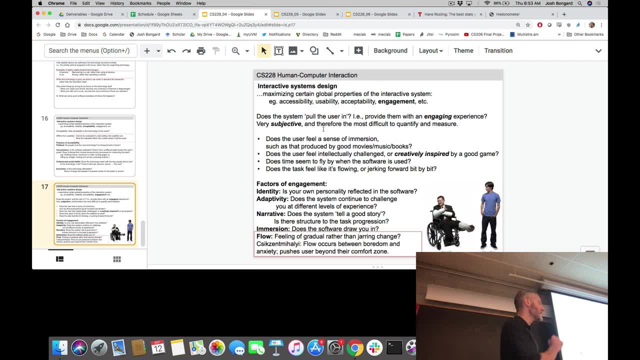 that sweet spot between frustration and boredom difficult to get right. because boredom difficult to get right, because boredom difficult to get right, because you need a system that can somehow. you need a system that can somehow, you need a system that can somehow measure boredom and frustration and tune. 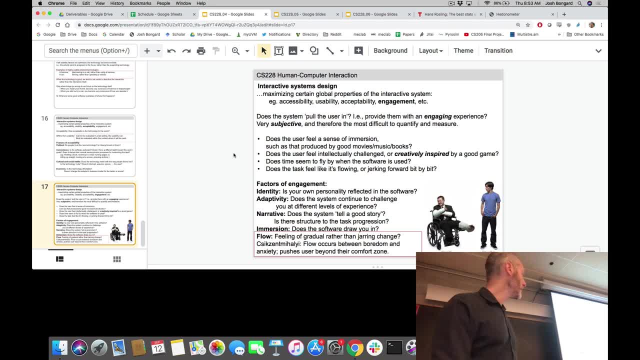 measure boredom and frustration and tune. measure boredom and frustration and tune itself accordingly. does the user talk itself accordingly? does the user talk itself accordingly? does the user talk about time flying by when they use the about time flying by when they use the about time flying by when they use the system, or does it feel like things are? 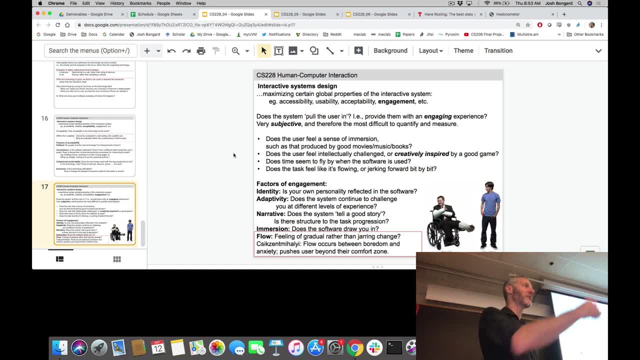 system, or does it feel like things are system? or does it feel like things are flowing from one to the next? or are they flowing from one to the next? or are they flowing from one to the next, or are they being jerked from one level of the game? 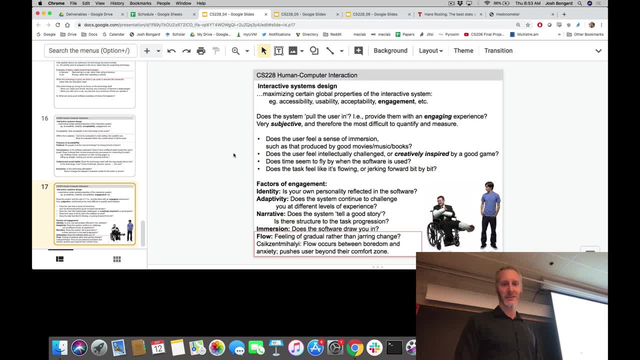 being jerked from one level of the game. being jerked from one level of the game or one level of the educational, or one level of the educational or one level of the educational software from one level to the next? how? software from one level to the next? how? 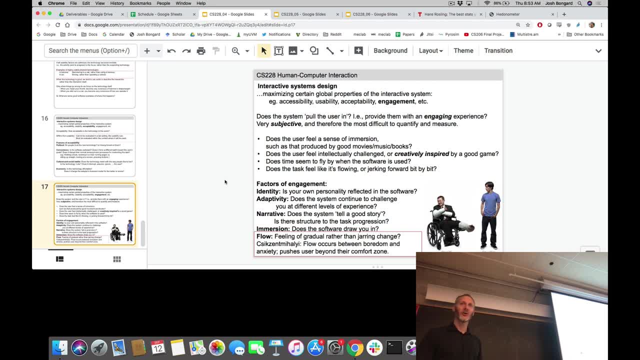 software from one level to the next. how do we go about trying to increase? do we go about trying to increase? do we go about trying to increase engagement again a difficult thing to do. engagement again a difficult thing to do. engagement again a difficult thing to do because we're in a very subjective area. 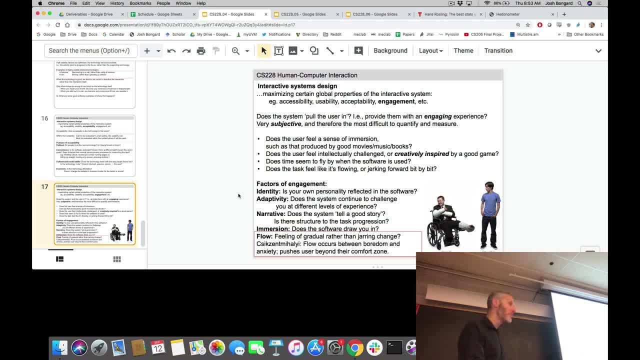 because we're in a very subjective area, because we're in a very subjective area now, but if you look at the history of now, but if you look at the history of now, but if you look at the history of design, Apple is sort of a master at this. 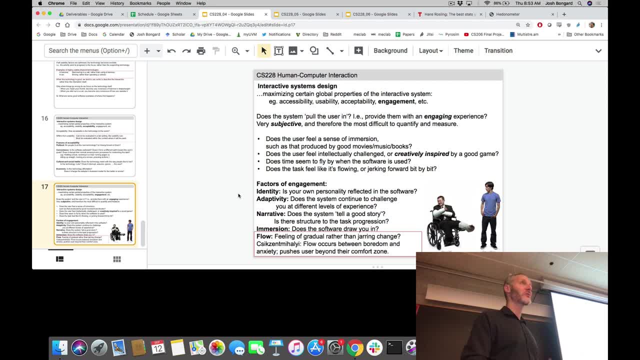 design. Apple is sort of a master at this design. Apple is sort of a master at this. there's sort of certain design. there's sort of certain design. there's sort of certain design, principles or rules of thumbs that come, principles or rules of thumbs that come, principles or rules of thumbs that come into play, things that are engaging seem. 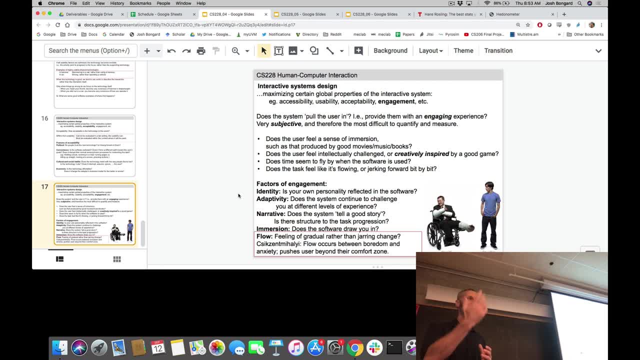 into play things that are engaging, seem into play things that are engaging seem to fit quote-unquote with the user, to fit quote-unquote with the user, to fit quote-unquote with the user. somehow they see their identity, somehow they see their identity, somehow they see their identity reflected, their identity or their. 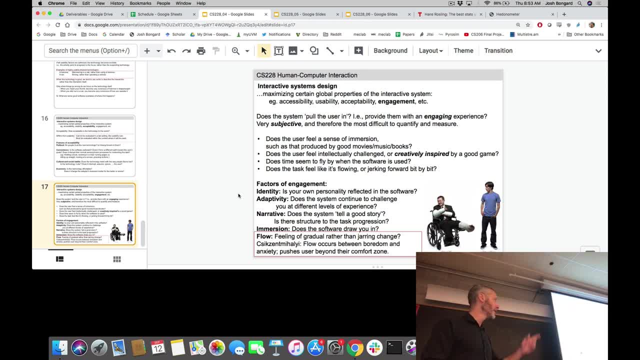 reflected their identity or their. reflected their identity or their philosophy reflected in the technology philosophy. reflected in the technology philosophy reflected in the technology. Apple exploited this to great effect in Apple exploited this to great effect in. Apple exploited this to great effect in their series of TV commercials about I'm. 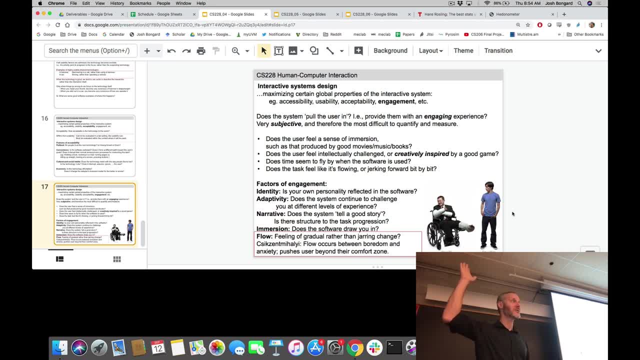 their series of TV commercials about I'm, their series of TV commercials about I'm a PC and I'm a Mac. do people still a PC and I'm a Mac? do people still a PC and I'm a Mac? do people still remember these commercials or am I? 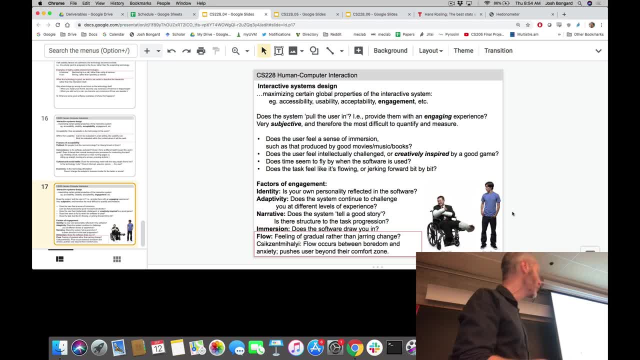 remember these commercials? or am I remember these commercials or am I dating myself here? okay, if you've never dating myself here, okay, if you've never dating myself here, okay, if you've never seen them, go go YouTube. I'm a PC, I'm a. seen them go go YouTube. I'm a PC, I'm a. 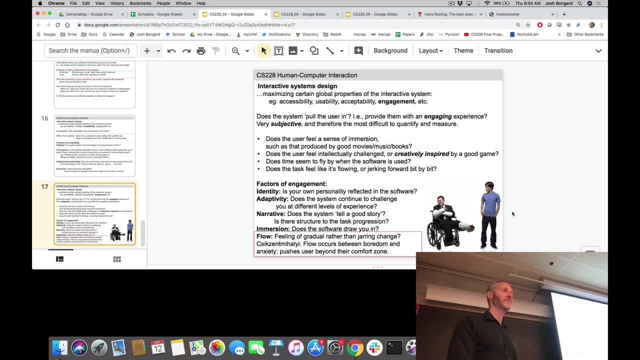 seen them go go YouTube. I'm a PC, I'm a Mac. which of these two people would you Mac? which of these two people would you Mac? which of these two people would you rather be okay, all right, so I already. rather be okay, all right, so I already. 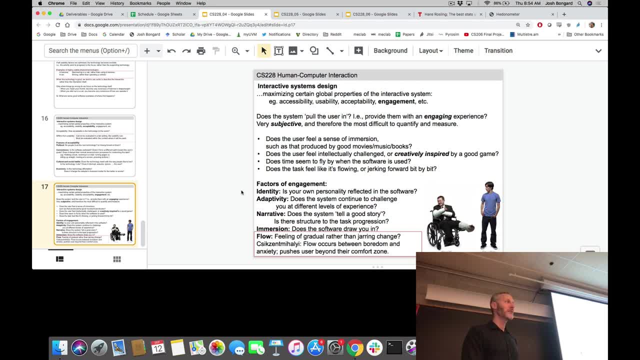 rather be okay, all right. so I already mentioned adaptivity. so if we are trying mentioned adaptivity, so if we are trying mentioned adaptivity, so if we are trying to creatively challenge the user, we need to creatively challenge the user, we need to creatively challenge the user, we need to add this additional level of 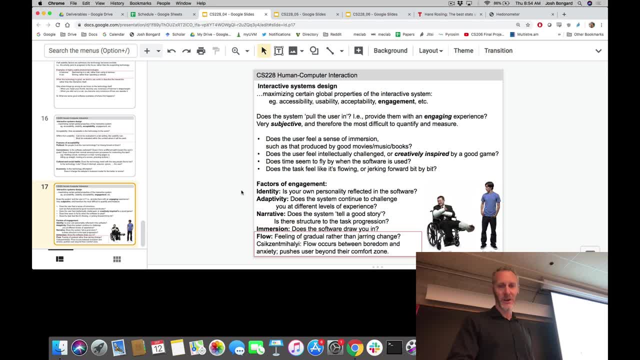 to add this additional level of, to add this additional level of adaptivity, which becomes extremely adaptivity, which becomes extremely adaptivity, which becomes extremely difficult to get right. is there a difficult to get right? is there a difficult to get right? is there a narrative to your system? if it's a, 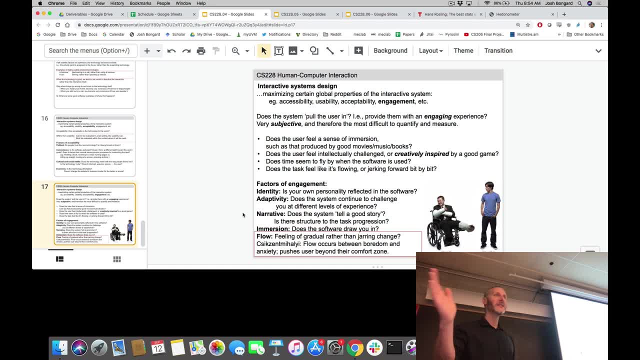 narrative to your system. if it's a narrative to your system, if it's a computer game, that might be relatively computer game, that might be relatively computer game, that might be relatively straightforward to get right. you're straightforward to get right. you're straightforward to get right. you're leading the user through a series of 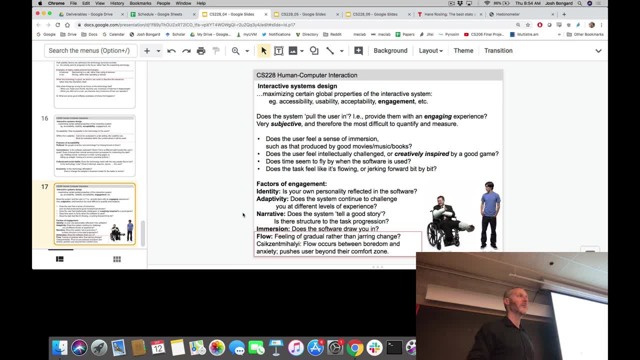 leading the user through a series of leading the user through a series of levels. but is there? is there a narrative levels? but is there? is there a narrative levels? but is there? is there a narrative arc? there may be sort of a relatively arc. there may be sort of a relatively. 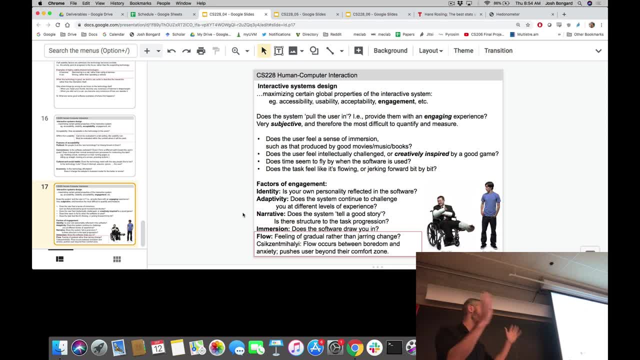 arc. there may be sort of a relatively nebulous, unspecified sort of experience. nebulous, unspecified sort of experience. nebulous, unspecified sort of experience. it may be a sandbox game or an open. it may be a sandbox game or an open. it may be a sandbox game or an open world or a wiki where people can create. 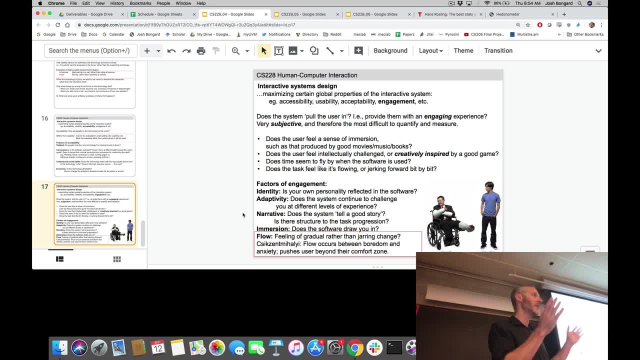 world or a wiki where people can create world or a wiki where people can create things on their own. there is no real by things on their own. there is no real by things on their own. there is no real by definition: start, middle and an end for a. 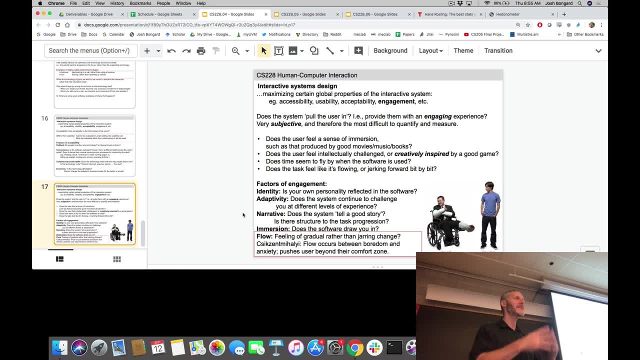 definition: start, middle and an end for a definition: start, middle and an end for a lot of people. that becomes disorienting, lot of people. that becomes disorienting lot of people. that becomes disorienting and frustrating- i can't tell if i made- and frustrating- i can't tell if i made. 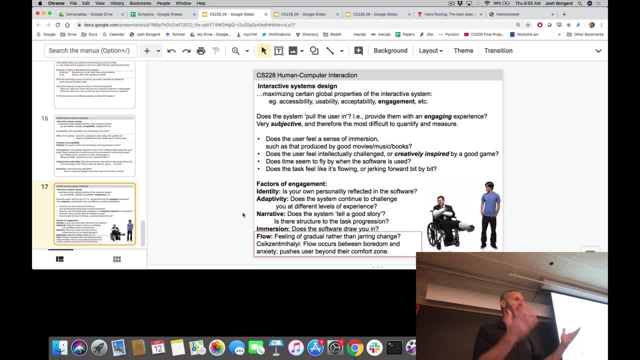 and frustrating. i can't tell if i made progress with this system. i spent two progress with this system. i spent two progress with this system. i spent two hours with it and i don't know if i'm hours with it and i don't know if i'm. 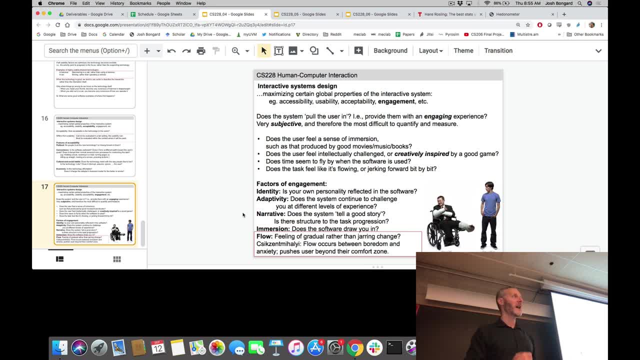 hours with it and i don't know if i'm any further than i was when i started, any further than i was when i started, any further than i was when i started? how do we help paint that picture for? how do we help paint that picture for? 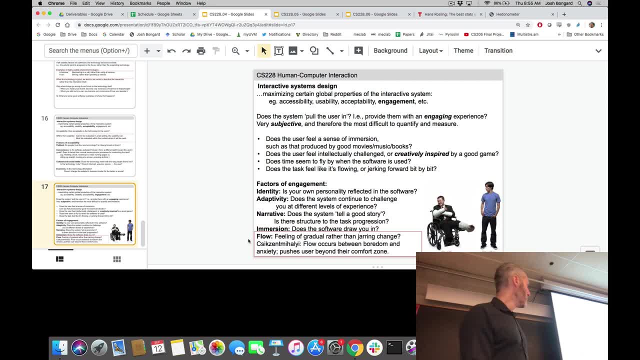 how do we help paint that picture for our users? difficult thing our users. difficult thing our users. difficult thing to do: immersion. so people talk about to do immersion. so people talk about to do immersion. so people talk about being drawn into a good book or a good, being drawn into a good book or a good. 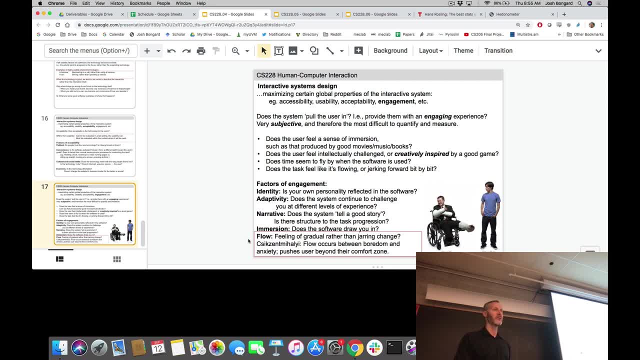 being drawn into a good book or a good movie. how does software and hardware go movie? how does software and hardware go movie? how does software and hardware go about drawing the user in? about drawing the user in, about drawing the user in. users will often describe engaging. users will often describe engaging. 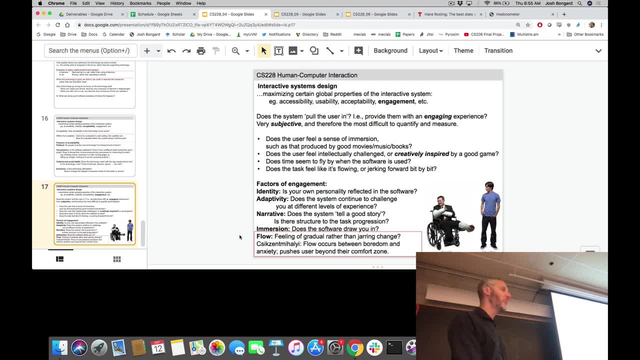 users will often describe engaging experiences as again it seemed like time experiences, as again it seemed like time experiences, as again it seemed like time, flew by flew by flew by. i was, i seemed to effortlessly be able. i was, i seemed to effortlessly be able. i was, i seemed to effortlessly be able to do a, b and c. 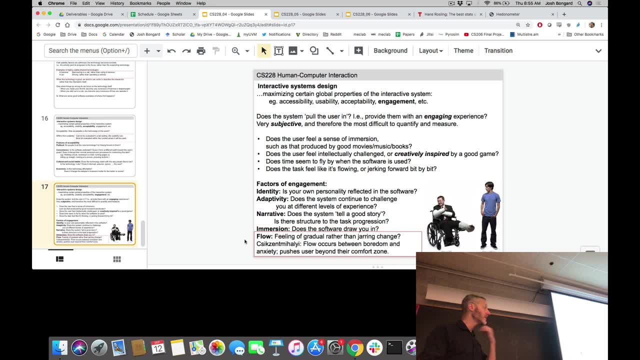 to do a, b and c. to do a, b and c. this is sort of a subjective experience. this is sort of a subjective experience. this is sort of a subjective experience that the psychologist chick said metalli. that the psychologist chick said metalli. that the psychologist chick said metalli spent quite a bit of time talking about. 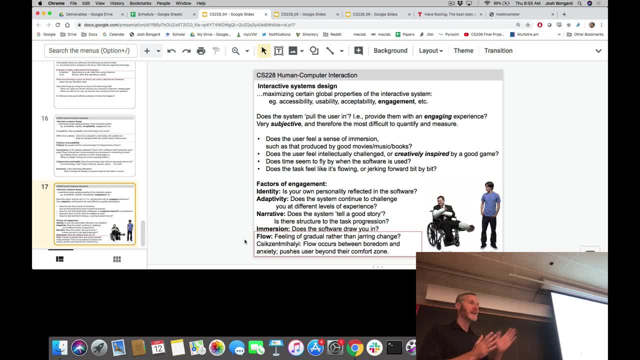 spent quite a bit of time talking about. spent quite a bit of time talking about: wrote a very famous book called flow. wrote a very famous book called flow. wrote a very famous book called flow. look, he looked at athletes and other. look, he looked at athletes and other. 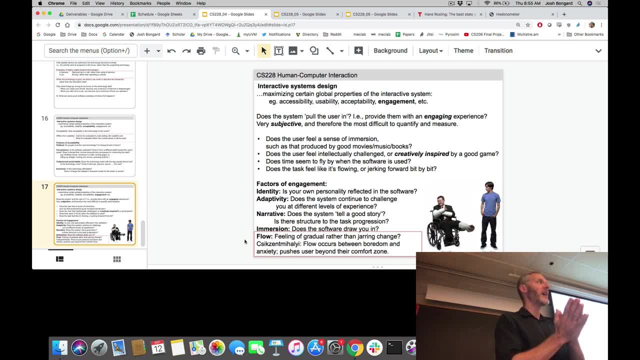 look. he looked at athletes and other performance performers at the peak of performance, performers at the peak of performance. performers at the peak of their ability in different areas and their ability in different areas and their ability in different areas, and asked them to describe when you played. asked them to describe when you played. 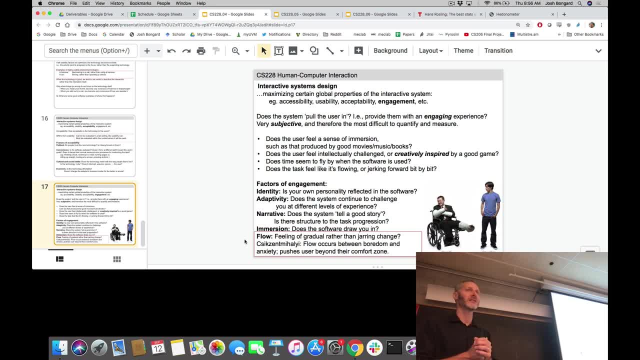 asked them to describe when you played your best game of tennis. what was it your best game of tennis? what was it your best game of tennis? what was it like? what happened during that? like what happened during that. like what happened during that experience and across very different. 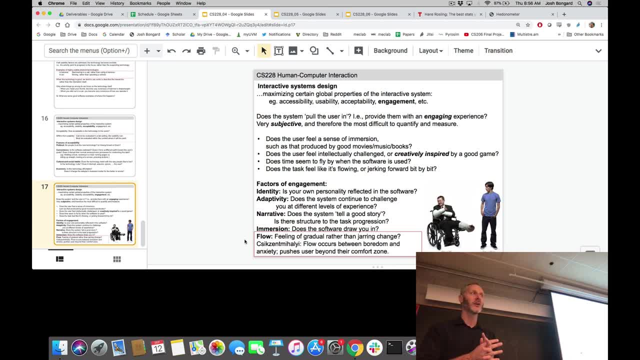 experience, and across very different experience and across very different domains. he realized he was getting back domains. he realized he was getting back domains. he realized he was getting back very similar stories from these top, very similar stories from these top, very similar stories from these top performers. time seemed to slow down. 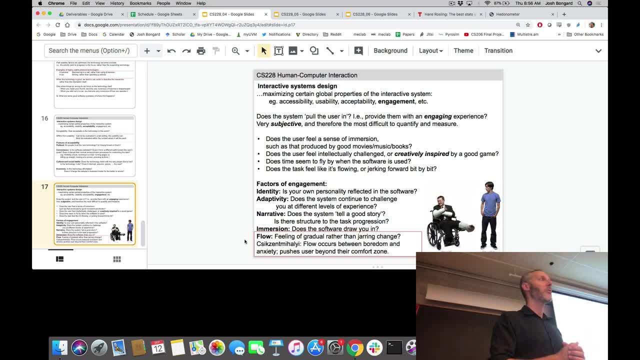 performers, time seemed to slow down. performers, time seemed to slow down. i- i had plenty of time to wind up and i, i had plenty of time to wind up and i, i had plenty of time to wind up and hit the ball exactly where i wanted. hit the ball exactly where i wanted. 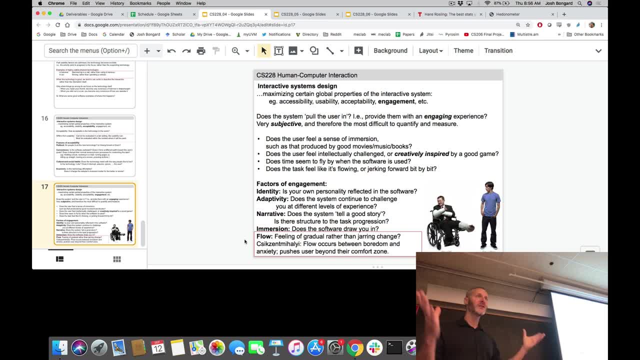 hit the ball exactly where i wanted. it took no effort at all. how do we go? it took no effort at all. how do we go? it took no effort at all. how do we go about creating a system where users about creating a system where users about creating a system where users have that experience in the system again. 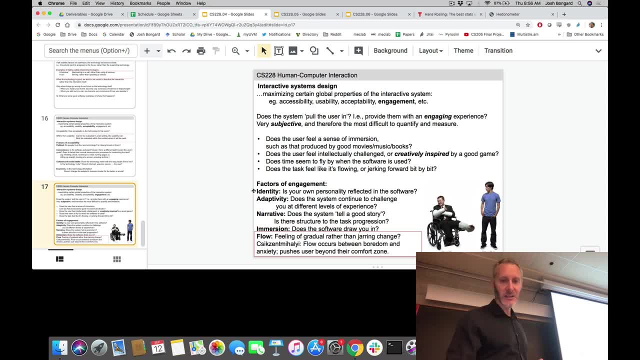 have that experience in the system again. have that experience in the system again difficult to say is a very subjective, difficult to say is a very subjective, difficult to say is a very subjective area. but let's look at these one two area. but let's look at these one two. 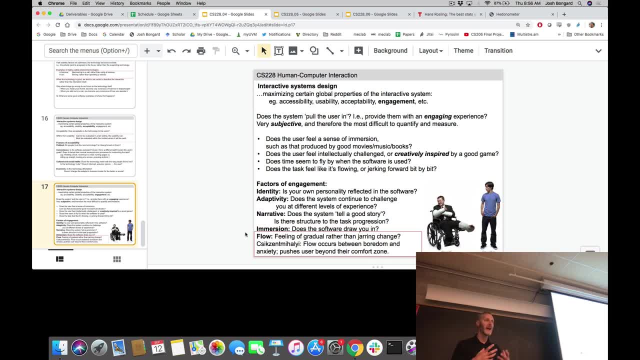 area. but let's look at these one, two, three, four, five uh design principles- three, four, five uh design principles. three, four, five uh design principles that we might try and maximize in our, that we might try and maximize in our, that we might try and maximize in our system, in our system, to create an 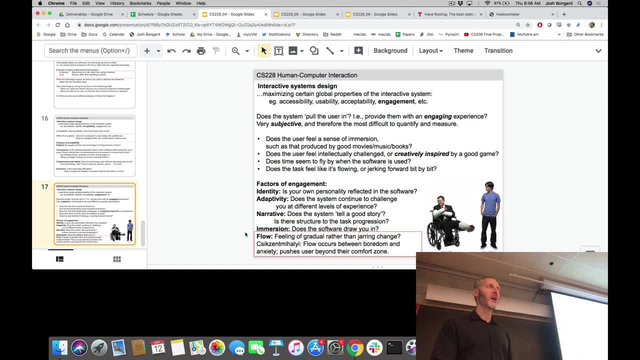 system in our system to create an system in our system to create an engaging experience. engaging experience, engaging experience. what are some examples of software and what are some examples of software and what are some examples of software and hardware that try to do this, hardware that try to do this? 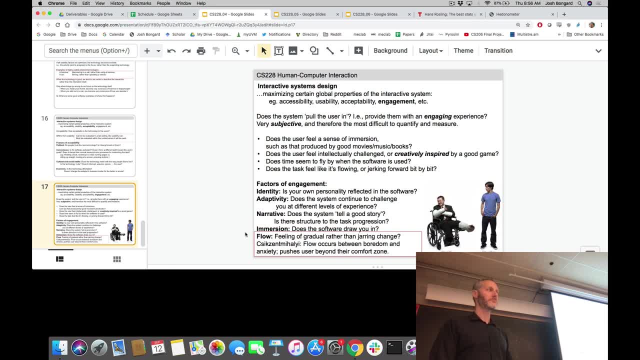 hardware that try to do this explicitly: uh, that website, uh, that website. uh, that website usually can graduate. uh, congratulate you, usually can graduate. uh, congratulate you, usually can graduate. uh, congratulate you when you are, when you are, when you are the first year, second year, okay, that's. 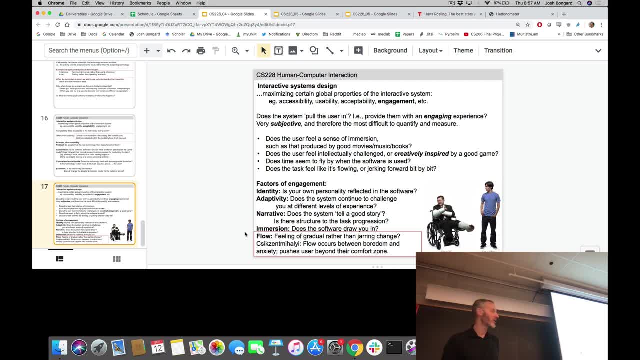 the first year, second year. okay, that's the first year, second year, okay, that's a progressive. exactly so: badges and a progressive, exactly so. badges and a progressive, exactly so: badges and points, points, points. so what, which of these five is that? so what, which of these five is that? 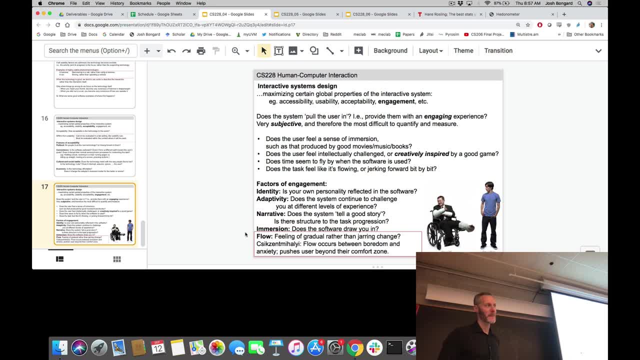 so what? which of these five is that addressing? it's an incentivization mechanism, right? it's an incentivization mechanism, right, it's an incentivization mechanism, right? you're incentivizing them to try to do. you're incentivizing them to try to do. you're incentivizing them to try to do something by giving them a badge. what is? 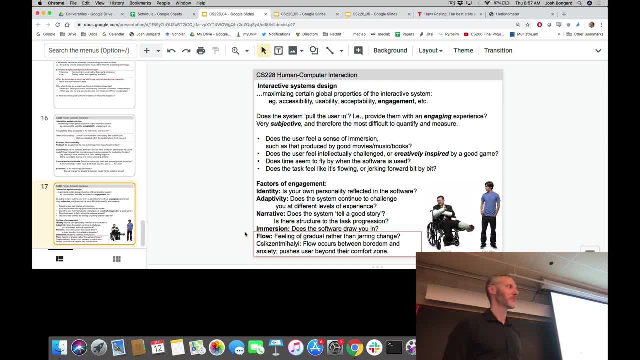 something by giving them a badge? what is something by giving them a badge? what is it? did you say that's identity like you're? did you say that's identity like you're? did you say that's identity like you're? if you're identifying that level of 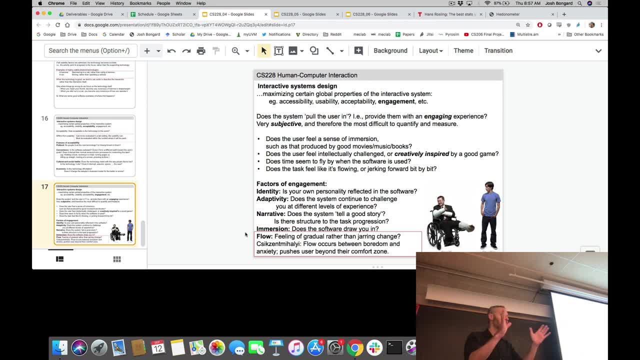 if you're identifying that level of, if you're identifying that level of engagement, engagement, engagement, possibly again we're in a subjective. possibly again we're in a subjective. possibly again we're in a subjective area. here there's no right or wrong area. here there's no right or wrong. 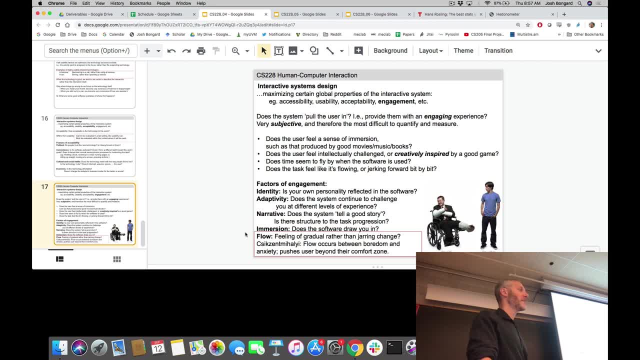 area. here there's no right or wrong answer. absolutely right. badges are kind of absolutely right. badges are kind of absolutely right. badges are kind of waypoints- right, you've made it this far. waypoints- right, you've made it this far. waypoints- right, you've made it this far. if you've ever used Duolingo, which is 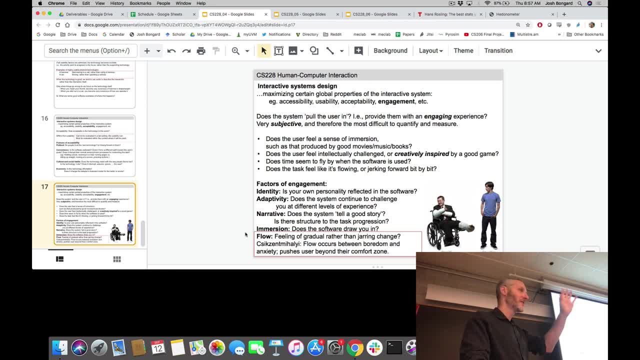 if you've ever used Duolingo, which is, if you've ever used Duolingo, which is the foreign language educational, the foreign language educational, the foreign language educational software. if you breathe, you get a badge software. if you breathe, you get a badge software. if you breathe, you get a badge right, but it's very important. 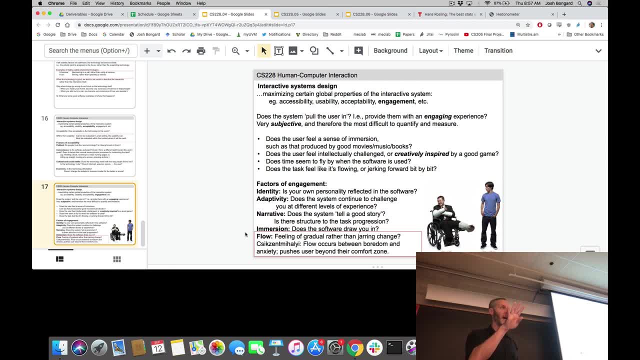 right, but it's very important, right, but it's very important, especially in an educational game, and especially in an educational game, and especially in an educational game, and this is going to be important for you in, this is going to be important for you in, this is going to be important for you in the last four weeks of this semester. 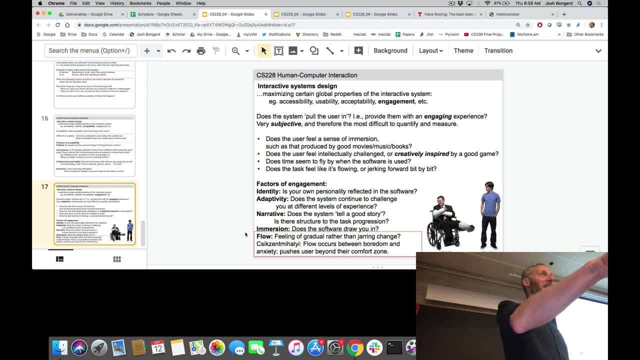 the last four weeks of this semester, the last four weeks of this semester. it's not a lot of fun to try and get. it's not a lot of fun to try and get. it's not a lot of fun to try and get your hand to hold exactly right to get. 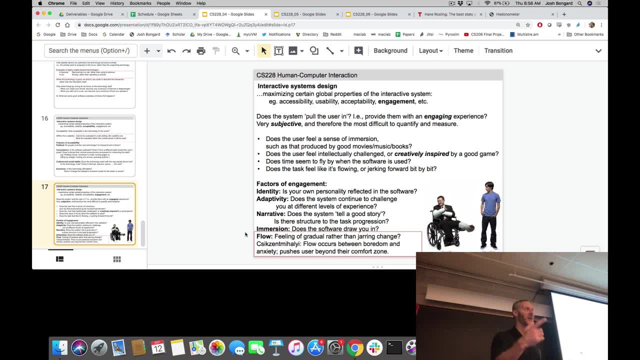 your hand to hold exactly right, to get your hand to hold exactly right to get the right gesture, let alone learn the the right gesture, let alone learn the the right gesture, let alone learn the gesture. remember the gesture. learning is gesture. remember the gesture. learning is gesture. remember the gesture. learning is not always a pleasurable experience. 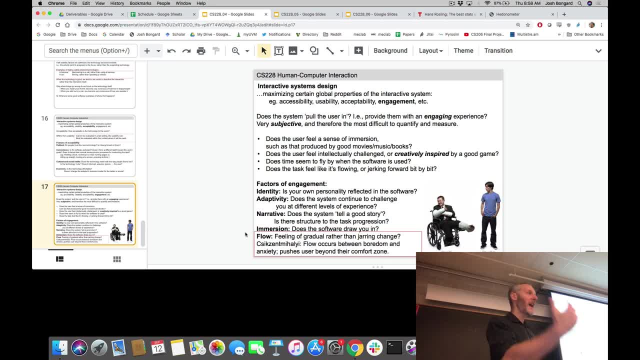 not always a pleasurable experience. not always a pleasurable experience, right, so can we help. can we help the right, so can we help. can we help the right, so can we help. can we help the user along right. we, we see you, we know. user along right, we, we see you, we know. 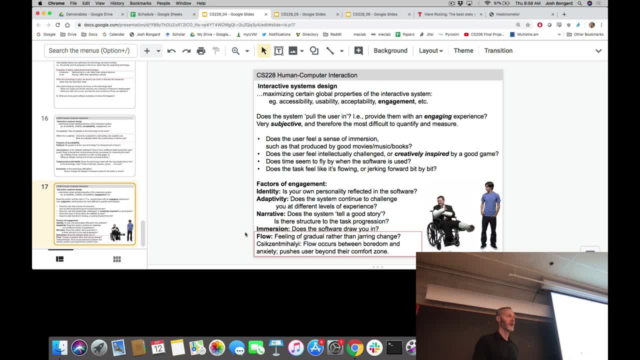 user along right. we, we see you. we know that you have put in a lot of effort, that you have put in a lot of effort. that you have put in a lot of effort. here's a gold star. you're now at level. here's a gold star. you're now at level. 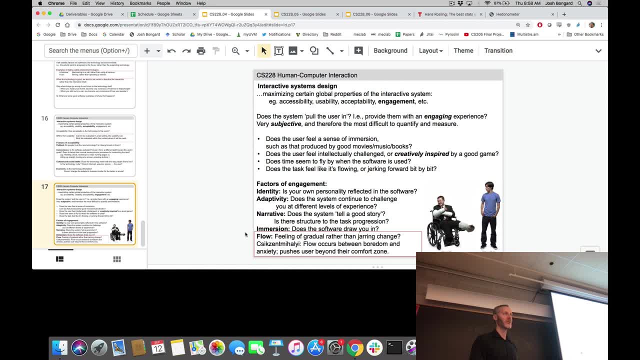 here's a gold star. you're now at level whatever that's a great example. other whatever that's a great example. other whatever that's a great example. other examples: absolutely so we'll talk a fair. absolutely so, we'll talk a fair. absolutely so we'll talk a fair bit about gamification. there needs to be a. 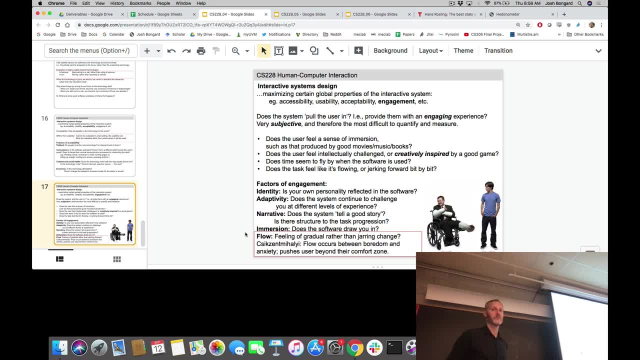 bit about gamification. there needs to be a bit about gamification. there needs to be a lot of out of adaptivity in there. lot of out of adaptivity in there, lot of out of adaptivity in there. um for the iphone, um for the iphone, um for the iphone. they deliberately, when you do the id. 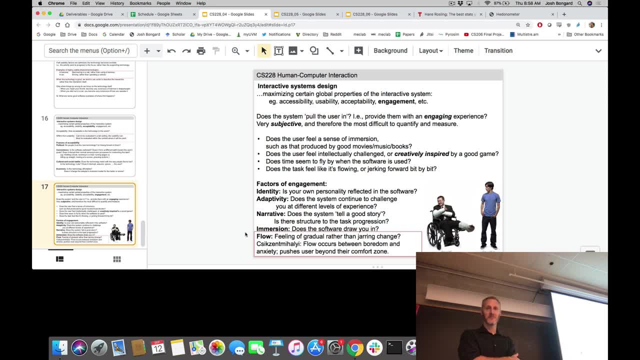 they deliberately when you do the id. they deliberately when you do the id. okay, okay, okay, okay. so it's not so. you're like um. so it's not so. you're like um. so it's not so. you're like um. playing to put your your thumbprints. 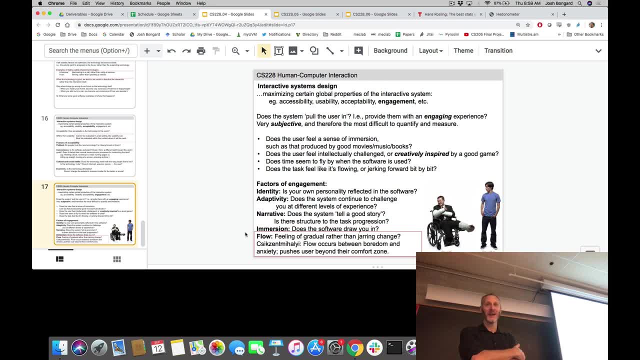 playing to put your, your thumbprints. playing to put your, your thumbprints, to get your id working. oh, i see that to get your id working. oh, i see that to get your id working. oh, i see that you got to match up your. yeah, exactly, you got to match up your. yeah, exactly. 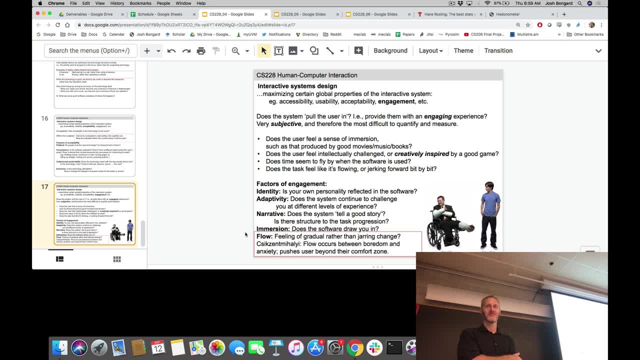 you got to match up your yeah, exactly like a childish kind of like. how would like a childish kind of like, how would like a childish kind of like, how would you um to make it fun? it's not just you, um to make it fun, it's not just. 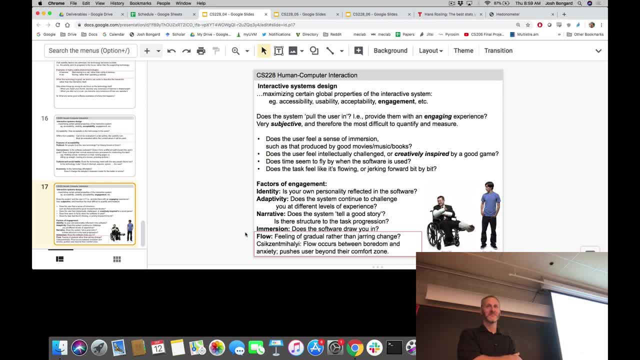 you, um, to make it fun. it's not just like, oh, like, oh, like, oh. it's like that. that's a great example gamifying. that that's a great example gamifying. that. that's a great example gamifying. just even recognizing a thumbprint. just even recognizing a thumbprint. 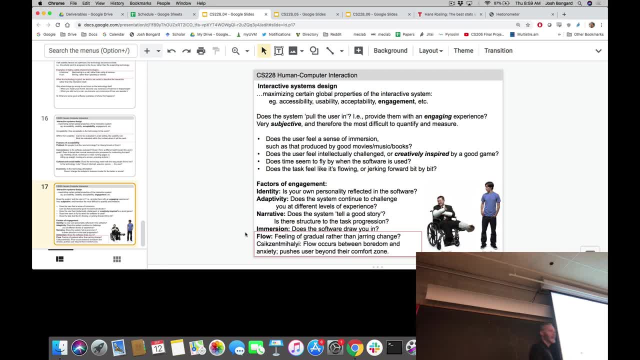 just even recognizing a thumbprint. what about immersion? this one is kind of. what about immersion? this one is kind of. what about immersion? this one is kind of interesting, right, interesting, right, interesting. right up until relatively recently- there was up until relatively recently, there was up until relatively recently- there was a screen and maybe a speaker where you 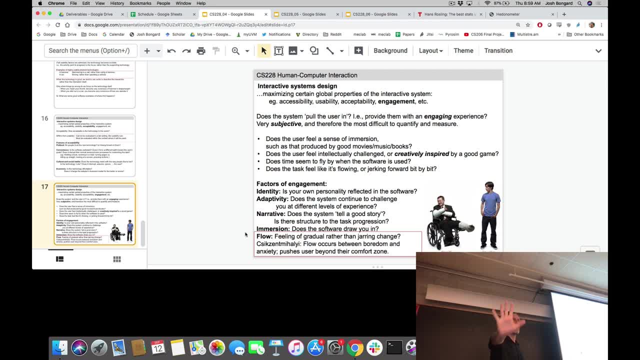 a screen and maybe a speaker where you a screen, and maybe a speaker where you could see and hear things, but the? the could see and hear things, but the? the could see and hear things, but the? the technology was over there, i'm not in. the technology was over there, i'm not in. 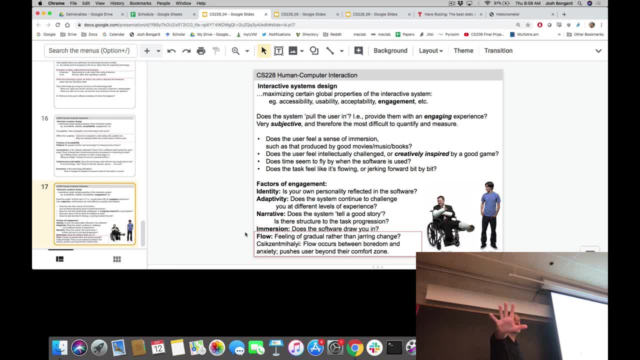 the technology was over there. i'm not in the game or in the system. same thing, the game or in the system. same thing the game or in the system. same thing, obviously, with a book and a movie. it's obviously with a book and a movie. it's. 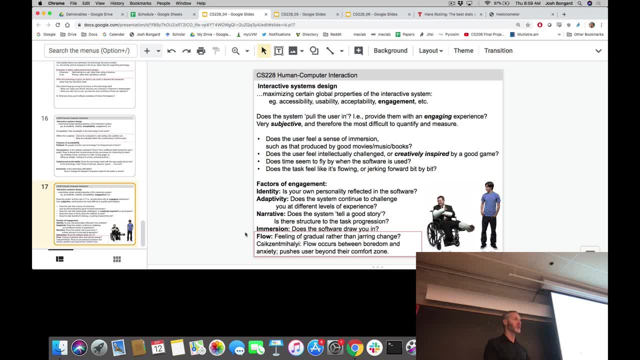 obviously, with a book and a movie, it's also distant from you, but also distant from you, but also distant from you. but if you've ever read a great book, or if you've ever read a great book, or if you've ever read a great book or watched a great movie, you feel like 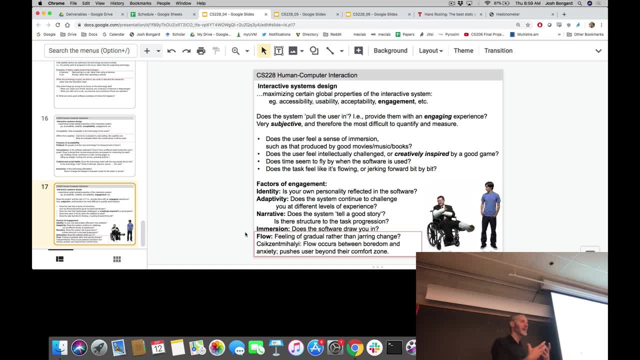 watched a great movie. you feel like watched a great movie. you feel like you're inside right. how do we you're inside right. how do we you're inside right? how do we? creating good engagement is often about creating. good engagement is often about creating good engagement is often about creating the illusion of 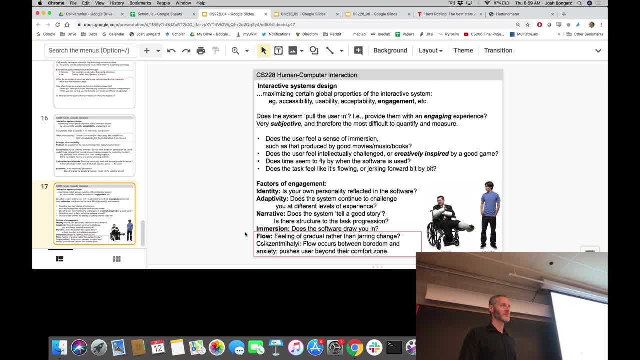 creating the illusion, of creating the illusion of so for the immersion. you can do like so for the immersion. you can do like so for the immersion. you can do like the oculus. or retire and help yourself the oculus, or retire and help yourself the oculus, or retire and help yourself physically inside. 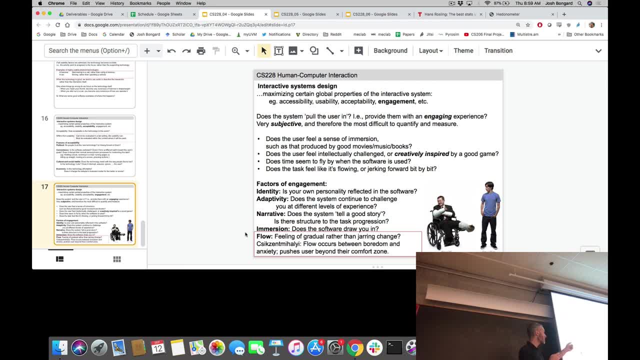 physically inside. physically inside. so you mentioned the oculus goggles. so you mentioned the oculus goggles. so you mentioned the oculus goggles for virtual reality. we'll spend a fair bit for virtual reality. we'll spend a fair bit for virtual reality. we'll spend a fair bit of time talking about virtual reality. 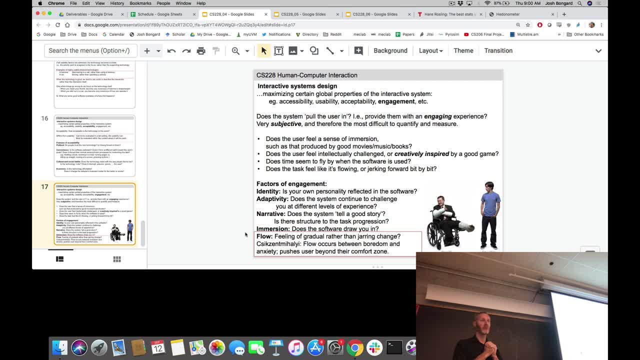 of time. talking about virtual reality of time. talking about virtual reality towards the end of the course, in the. towards the end of the course, in the. towards the end of the course, in the. looking inward, looking inward, looking inward. part of the course. what is it about? part of the course. what is it about? 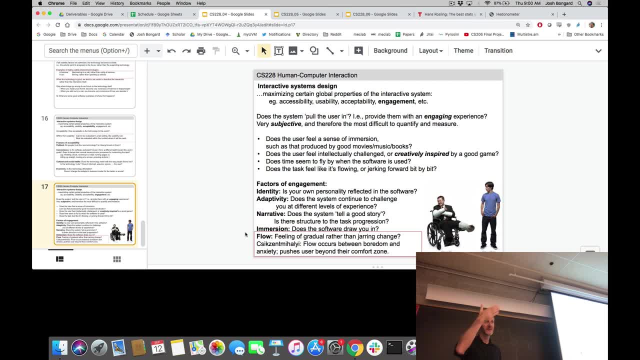 part of the course. what is it about the goggles that draws you in? you're the goggles that draws you in. you're the goggles that draws you in. you're obviously wearing them. so the screen is obviously wearing them. so the screen is obviously wearing them. so the screen is closer to your eyes. 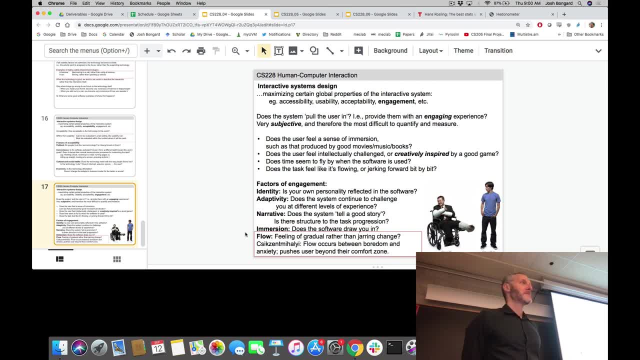 closer to your eyes. closer to your eyes, i'd say the most important factor in, i'd say the most important factor in, i'd say the most important factor in version is the progressive struggle version is the progressive struggle version is the progressive struggle. okay, through the events of the 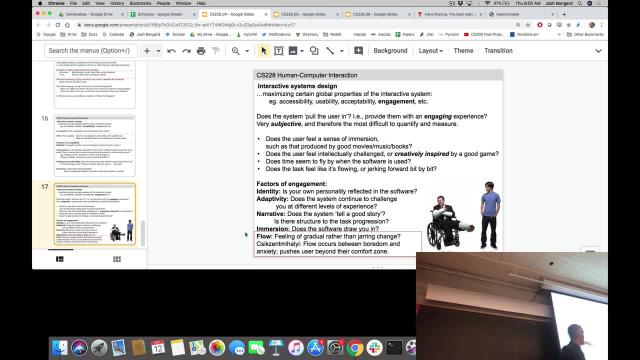 okay, through the events of the, okay, through the events of the activities in that technology activities in that technology activities in that technology, okay, the progressive struggle right. okay, the progressive struggle right. okay, the progressive struggle right, feeling challenged, somehow keeping them feeling challenged, somehow keeping them feeling challenged, somehow keeping them right at that level. yeah, definitely. 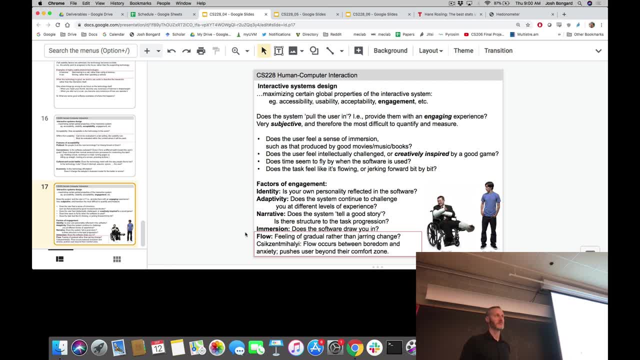 right at that level? yeah, definitely right at that level. yeah definitely, research the process and certain things. research the process and certain things. research the process and certain things become most acceptable over time, become most acceptable over time, become most acceptable over time because of the results okay, because of the results okay. 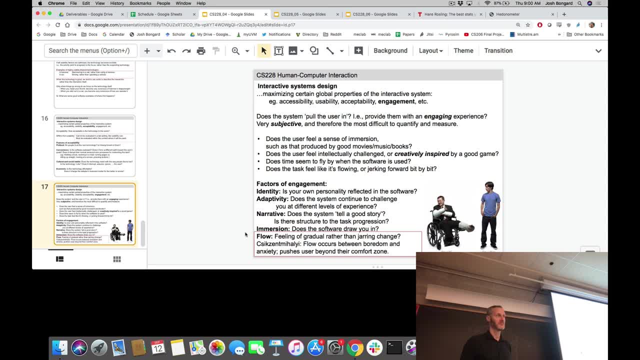 because of the results. okay, okay, okay, okay, wow, wow, wow. and then like mmo that evolved over, and then like mmo that evolved over, and then like mmo that evolved over time, because they realized the time, because they realized the time, because they realized the consequences of making it painful. 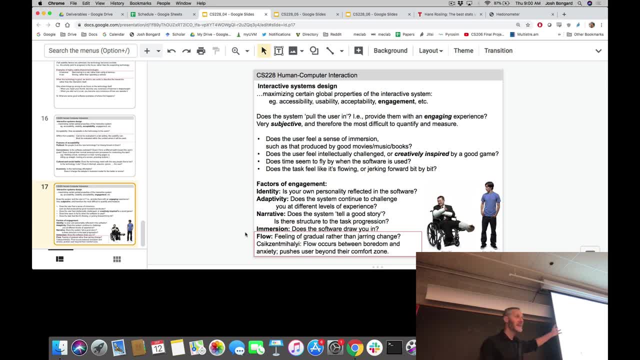 consequences of making it painful. consequences of making it painful: so interesting too much. so interesting too much. so interesting too much. exactly right the addictive or the. the exactly right, the addictive or the. the exactly right the addictive or the. the. the amount of effort needed to put in to. 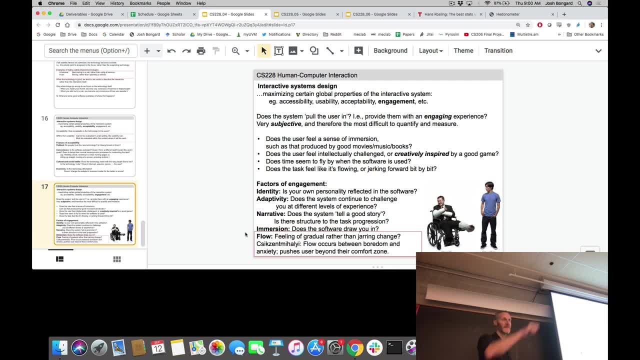 the amount of effort needed to put in to the amount of effort needed to put in to progress. that's important. let's come progress. that's important. let's come progress. that's important. let's come back to immersion. absolutely right, so you have this. absolutely right, so you have this. 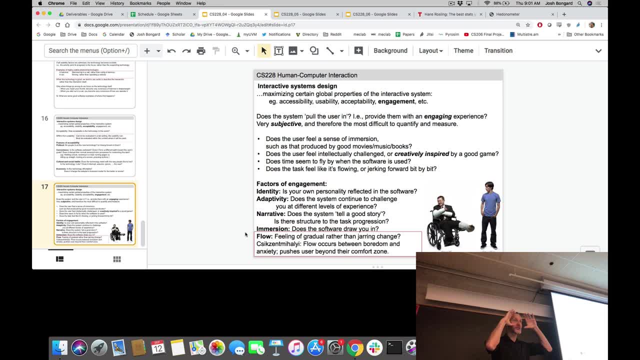 absolutely right. so you have this physical experience of putting on physical experience of putting on physical experience of putting on goggles if you put on actual goggles, goggles if you put on actual goggles. goggles if you put on actual goggles that have a pane of glass. there's that have a pane of glass, there's. 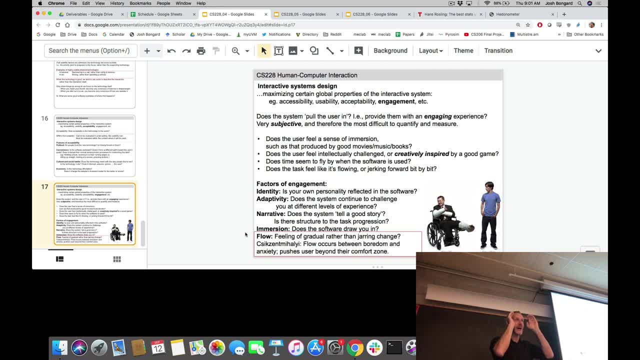 that have a pane of glass. there's usually some obstruction here, and you're usually some obstruction here, and you're usually some obstruction here and you're seeing through the glass, right. so when seeing through the glass, right. so when seeing through the glass, right so, when you put on the vr goggles, it casts the. 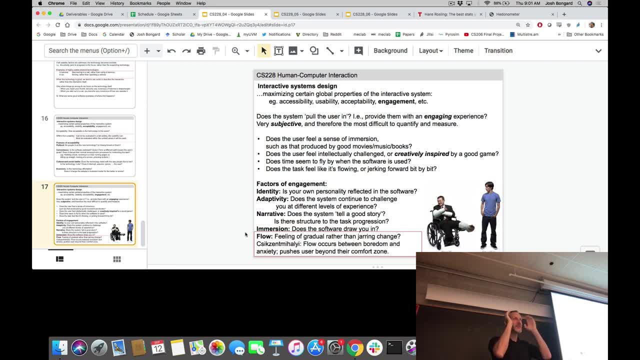 you put on the vr goggles, it casts the you put on the vr goggles, it casts the same illusion, same illusion, same illusion. so i'm expecting, as i wear the goggles, so i'm expecting, as i wear the goggles, so i'm expecting, as i wear the goggles, to have a similar experience to when i 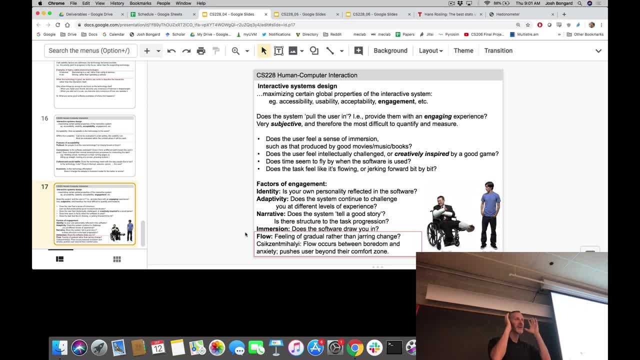 to have a similar experience to when i, to have a similar experience to when i wear actual goggles or glasses, or wear actual goggles or glasses, or wear actual goggles or glasses or something else similar. remember our something else similar. remember our something else similar. remember our discussion about when you're deploying. 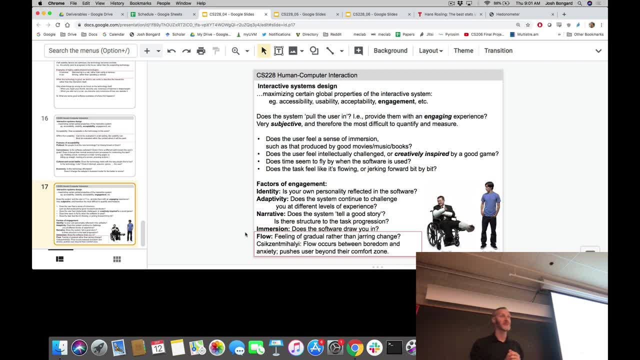 discussion about when you're deploying, discussion about when you're deploying new kinds of technology and vr- new kinds of technology and vr- new kinds of technology and vr definitely qualifies for a lot of people. definitely qualifies for a lot of people. definitely qualifies for a lot of people. they may be in the process of using vr. 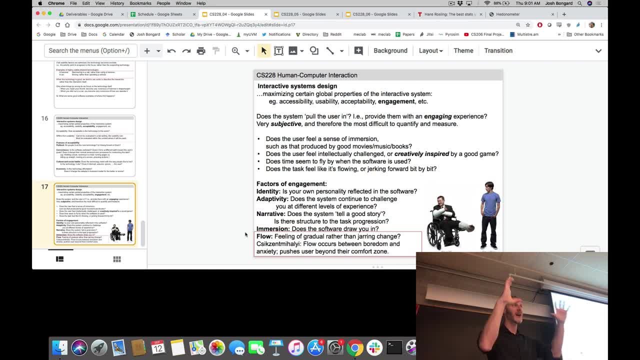 they may be in the process of using vr. they may be in the process of using vr for the first time. they have for the first time they have for the first time they have expectations about what's going to happen, expectations about what's going to happen, expectations about what's going to happen when they wear these goggles. what else is? 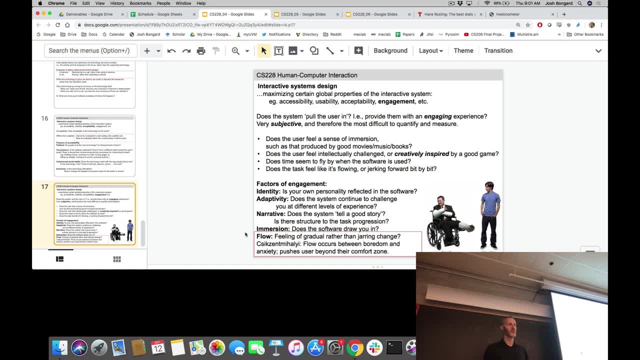 when they wear these goggles? what else is when they wear these goggles? what else is going on with vr goggles? that helps to going on with vr goggles. that helps to going on with vr goggles. that helps to create this illusion that you're looking. create this illusion that you're looking. 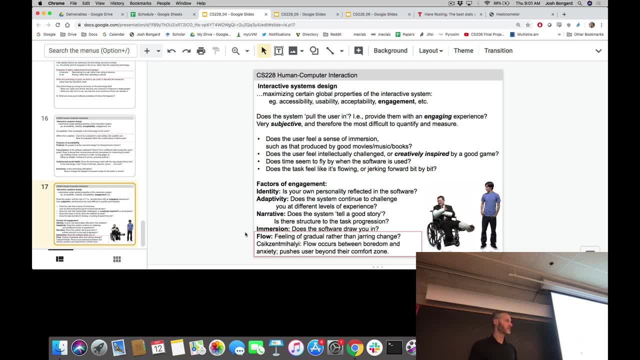 create this illusion that you're looking not at the, not at the physical world, not at the, not at the physical world, not at the, not at the physical world anymore. but this virtual world the way anymore. but this virtual world the way anymore. but this virtual world, the way it responds to the movement of your head. 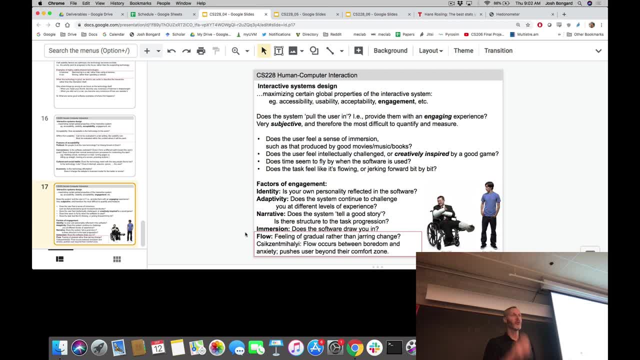 it responds to the movement of your head. it responds to the movement of your head, right. so there are sensors in the goggle right. so there are sensors in the goggle right. so there are sensors in the goggle that detect head orientation in the real, that detect head orientation in the real. 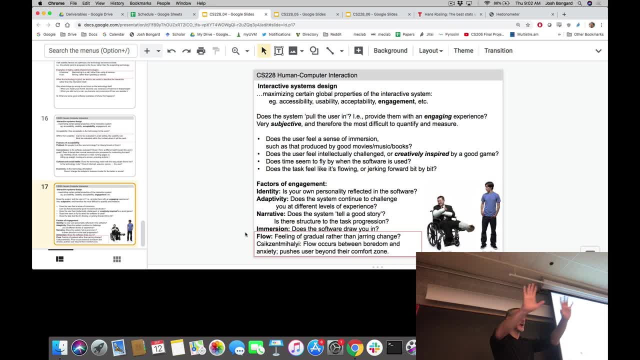 that detect head orientation in the real world. when I turn my head to the right world. when I turn my head to the right world. when I turn my head to the right- all of you. when I turn my head to the- all of you. when I turn my head to the- 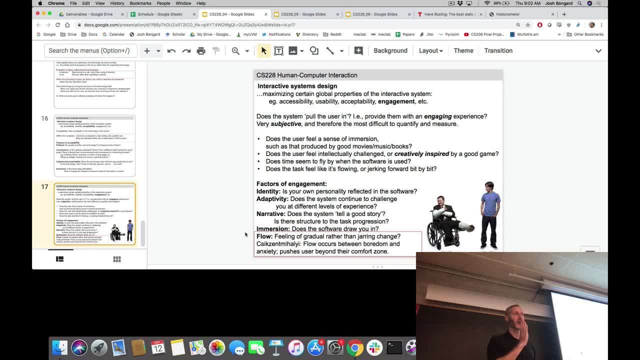 all of you. when I turn my head to the left, all of you flow to the right. the left- all of you flow to the right. the left, all of you flow to the right. the goggle detects movement of head to the goggle detects movement of head to the. 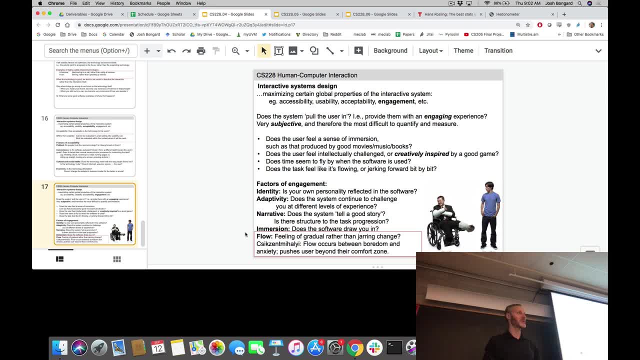 goggle detects movement of head to the left and updates the image so that left and updates the image so that left and updates the image so that everything in the image flows to the. everything in the image flows to the. everything in the image flows to the right, right. okay, that's one of dozens, or 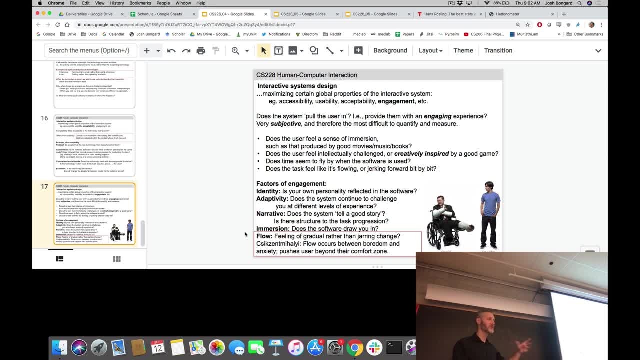 right, right, okay, that's one of dozens. or right right, okay, that's one of dozens, or hundreds of examples that need to be hundreds of examples, that need to be hundreds of examples that need to be built into VR to be able to create the built into VR to be able to create the. 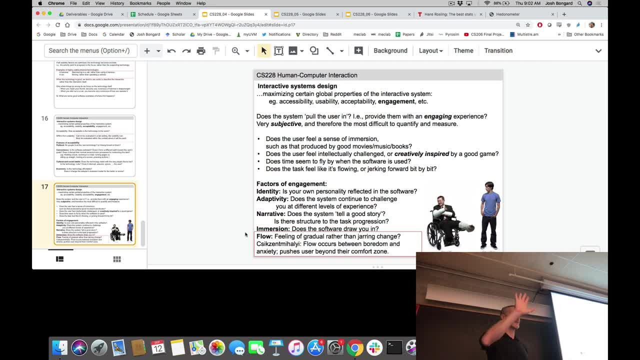 built into VR to be able to create the experience where suddenly the user goes experience where suddenly the user goes. experience where suddenly the user goes from realizing. they're looking at an from realizing. they're looking at an from realizing. they're looking at an illusion to feeling that they're. 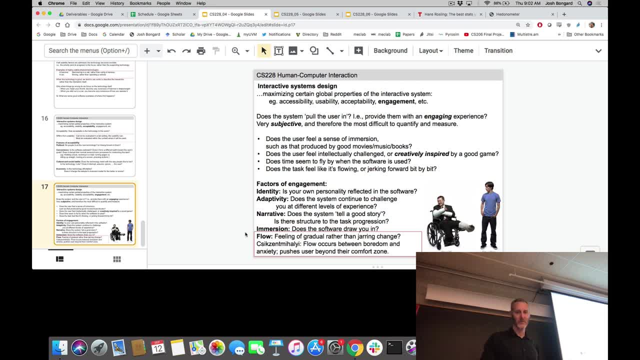 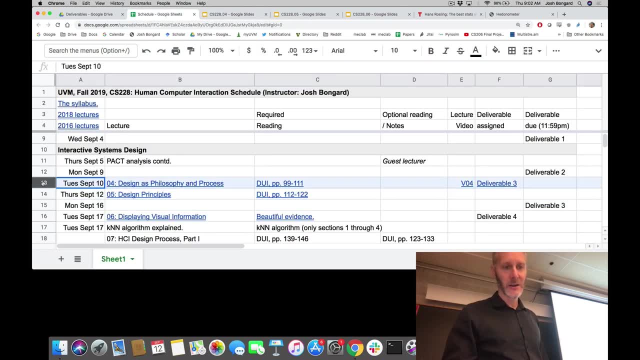 illusion, to feeling that they're illusion, to feeling that they're actually in this virtual environment, actually in this virtual environment, actually in this virtual environment. philosophy and process: so we can talk philosophy and process. so we can talk philosophy and process. so we can talk about different kinds of processes. 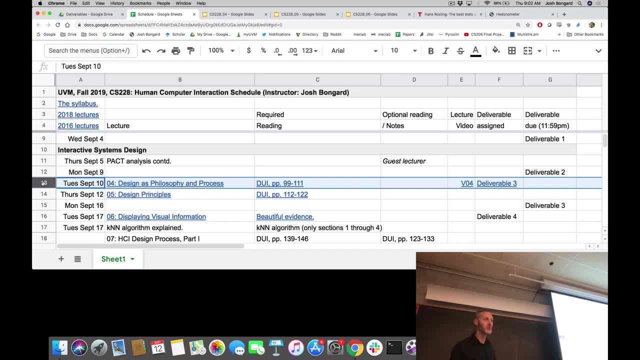 about different kinds of processes, about different kinds of processes, different ways to move down and try and different ways to move down and try and different ways to move down and try and measure and improve these things. we can measure and improve these things. we can measure and improve these things. we can elucidate lots of different design. 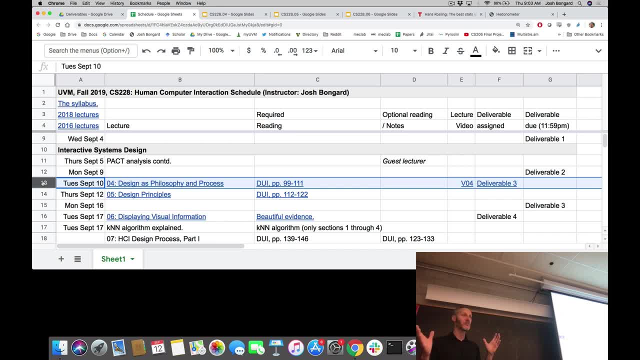 elucidate lots of different design, elucidate lots of different design processes, and then we can argue about processes, and then we can argue about processes, and then we can argue about which of those processes are better. which of those processes are better, which of those processes are better, depending on our design philosophy. 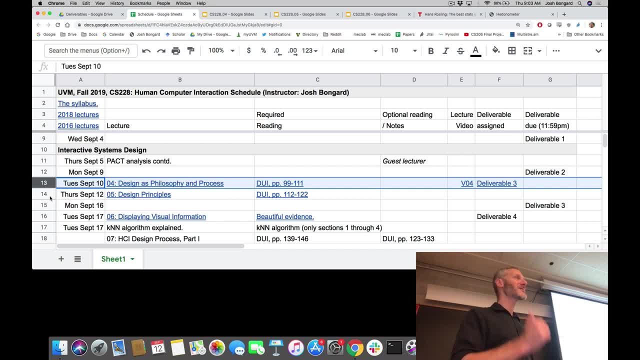 depending on our design philosophy, depending on our design philosophy, regardless of which process you choose, regardless of which process you choose, regardless of which process you choose, there are certain design principles or there are certain design principles, or there are certain design principles or rules of thumb that we want to try and 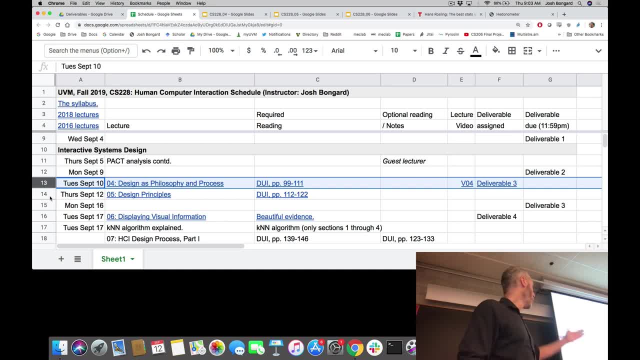 rules of thumb that we want to try and rules of thumb that we want to try and use when we are designing our hci system. use when we are designing our hci system. use when we are designing our hci system. one of those design principles is: 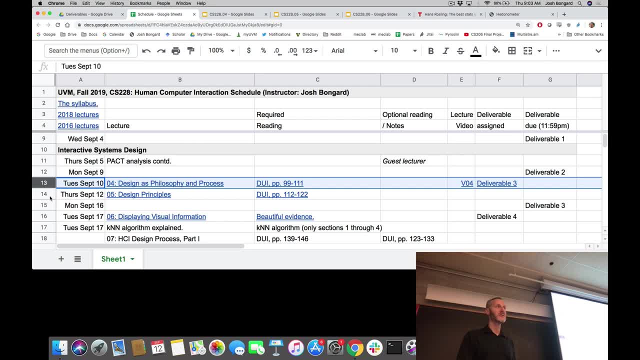 one of those design principles is. one of those design principles is something we just talked about. no matter something we just talked about, no matter something we just talked about. no matter what the technology is, people are going what the technology is. people are going what the technology is. people are going to bring their experiences from the 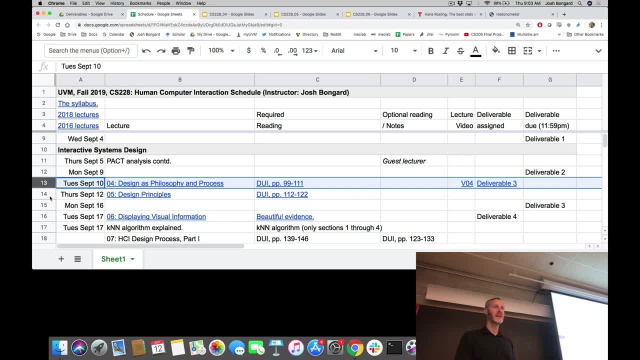 to bring their experiences from the, to bring their experiences from the physical world to bear on your system, physical world to bear on your system, physical world to bear on your system. they have expectations when they're they have expectations when they're looking at something and they move. 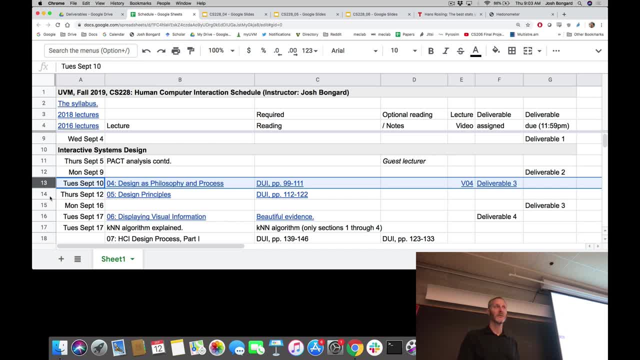 looking at something and they move looking at something and they move their head about what the result will be. their head about what the result will be. their head about what the result will be: right your software, whatever it is, should right. your software, whatever it is, should right. your software, whatever it is, should support those expectations as best you. 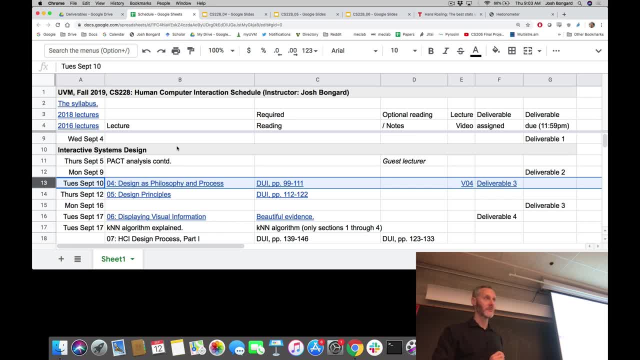 support those expectations as best you. support those expectations as best you can. yes on your slide. the non-functional can: yes on your slide. the non-functional can: yes on your slide. the non-functional set: you've had those four set. you've had those four set. you've had those four requirements right there, plus etc. so 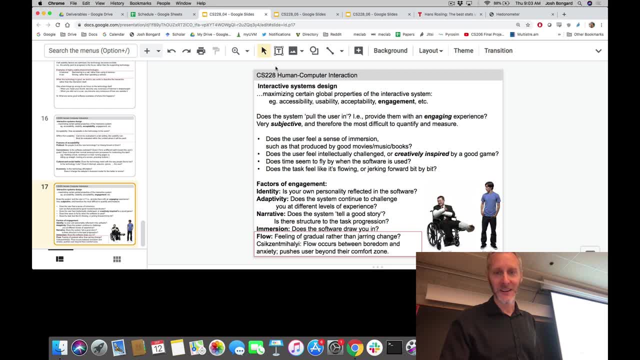 requirements right there plus etc. so requirements right there plus etc. so what else falls in your league plus etc. what else falls in your league plus etc. what else falls in your league plus etc. good question, okay, so uh, it's again. good question, okay, so uh, it's again. 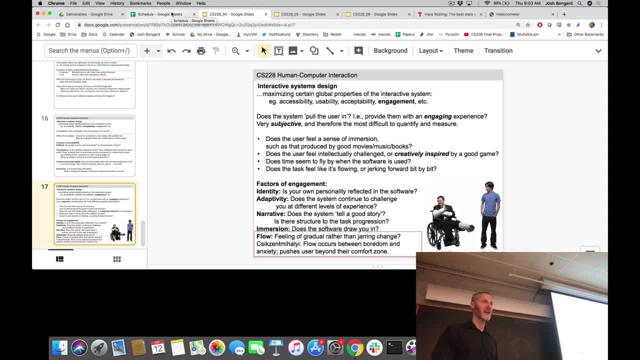 good question, okay, so, uh, it's again something that's not specifically about something that's not specifically about something that's not specifically about the function itself, but something that's the function itself, but something that's the function itself, but something that's beyond just the function, right? so the 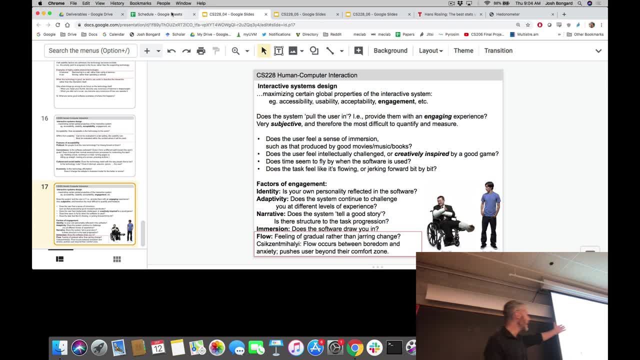 beyond just the function. right, so the beyond, just the function. right so the system. the user is frustrated with the system. the user is frustrated with the system. the user is frustrated with the system. why it may not necessarily be an system, why it may not necessarily be an. 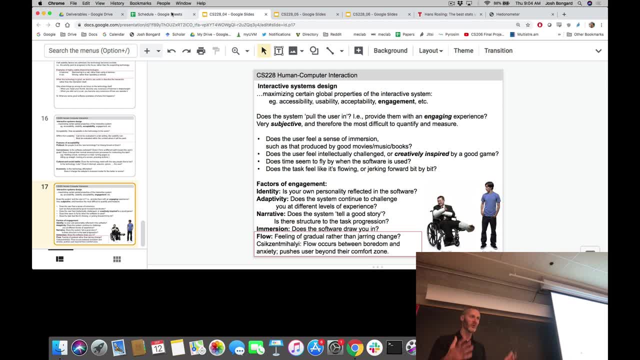 system, why it may not necessarily be an acceptable engaging usability or acceptable engaging usability or acceptable engaging usability or accessible issue. it's it's something else. accessible issue- it's it's something else. accessible issue- it's it's something else. right? so we're looking at this level. 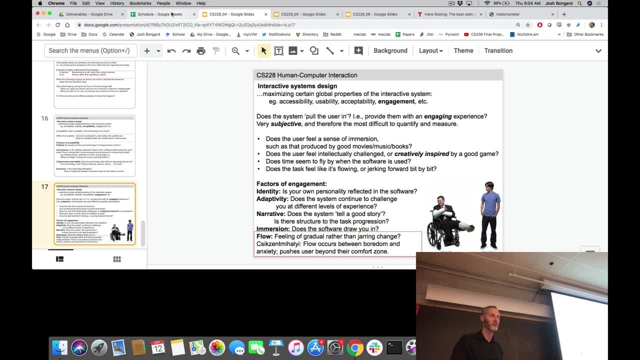 right. so we're looking at this level, right, so we're looking at this level for those other things. so that's what for those other things? so that's what for those other things. so that's what the etc is meant for there's other, the etc is meant for there's other. 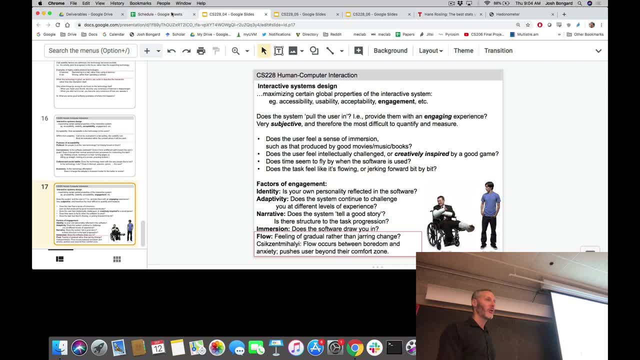 the etc is meant for. there's other things beyond what we've talked about. things beyond what we've talked about, things beyond what we've talked about here that might affect whether someone here. that might affect whether someone here. that might affect whether someone chooses your system over. 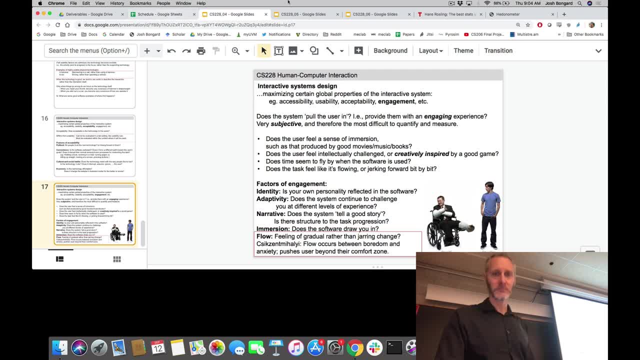 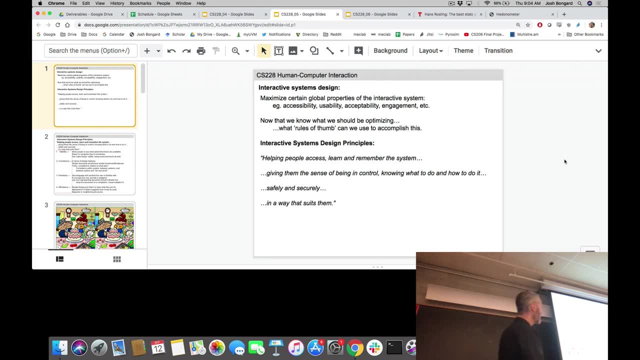 chooses your system over, chooses your system over another. okay, so let's move on now and talk about: okay, so let's move on now and talk about: okay, so let's move on now and talk about design, design, design, principles, principles, principles. so we know what we're trying to. 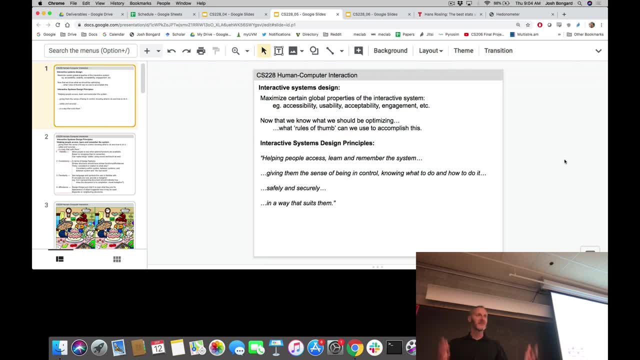 so we know what we're trying to. so we know what we're trying to optimize. which are things that make the optimize? which are things that make the optimize? which are things that make the system desirable to the user. they might system desirable to the user, they might. 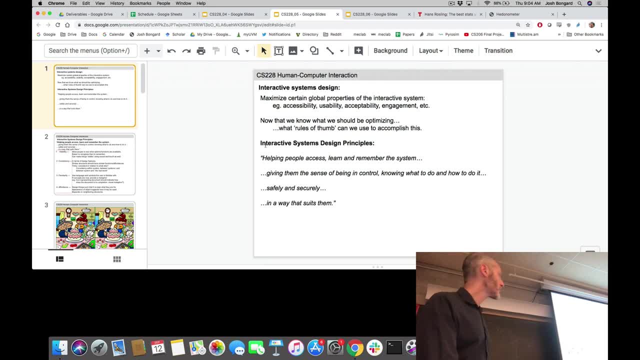 system desirable to the user, they might choose it over others, choose it over others, choose it over others. how do we sort of, how do we sort of, how do we sort of apply some rules of thumbs to do this in- apply some rules of thumbs to do this in. 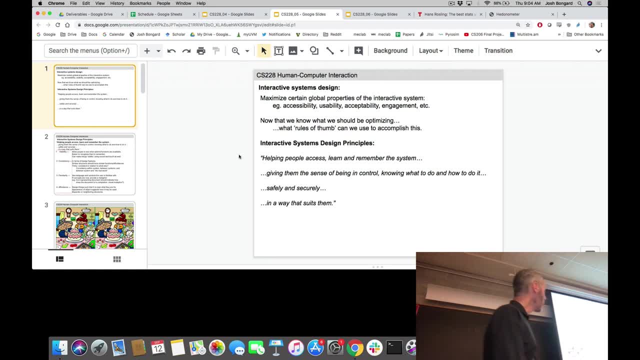 apply some rules of thumbs to do this in the book, the book, the book in the reading. it mentions helping people in the reading. it mentions helping people in the reading. it mentions helping people access, learn and remember the system. access, learn and remember the system. access, learn and remember the system, giving the sense of being in control. and 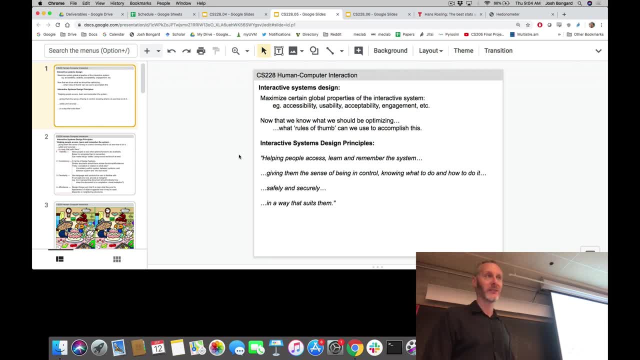 giving the sense of being in control. and giving the sense of being in control and knowing what to do and how to do it. knowing what to do and how to do it. knowing what to do and how to do it safely and securely, in a way that suits. 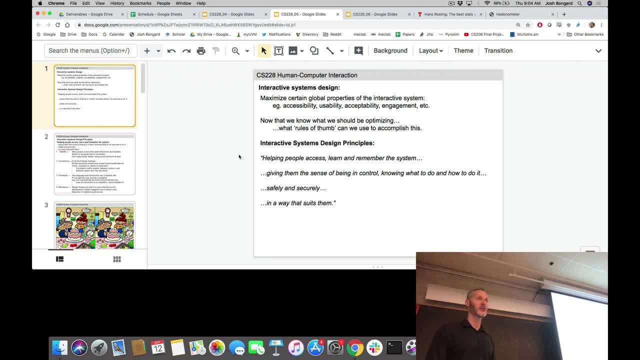 safely and securely in a way that suits safely and securely in a way that suits them. it's a mouthful, and again full of a them. it's a mouthful, and again full of a them. it's a mouthful, and again full of a lot of vague terms. 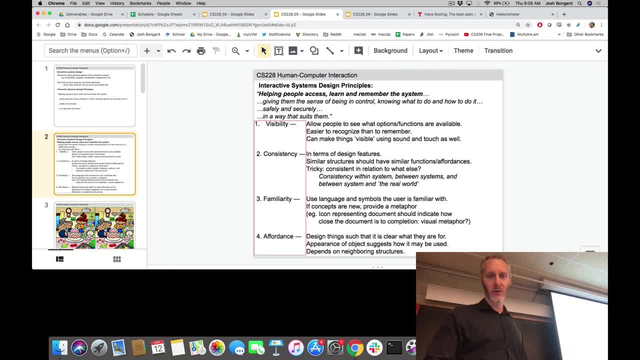 lot of vague terms. lot of vague terms. so we're going to try and take these. so we're going to try and take these. so we're going to try and take these terms and we're going to gradually walk terms and we're going to gradually walk. 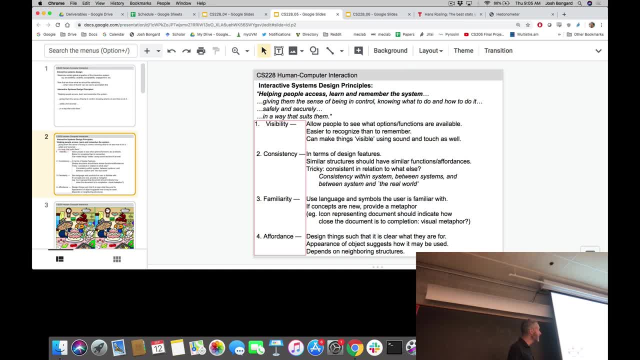 terms and we're going to gradually walk through in this lecture, through in this lecture through in this lecture: 12 features underneath here: 12 design. 12 features underneath here: 12 design. 12 features underneath here: 12 design principles, principles, principles that can help you improve the various 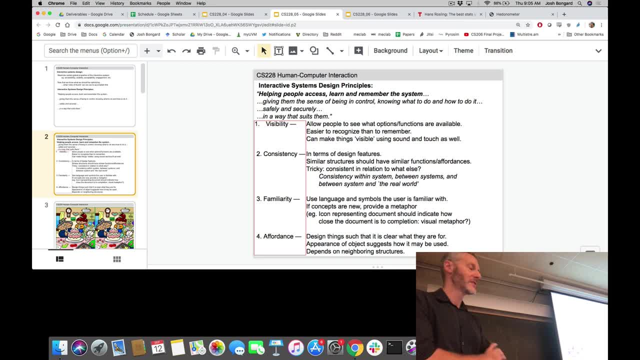 that can help you improve the various that can help you improve the various non-functional requirements of an non-functional requirements of an non-functional requirements of an interactive system. interactive system, interactive system. let's start again, as always, with some. let's start again, as always, with some. 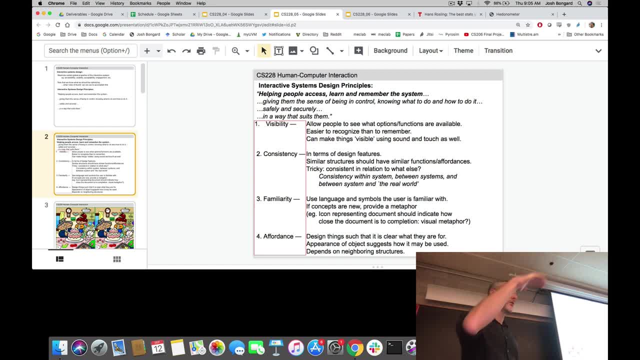 let's start again, as always, with some of the more obvious things, and we'll march of the more obvious things, and we'll march of the more obvious things, and we'll march in this set of 12 design principles, in this set of 12 design principles. 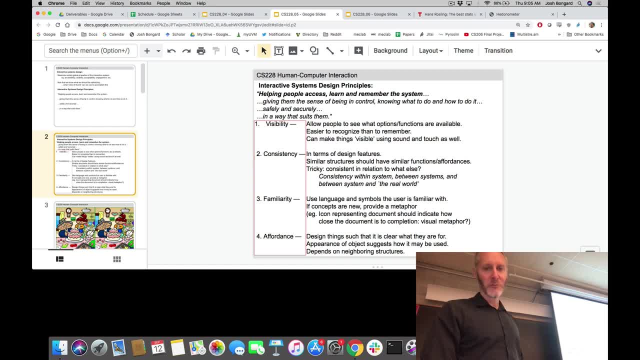 in this set of 12 design principles, to some, that are less obvious, to some that are less obvious, to some that are less obvious. let's start with visibility, so we want. let's start with visibility, so we want. let's start with visibility, so we want to make. 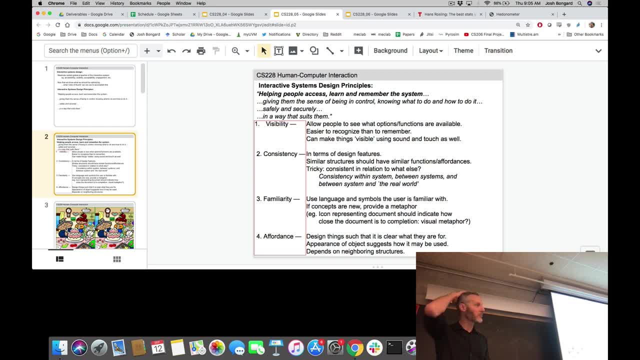 to make, to make aspects of our system visible. if our aspects of our system visible, if our aspects of our system visible, if our system is a black box system is a black box system is a black box. it's the user is going to get confused. it's the user is going to get confused. 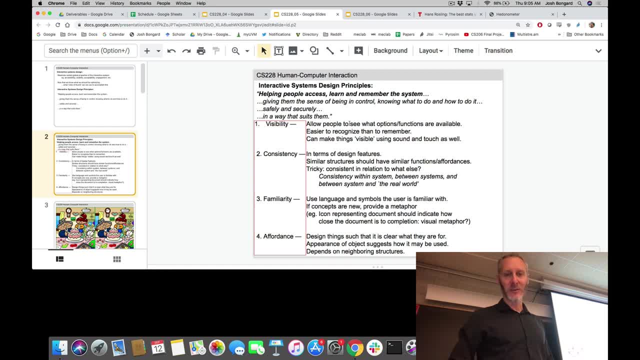 it's, the user is going to get confused very quickly. so the obvious thing we can very quickly, so the obvious thing we can very quickly, so the obvious thing we can do is obviously do is obviously do is obviously allow people to see what options, and allow people to see what options and 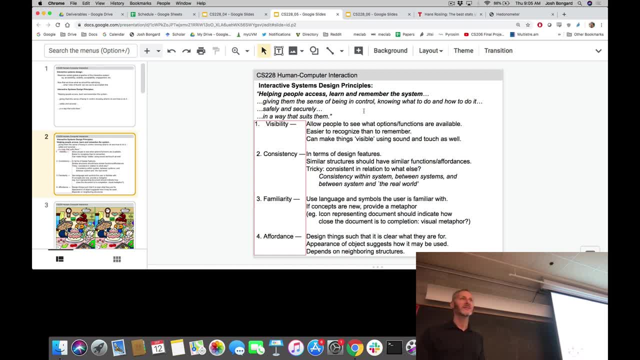 allow people to see what options and functions are available. functions are available. functions are available. display them in a way that makes them display them in a way that makes them display them in a way that makes them easy to remember, easy to learn, easy to remember, easy to learn. 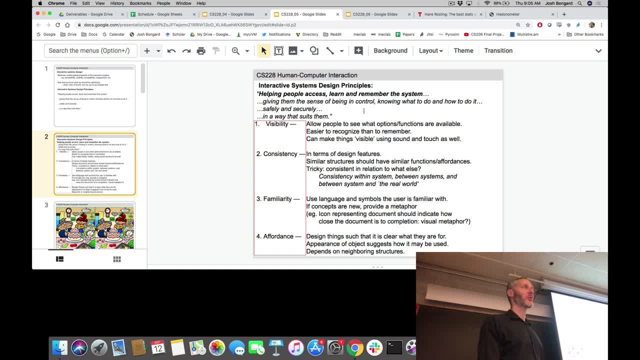 easy to remember, easy to learn. there's lots of ways of getting this. there's lots of ways of getting this. there's lots of ways of getting this. wrong, wrong, wrong. what are some of the wrong ways of what are some of the wrong ways of what are some of the wrong ways of making a system visible? 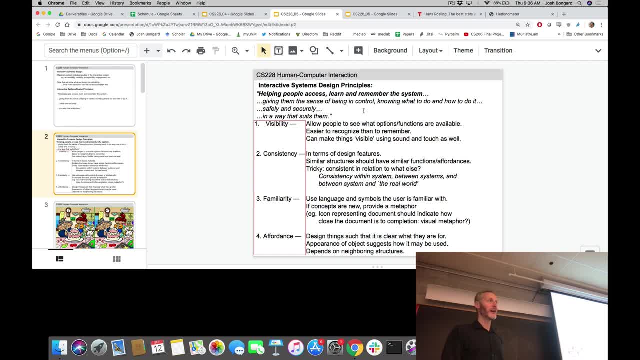 making a system visible. making a system visible. we have too much information. we have too much information. we have too much information, absolutely right. so remember the google. absolutely right, so remember the google, absolutely right. so remember the google landing page. landing page. landing page. there's a little bit of information. 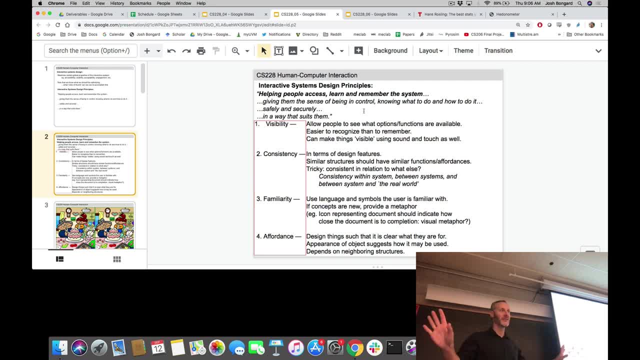 there's a little bit of information. there's a little bit of information there about what you can do there, about what you can do there, about what you can do on the google main page, and that's it on the google main page. and that's it on the google main page and that's it. the rest is white space, right? so? 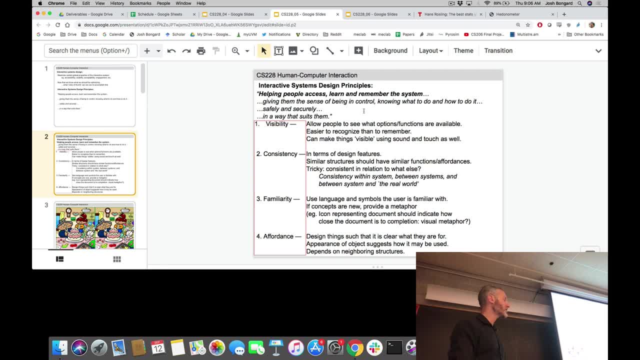 the rest is white space, right? so the rest is white space, right? so we want to make the functions, uh, we, we want to make the functions. uh, we, we want to make the functions. uh, we want to. we want to suggest how, the want to. we want to suggest how the. 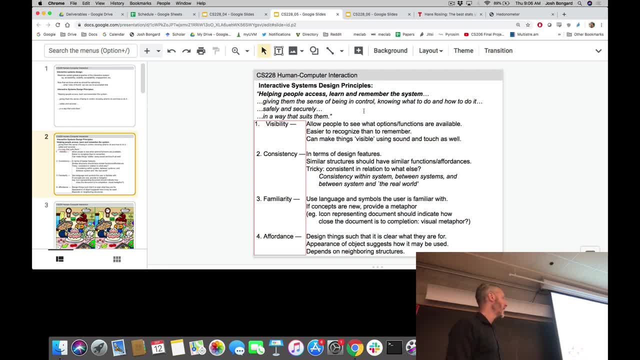 want to, we want to suggest how the system can be used by system, can be used by system, can be used by displaying various functions but not displaying various functions but not displaying various functions, but not too much, and again on the surface that too much and again on the surface that. 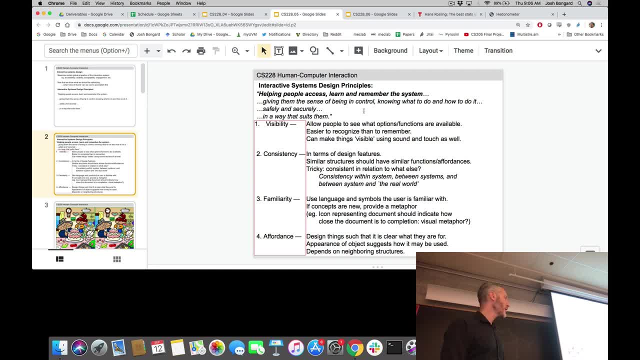 too much. and again, on the surface that sounds easy but kind of difficult to do. sounds easy but kind of difficult to do, sounds easy but kind of difficult to do. think about the system that you're think about, the system that you're think about the system that you're developing with the leap motion device. 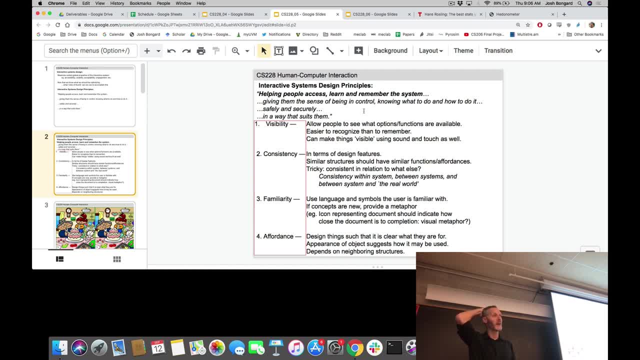 developing with the leap motion device. developing with the leap motion device later on in this semester. you're going later on in this semester. you're going later on in this semester you're going to put this device down in front of. to put this device down in front of. 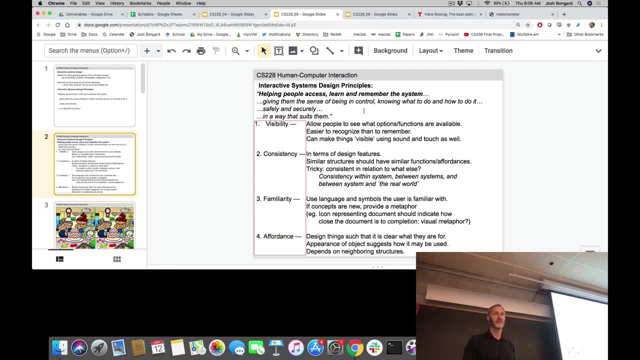 to put this device down in front of in front of family members, in front of family members, in front of family members, and say: have at it, the game is you're. and say: have at it, the game is you're. and say: have at it, the game is you're not allowed to tell them how to use. 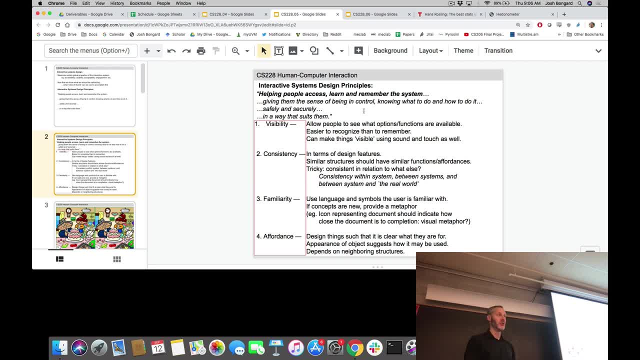 not allowed to tell them how to use, not allowed to tell them how to use the system, the system, the system. the first thing you'll probably want to, the first thing you'll probably want to, the first thing you'll probably want to do, is the moment they bring their hand. 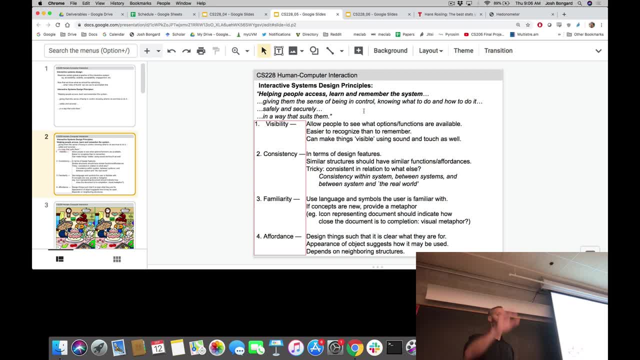 do is the moment they bring their hand do is the moment they bring their hand or hands over the device. they see this, or hands over the device. they see this, or hands over the device. they see this. wireframe of a hand right the moment. wireframe of a hand right the moment. 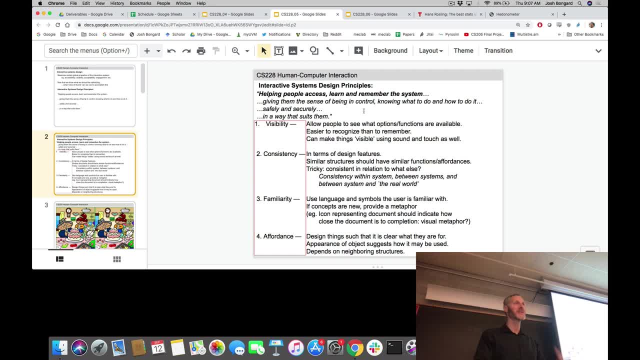 wireframe of a hand, right the moment. they see that wireframe of the hand. they see that wireframe of the hand. they see that wireframe of the hand. you've communicated a lot of what your. you've communicated a lot of what your. you've communicated a lot of what your system does. 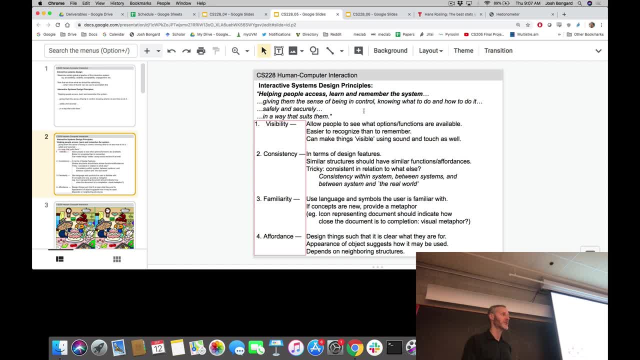 system does, system does, but maybe not everything right at some, but maybe not everything right at some, but maybe not everything right at some point you're going to turn your system point. you're going to turn your system point. you're going to turn your system into an educational game. how do you? 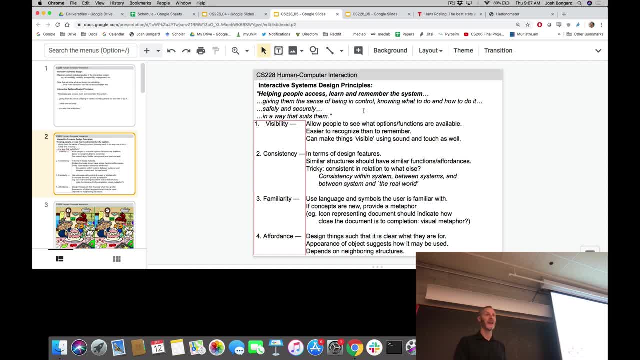 into an educational game. how do you into an educational game, how do you signal to the users that they can signal to the users, that they can signal to the users that they can actually learn asl using the system, actually learn asl using the system, actually learn asl using the system, above and beyond just waving your hand. 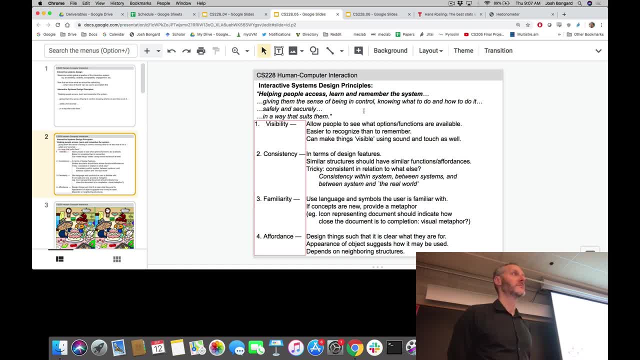 above and beyond just waving your hand, above and beyond just waving your hand over the device, over the device, over the device, we could put text to the screen. we're we could put text to the screen. we're we could put text to the screen. we're going to assume for this course that 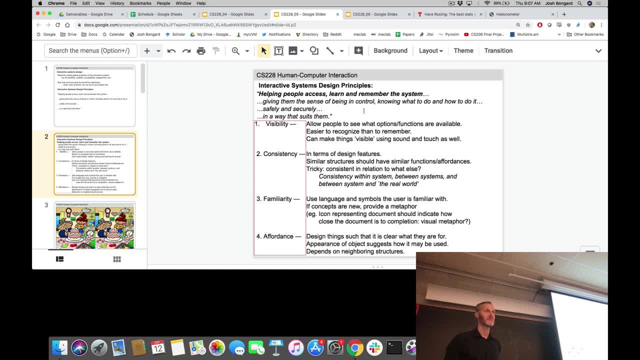 going to assume for this course that going to assume, for this course, that whoever is using your system does not whoever is using your system does not. whoever is using your system does not speak or read english. speak or read english. speak or read english. no paragraph is of explanatory text. 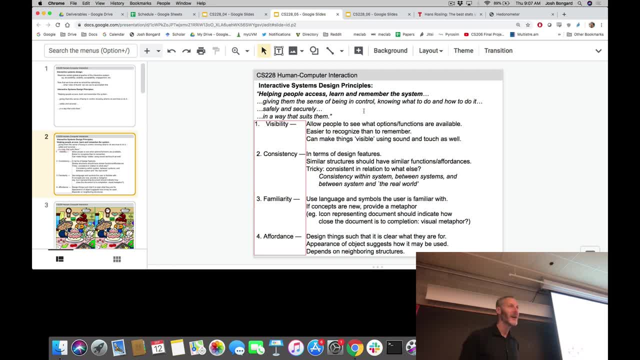 no paragraph is of explanatory text. no paragraph is of explanatory text because now we made the system overly. because now we made the system overly, because now we made the system overly visible, they've got to sit there visible. they've got to sit there visible. they've got to sit there and read the fine print before they use. 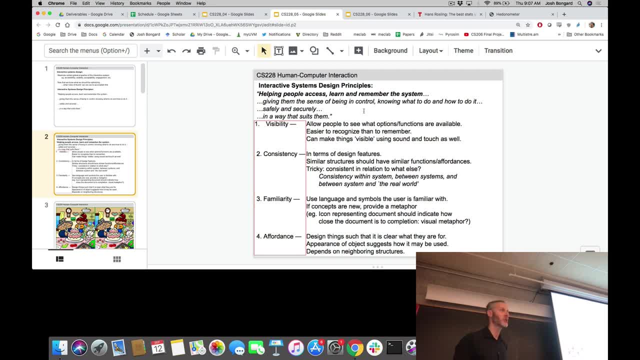 and read the fine print before they use. and read the fine print before they use. it probably not acceptable. how many of it probably not acceptable? how many of it probably not acceptable? how many of you read the tutorials for new apps? you read the tutorials for new apps. 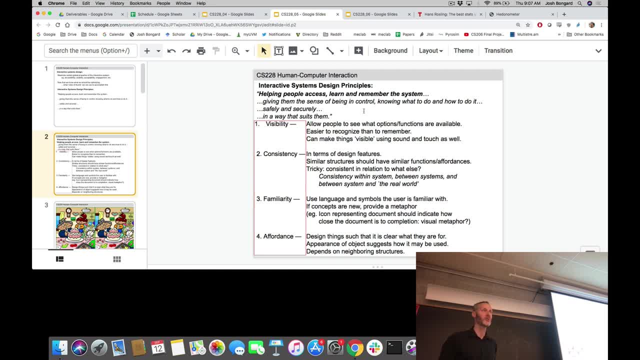 you read the tutorials for new apps. i don't know if they even make. i don't know if they even make. i don't know if they even make tutorials for apps anymore, right, it's tutorials for apps anymore. right, it's tutorials for apps anymore. right. it's absolutely unacceptable. so we're going. 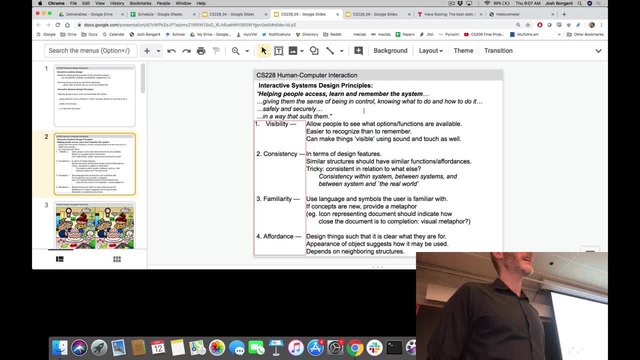 absolutely unacceptable. so we're going absolutely unacceptable. so we're going to have to do it without to do it, without to do it without text. so now we're back in hci land text. so now we're back in hci land text. so now we're back in hci land. right, we're going to have to use. 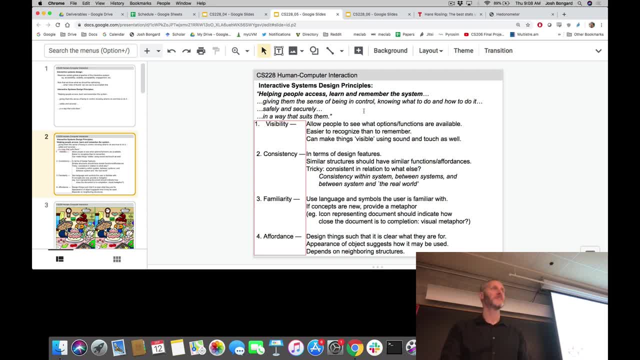 right, we're going to have to use- right, we're going to have to use- visual hints to communicate how the visual hints to communicate, how the visual hints to communicate how the system can be used. absolutely, that's a great example, right, absolutely, that's a great example, right. 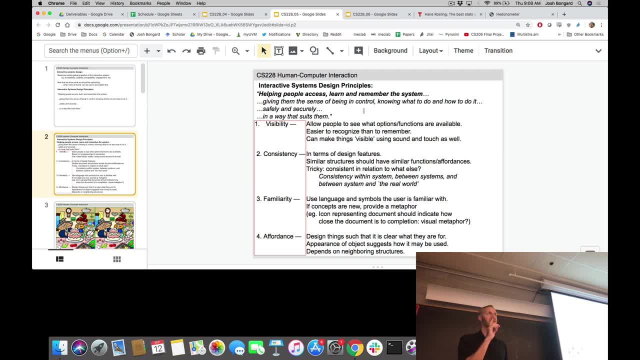 absolutely. that's a great example, right? the little robot says do or show. the little robot says do or show. the little robot says do or show. signals doesn't say do what i do. signals doesn't say do what i do. signals doesn't say do what i do. we've already mentioned that users bring. 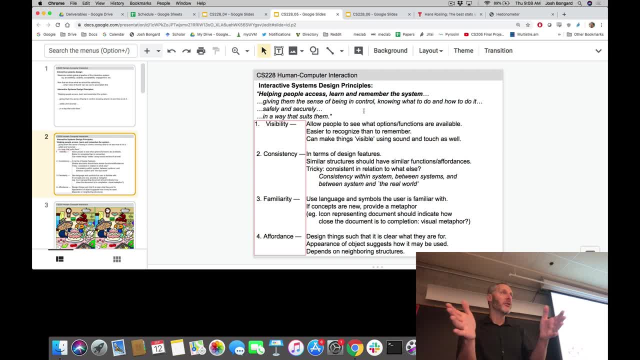 we've already mentioned that users bring. we've already mentioned that users bring their expectations about the physical, their expectations about the physical, their expectations about the physical world to bear on a new interactive world, to bear on a new interactive world, to bear on a new interactive technology. they also bring their 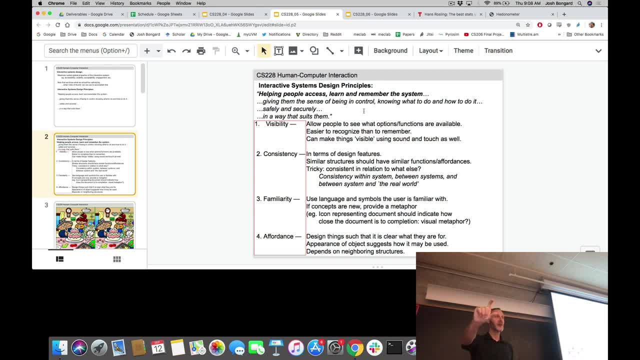 technology. they also bring their technology, they also bring their expectations about social interactions, expectations about social interactions, expectations about social interactions. so the moment you flash up a little, so the moment you flash up a little, so the moment you flash up a little avatar or a robot, you're already. 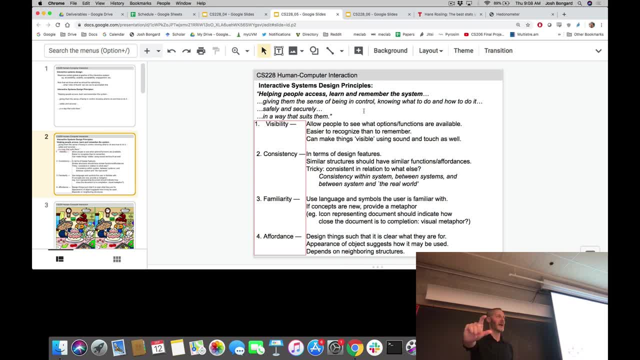 avatar or a robot. you're already avatar or a robot. you're already signaling. bring your social signaling, bring your social signaling, bring your social expectations to bear on this. i'm a expectations to bear on this. i'm a expectations to bear on this. i'm a little robot and i'm looking out at the 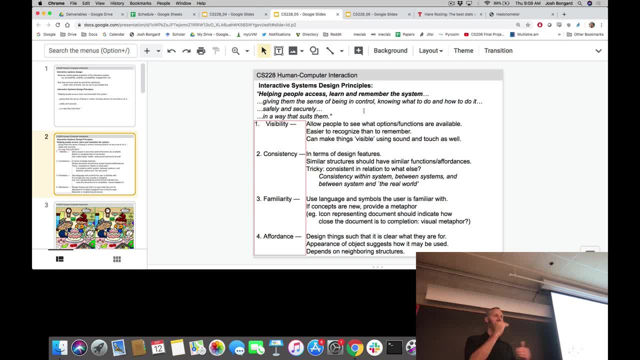 little robot and i'm looking out at the little robot and i'm looking out at the screen at you, right, without any text screen at you, right, without any text screen at you, right, without any text. you're already setting the stage for what. you're already setting the stage for what? 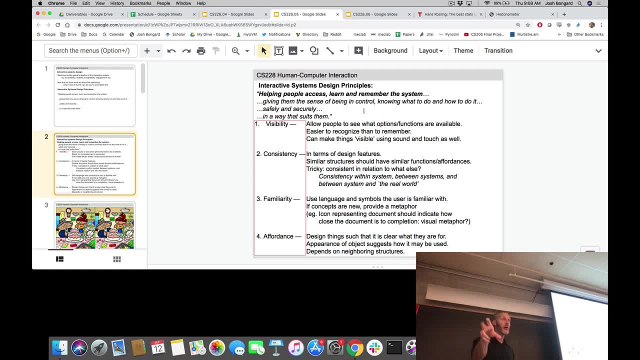 you're already setting the stage for what the user can expect. the user can expect, the user can expect if this little robot or the owl, or if this little robot or the owl, or if this little robot or the owl or whatever it is, the avatar starts to do. 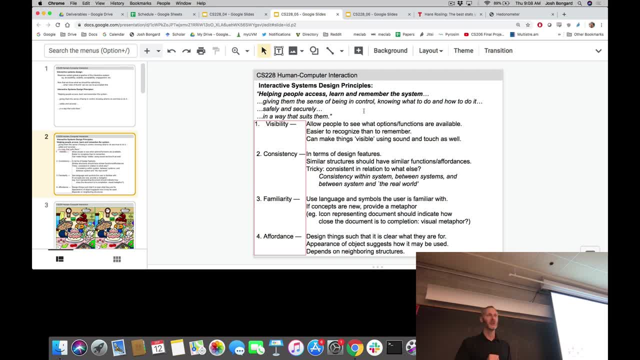 whatever it is the avatar starts to do, whatever it is the avatar starts to do something without having to say it most something, without having to say it most something, without having to say it, most users will realize it wants me to do. users will realize it wants me to do. 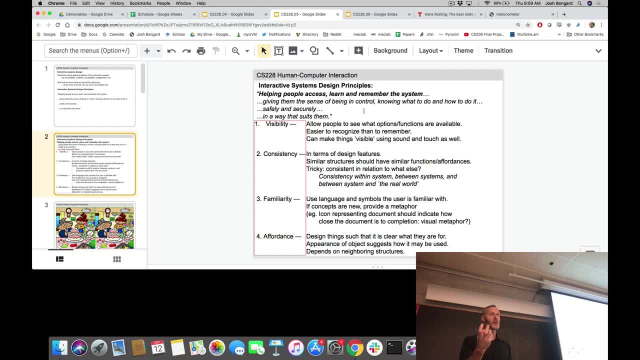 users will realize it wants me to do what it's doing right, very, very simple. what it's doing right very, very simple. what it's doing right very, very simple: it's exploiting the expect social. it's exploiting the expect social. it's exploiting the expect social expectations that user brings to bear on. 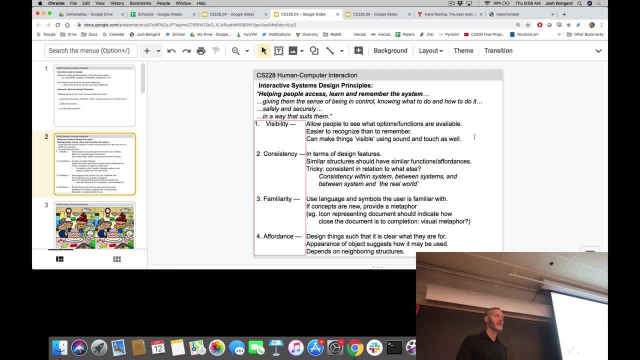 expectations that user brings to bear. on expectations that user brings to bear on the system, the system, the system. okay. how else can we make this system okay? how else can we make this system okay? how else can we make this system visible, aside from just showing things visible, aside from just showing things. 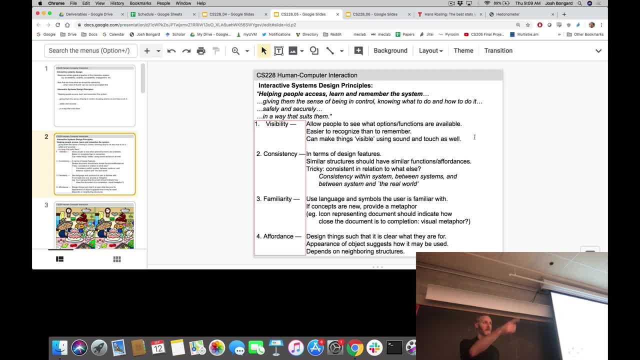 visible, aside from just showing things on the screen. we can move to sound and touch well we. we can move to sound and touch well we. we can move to sound and touch well we. could. we can move beyond the example of could. we can move beyond the example of. 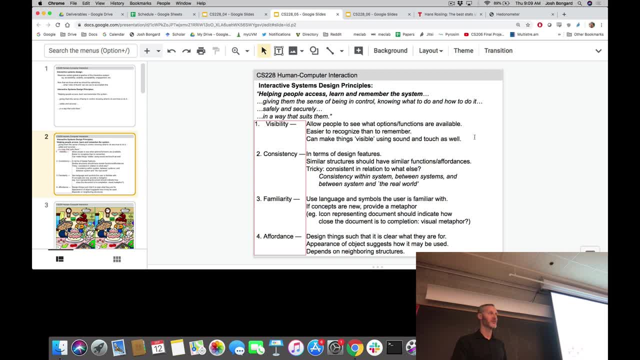 could. we can move beyond the example of the motion now. what kinds of technology the motion now? what kinds of technology? the motion now. what kinds of technology communicate information to you outside? communicate information to you outside? communicate information to you outside of the visual sense, of the visual sense? 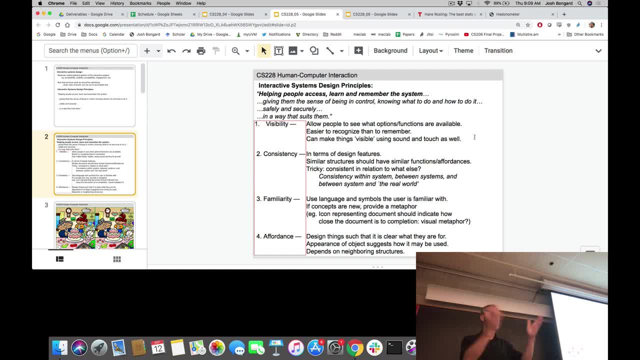 of the visual sense, your phone right, so you might have set your phone right. so you might have set your phone right, so you might have set your phone to vibrate if you receive a. your phone to vibrate if you receive a. your phone to vibrate if you receive a text message from a certain person, right. 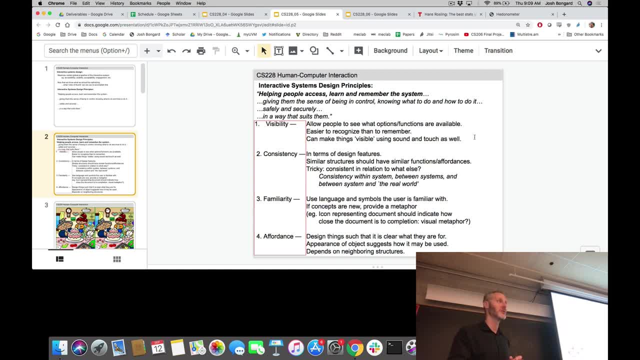 text message from a certain person, right. text message from a certain person, right? something urgent that you're trying to something urgent, that you're trying to something urgent that you're trying to monitor. it'll only interrupt you in monitor. it'll only interrupt you in monitor. it'll only interrupt you in those cases, right? 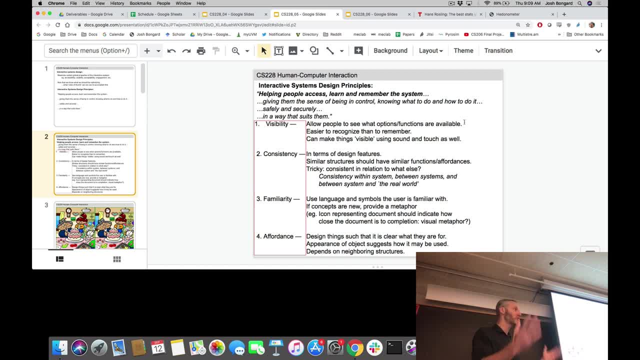 those cases right, those cases right. important to get those kinds of things. important to get those kinds of things. important to get those kinds of things right for most of us. we're drowning in right for most of us. we're drowning in right for most of us. we're drowning in notifications these days. so, with all the 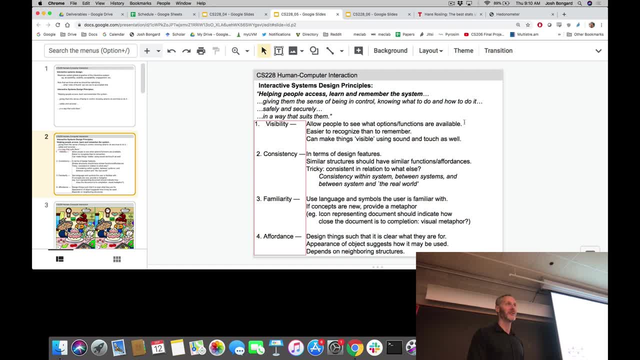 notifications these days, so with all the notifications these days, so with all the technology that we now use. it's a little technology that we now use. it's a little technology that we now use. it's a little bit too visible, right, people are trying. bit too visible, right, people are trying. 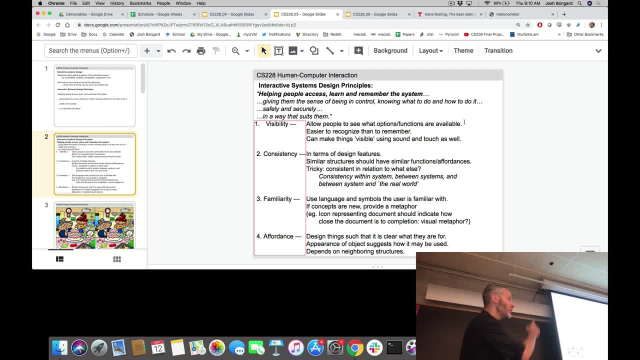 bit too visible. right, people are trying to figure out how to make things less, to figure out how to make things less, to figure out how to make things less visible and how to tune our devices to visible, and how to tune our devices to visible and how to tune our devices to only communicate the right information. 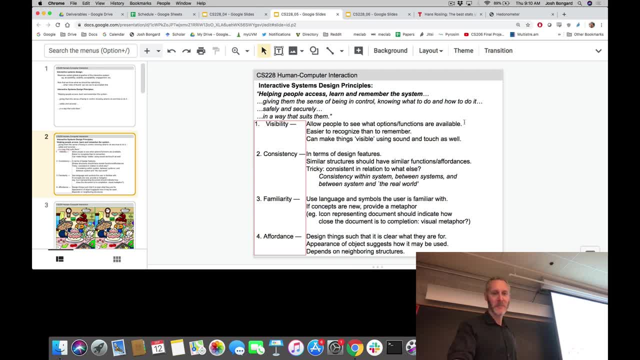 only communicate the right information, only communicate the right information to us at the right time. tricky to get to us at the right time. tricky to get to us at the right time. tricky to get that one right. we also want to try. and that one right. we also want to try and. 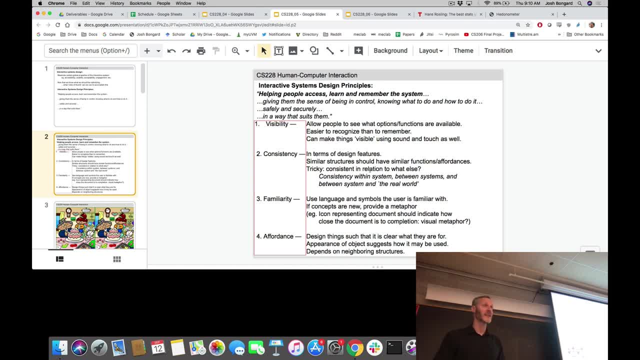 that one right. we also want to try and make our system consistent, and this again make our system consistent and this again make our system consistent. and this again goes back to this idea of expectations, goes back to this idea of expectations, goes back to this idea of expectations and prediction. you don't want a user. 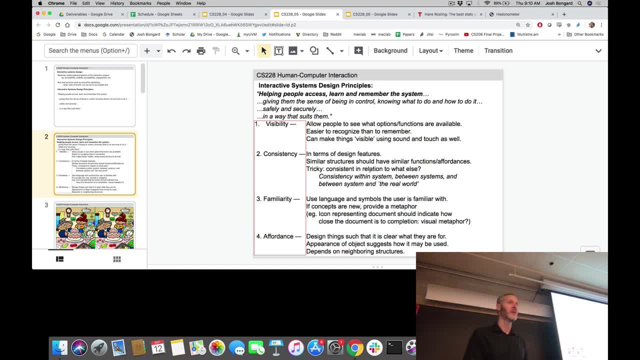 and prediction. you don't want a user and prediction. you don't want a user having to try and relearn every new, having to try and relearn every new, having to try and relearn every new software system from scratch. there's some software system from scratch, there's some. 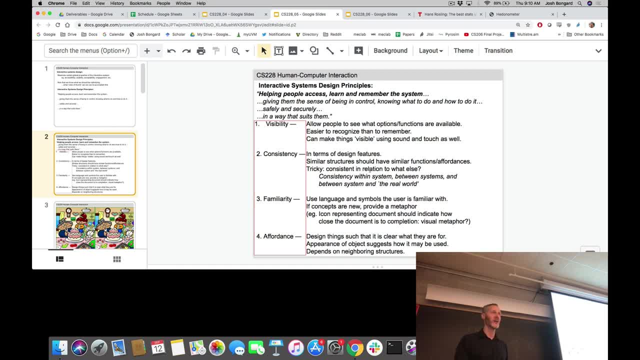 software system from scratch. there's some obvious consistent design features. obvious consistent design features. obvious consistent design features that are out there. if you download any that are out there, if you download any that are out there, if you download any new app, what do you expect to see when? 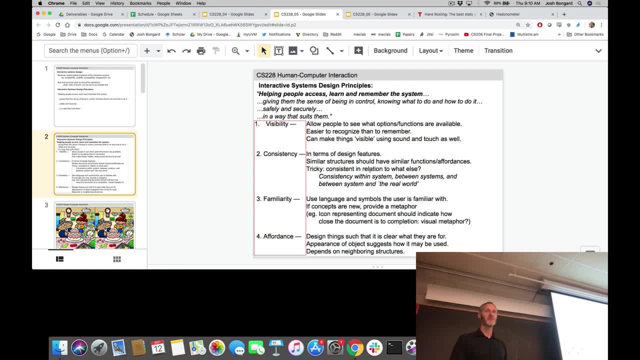 new app. what do you expect to see when new app? what do you expect to see when you start up the app? what are some you start up the app. what are some you start up the app. what are some things that have to be consistent across, things that have to be consistent across. 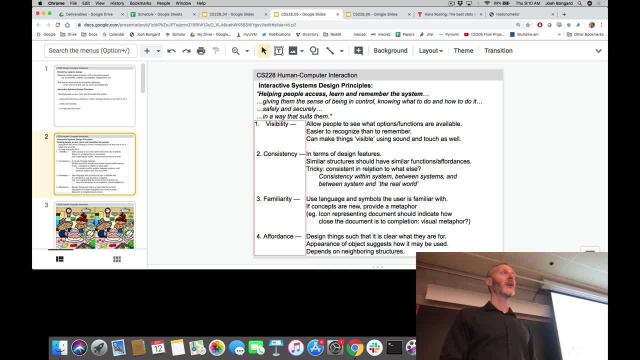 things that have to be consistent across apps. okay, right, so there's usually a apps. okay, right, so there's usually a apps. okay, right, so there's usually a splash screen or a login. you're usually splash screen or a login. you're usually splash screen or a login. you're usually not dumped directly into the app itself. 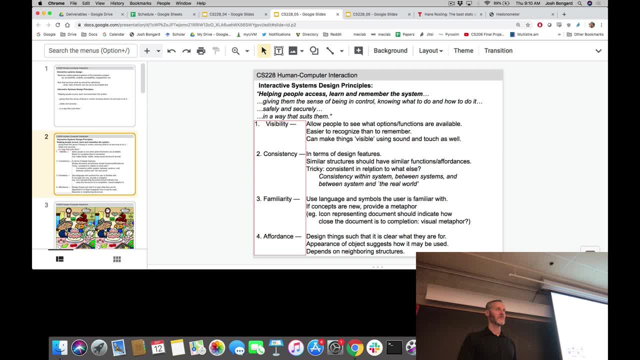 not dumped directly into the app itself. not dumped directly into the app itself. what else the app starts up and I see what else the app starts up and I see what else the app starts up and I see the splash page. I don't like this app. the splash page. I don't like this app. 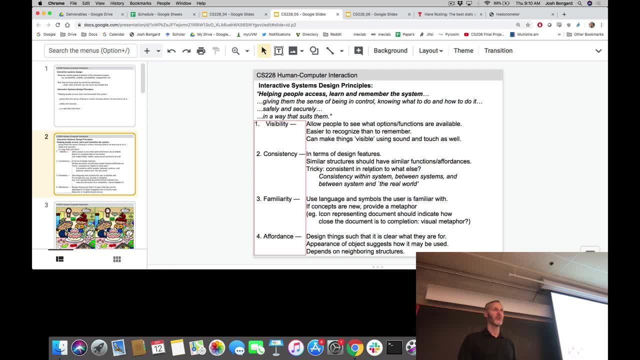 the splash page. I don't like this app. exit- I want out get rid of it. where do exit? I want out get rid of it. where do exit? I want out get rid of it. where do I go? the close button right and maybe I go the close button right and maybe. 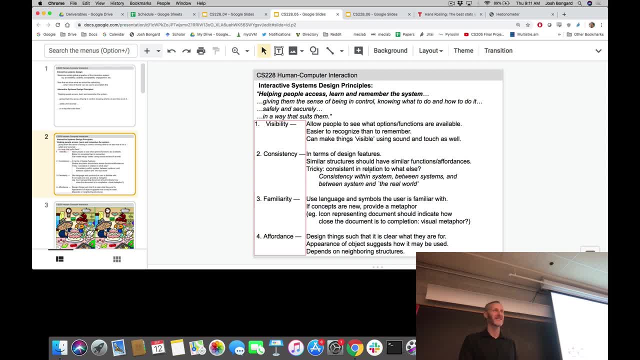 I go the close button right and maybe that's on my phone itself. but usually that's on my phone itself. but usually that's on my phone itself. but usually the app has some sort of exit pathway. the app has some sort of exit pathway. the app has some sort of exit pathway. where is the exit pathway to the right? 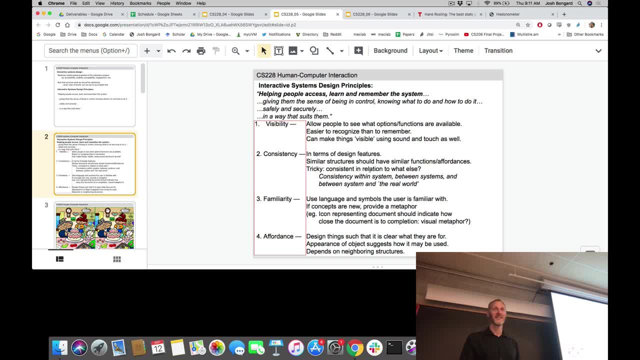 where is the exit pathway to the right? where is the exit pathway to the right exactly? could be more specific. could be exactly. could be more specific. could be exactly. could be more specific. could be: usually bottom center or upper right. usually bottom center or upper right. usually bottom center or upper right. right seem kind of arbitrary in the old 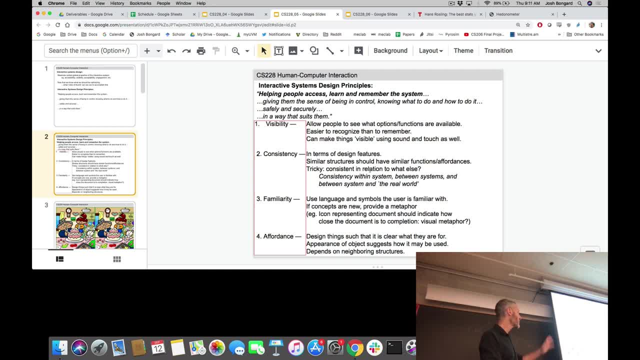 right seem kind of arbitrary in the old right, seem kind of arbitrary in the old days as you could probably imagine it, days as you could probably imagine it, days as you could probably imagine. it was everywhere for different apps, so was everywhere for different apps, so was everywhere for different apps. so there's been this implicit convergence. 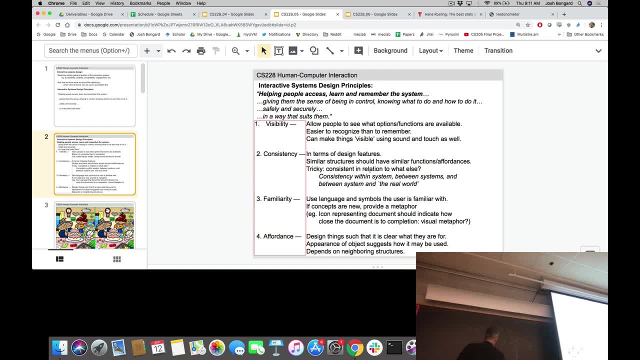 there's been this implicit convergence. there's been this implicit convergence on certain consistency, one of the most on certain consistency, one of the most on certain consistency. one of the most recent ones is this icon: what does it recent ones? is this icon? what does it recent ones? is this icon? what does it mean? menu more right. so these lines. 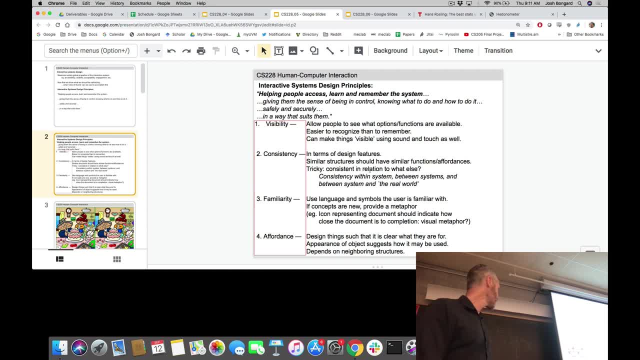 mean menu more right. so these lines mean menu more right. so these lines represent menu items. if you think about represent menu items, if you think about represent menu items, if you think about, it's a very abstract ideogram, right? but it's a very abstract ideogram, right? but 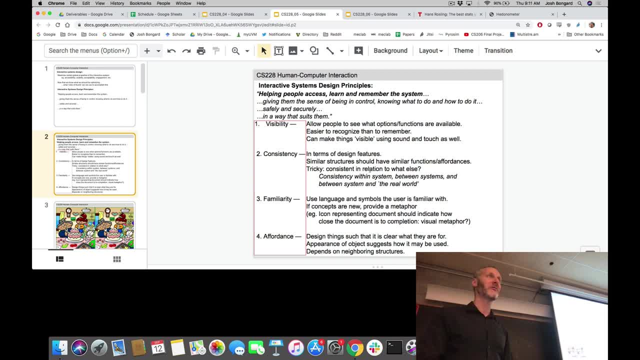 it's a very abstract ideogram, right, but anybody's used technology enough, we all. anybody's used technology enough, we all. anybody's used technology enough. we all know about cascading functions and menu, know about cascading functions and menu, know about cascading functions and menu, hierarchies and so on. it's all been. 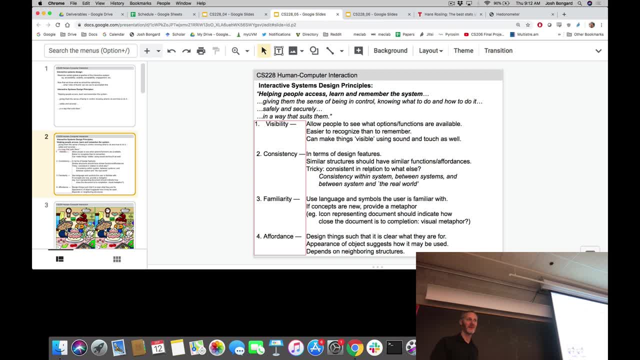 hierarchies and so on. it's all been hierarchies and so on. it's all been condensed down in just the last few, condensed down in just the last few, condensed down in just the last few years. to this right, so the app is going. years to this right, so the app is going. 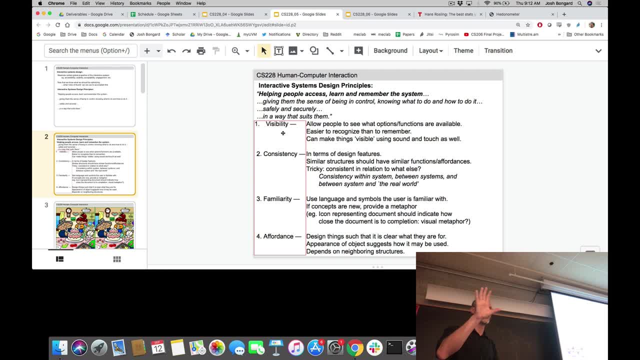 years to this right. so the app is going to visibly show me just the stuff I need. to visibly show me just the stuff I need to visibly show me just the stuff I need. for now on the login page, it's just how. for now on the login page, it's just how. 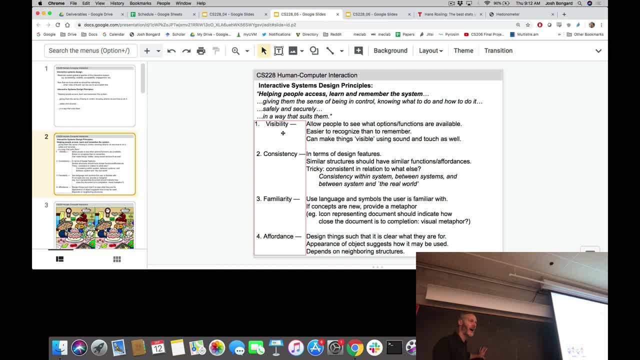 for now on the login page. it's just: how do I log in? it's gonna hide everything. do I log in? it's gonna hide everything. do I log in? it's gonna hide everything else, and usually it's gonna hide all else, and usually it's gonna hide all. 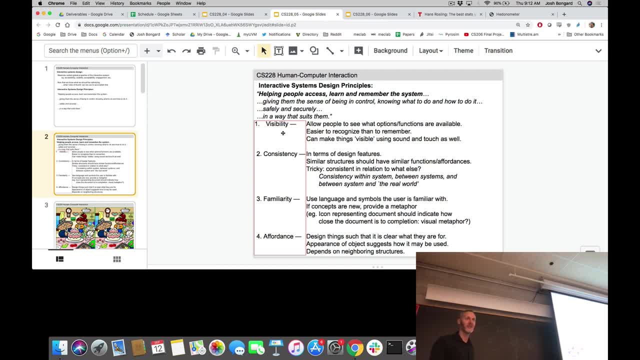 else, and usually it's gonna hide all that other stuff under quote-unquote, that other stuff under quote-unquote, that other stuff under quote-unquote. underneath this thing. what are some underneath this thing? what are some underneath this thing? what are some other examples of consistencies across? 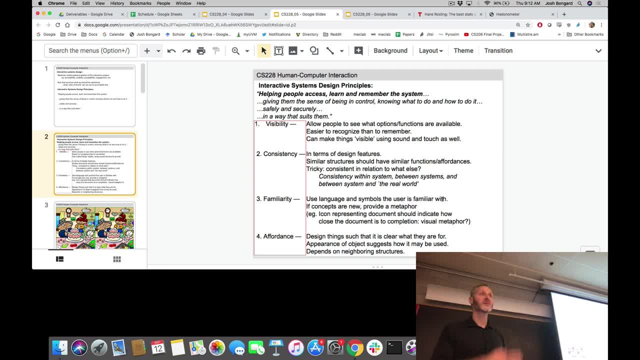 other examples of consistencies across other examples of consistencies across software systems across software systems. software systems across software systems, software systems across software systems. and the physical world- what are some? and the physical world- what are some? and the physical world- what are some other aspects of apps or software web? 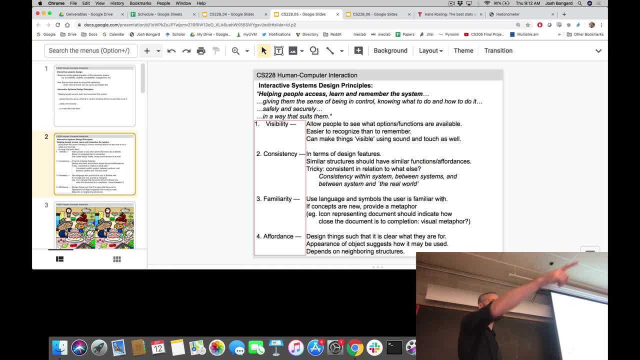 other aspects of apps or software web, other aspects of apps or software web pages. that sort of build on our pages, that sort of build on our pages, that sort of build on our expectations from the real world. yes, expectations from the real world. yes, expectations from the real world, yes. 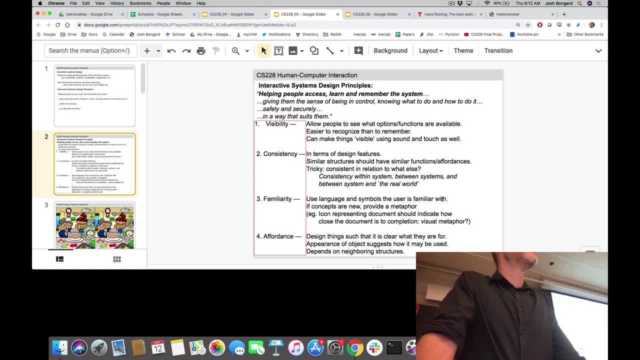 yes, yes, I absolutely right so most websites. I absolutely right so, most websites. I absolutely right. so most websites today. they're a lot, much larger text today. they're a lot, much larger text today. they're a lot, much larger text, more white space right than it used to. 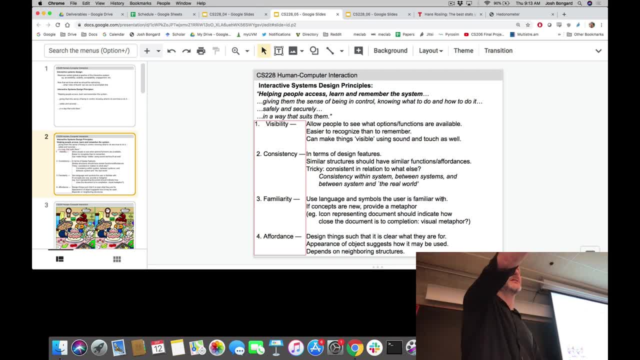 more white space right than it used to. more white space right than it used to be. we're all converging to this sort of be. we're all converging to this sort of be. we're all converging to this sort of implicit consistency scrolling right. implicit consistency: scrolling right. 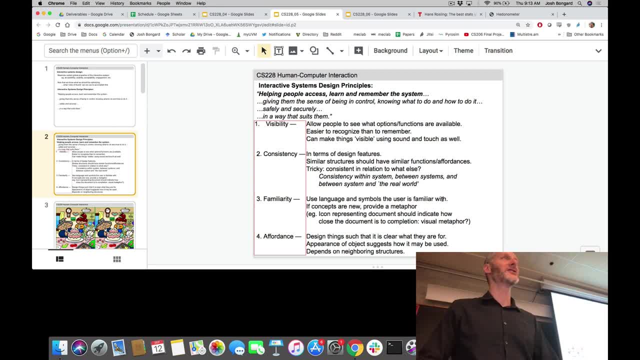 implicit consistency, scrolling right exactly. I don't need to crowd all the exactly. I don't need to crowd all the exactly. I don't need to crowd all the information on to a page and make sure information on to a page and make sure information on to a page and make sure that you can see it all on the splash. 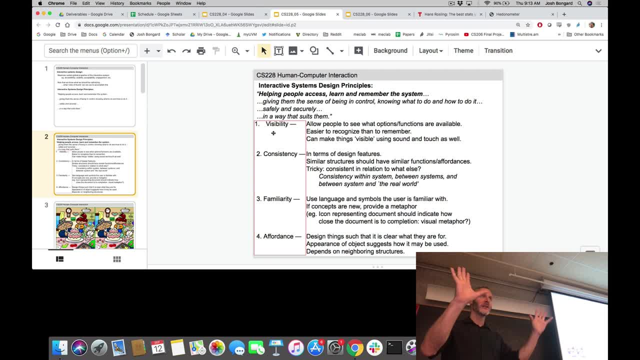 that you can see it all on the splash, that you can see it all on the splash page. most people now expect a little bit page. most people now expect a little bit page. most people now expect a little bit of text, a lot of white space and, if I 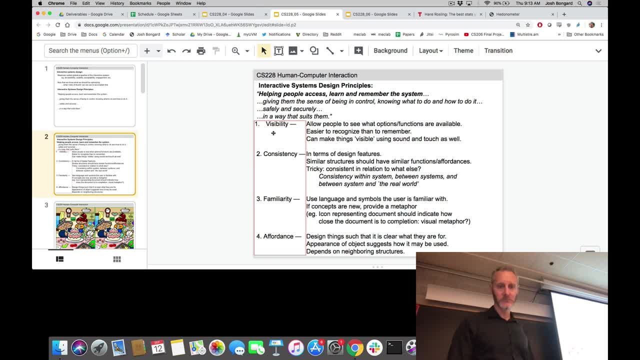 of text a lot of white space, and if I of text a lot of white space. and if I want more, I'll, I'll go scrolling. okay, want more? I'll, I'll go scrolling. okay, want more? I'll, I'll go scrolling. okay, let's come back to you. have a comment? 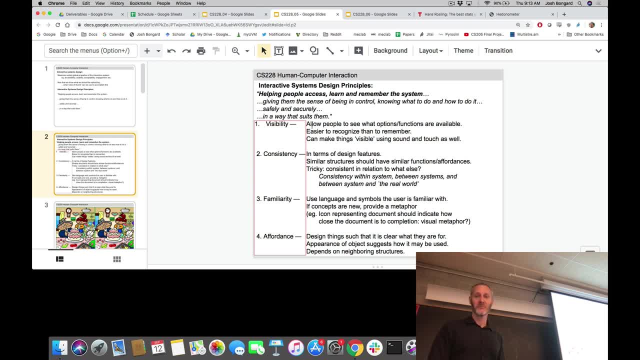 let's come back to you have a comment. let's come back to you, have a comment. what's rubber banding that one? I don't. what's rubber banding that one? I don't. what's rubber banding that one? I don't know. yep, that it does what that it. 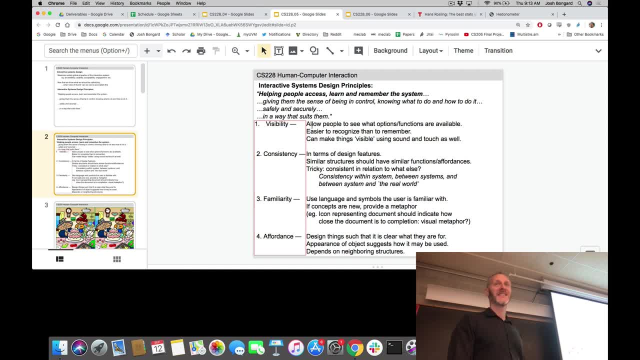 know, yep, that it does what. that it know, yep, that it does what. that it bounces around. oh, that it tells you bounces around. oh, that it tells you bounces around. oh, that it tells you it's the end. oh, I rubber band, I get it. it's the end. oh, I rubber band, I get it. it's the end. oh, I rubber band, I get it right. exactly it doesn't crash at the right. exactly it doesn't crash at the right. exactly it doesn't crash at the end. it sort of bounces around a little. 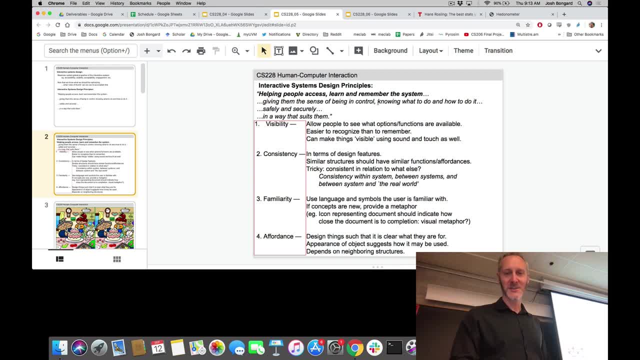 end. it sort of bounces around a little end. it sort of bounces around a little bit. that's a good, that's a good one bit, that's a good, that's a good one bit, that's a good, that's a good one right, kind of subtle, very nice, very nice. 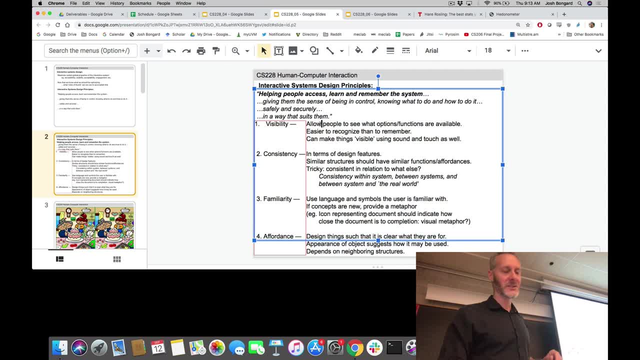 right kind of subtle, very nice, very nice. right kind of subtle, very nice, very nice. okay, let's come back. I forgot to. okay, let's come back. I forgot to. okay, let's come back. I forgot to mention something about visibility. so we mention something about visibility, so we 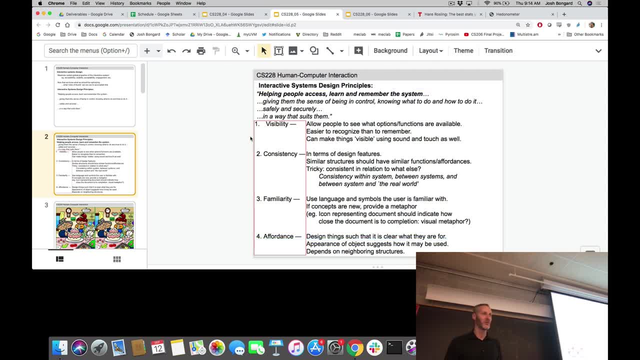 mention something about visibility. so we want to make our system visible, but it want to make our system visible, but it want to make our system visible, but it understanding of the human visual system, understanding of the human visual system, understanding of the human visual system. the human visual system is wonderful. 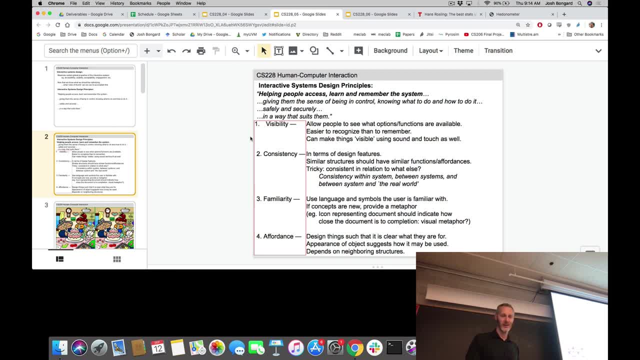 the human visual system is wonderful. the human visual system is wonderful. works well for some things, not so well. works well for some things, not so well. works well for some things, not so well for other things. so let's play the photo for other things. so let's play the photo. 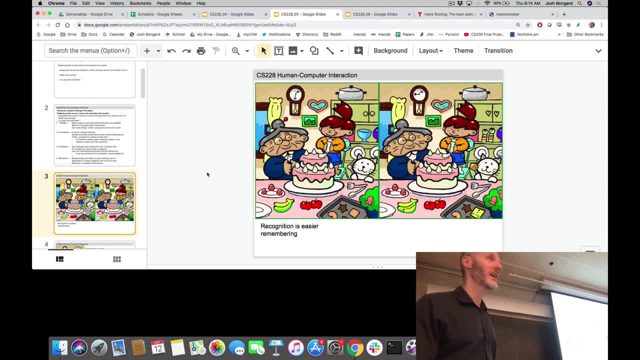 for other things. so let's play the photo game for a moment to drive home this game for a moment to drive home this game for a moment to drive home this point. I apologize for those in the back point. I apologize for those in the back point, I apologize for those in the back. how many differences between these two. 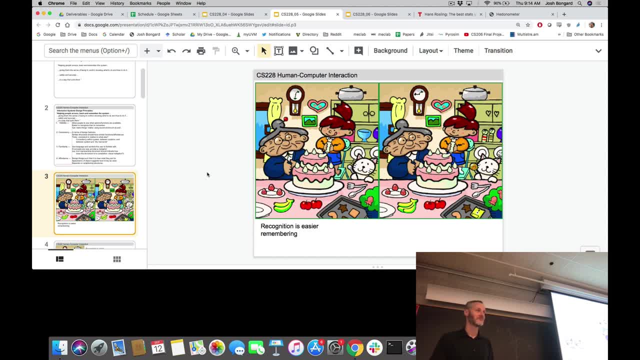 how many differences between these two, how many differences between these two cartoon images? okay, hold on to your number for a moment. okay, hold on to your number for a moment. okay, hold on to your number for a moment. so, in this tongue-in-cheek example, I am. 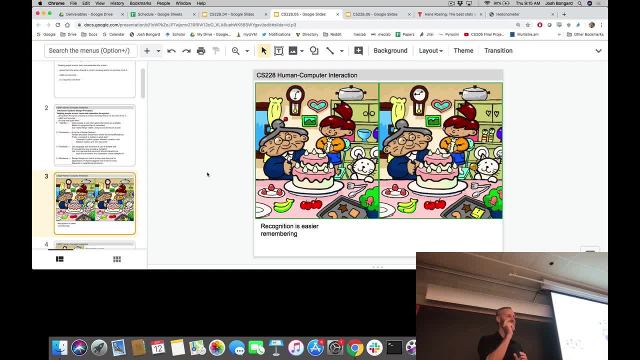 so in this tongue-in-cheek example I am. so in this tongue-in-cheek example, I am trying to communicate some information, trying to communicate some information, trying to communicate some information to you, I'm trying to make specific to you. I'm trying to make specific. 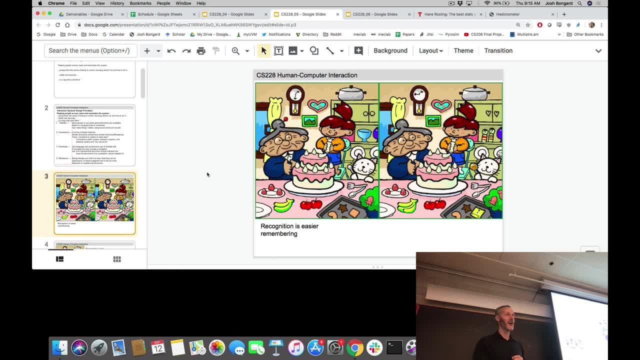 to you. I'm trying to make specific details visible, and those details are details visible and those details are details visible. and those details are the differences between the two images, the differences between the two images, the differences between the two images. the whole point of this game is they're. 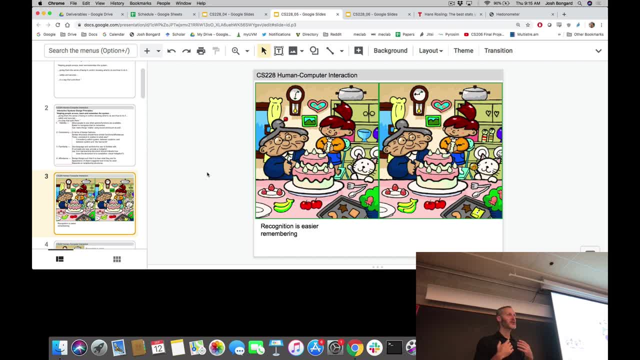 the whole point of this game is they're the whole point of this game is they're not. it's not made easy for you, let's not. it's not made easy for you, let's not. it's not made easy for you, let's assume I want to make that information. 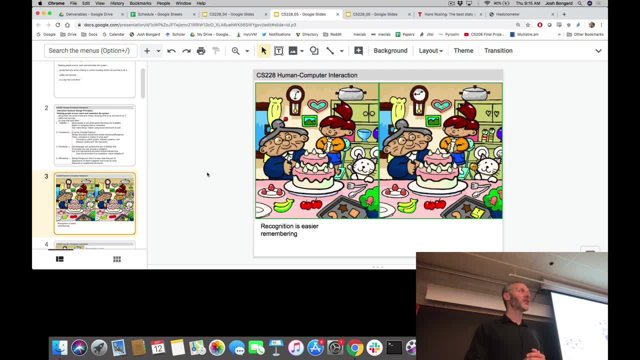 assume I want to make that information, assume I want to make that information as obvious to you as possible. I could, as obvious to you as possible. I could. as obvious to you as possible, I could add some additional ink I could draw. add some additional ink I could draw. 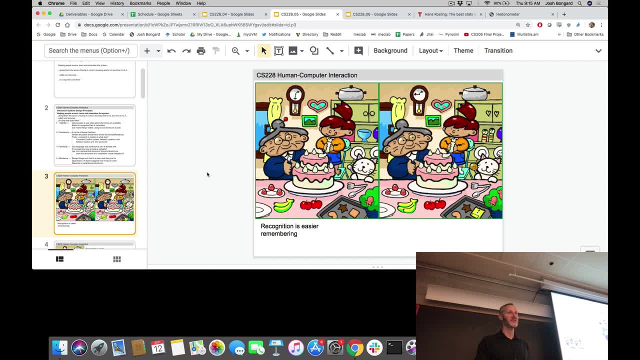 add some additional ink. I could draw circles around points in the images, circles around points in the images, circles around points in the images where there are differences. but I'm where there are differences, but I'm where there are differences, but I'm adding ink. remember our discussion from: 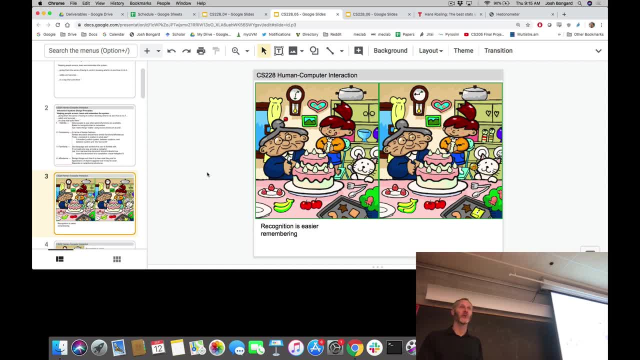 adding ink. remember our discussion from adding ink. remember our discussion from Tuesday about trying to maximize the Tuesday, about trying to maximize the Tuesday, about trying to maximize the data to ink ratio. I want to communicate data to ink ratio. I want to communicate data to ink ratio. I want to communicate as much information to you as possible. I. 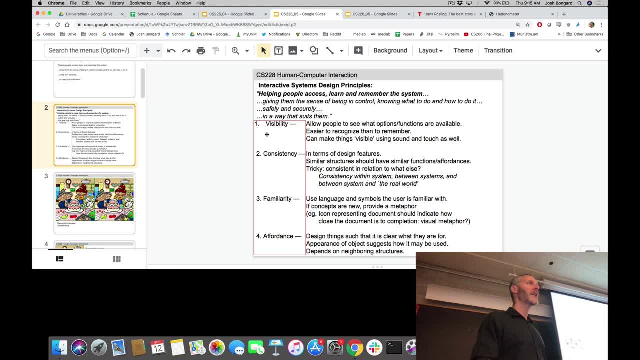 as much information to you as possible. I as much information to you as possible. I want to make various options or things, want to make various options or things, want to make various options or things visible. but I don't want to do so by visible, but I don't want to do so by. 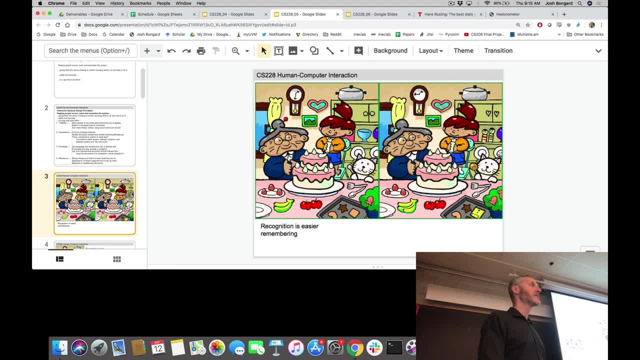 visible, but I don't want to do so by splashing too much ink or too much. splashing too much ink or too much. splashing too much ink or too much detail on to the screen. so how could I detail on to the screen? so how could I? 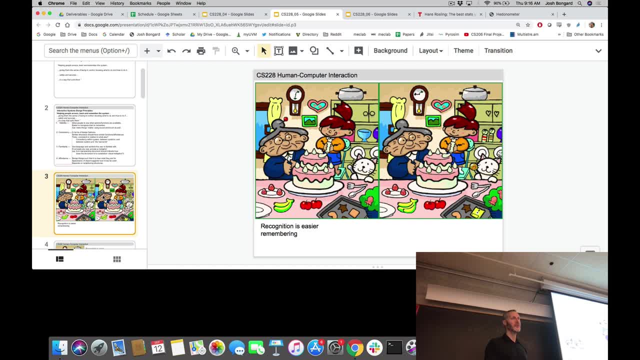 detail on to the screen. so how could I go about making that those items more? go about making that those items more, go about making that those items more obvious without having to add any obvious, without having to add any obvious, without having to add any additional ink? absolutely so, instead of 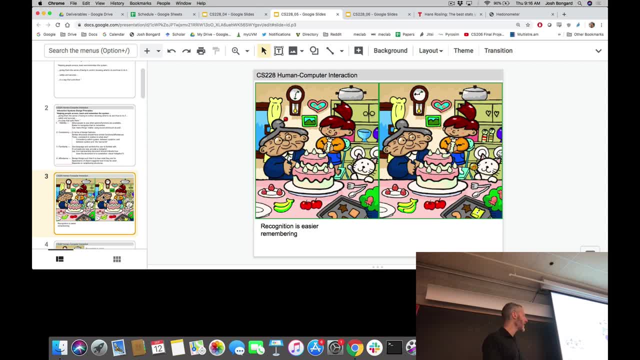 additional ink. absolutely so, instead of additional ink: absolutely so, instead of adding I we could subtract right. this is adding I, we could subtract right. this is adding I, we could subtract right. this is again a great unspoken design principle. again a great unspoken design principle. again a great unspoken design principle. well, design in general: right, less is. 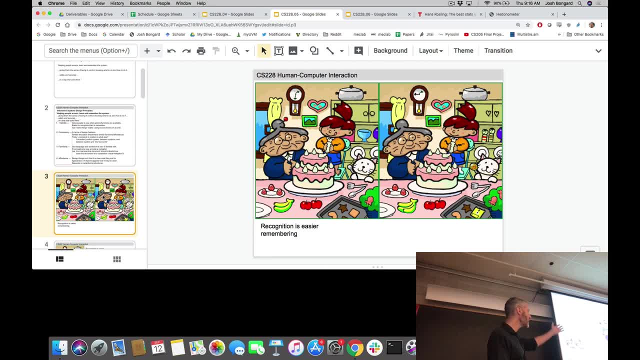 well. design in general: right. less is well. design in general, right. less is more, more more room, room, room, room, room. rather than add for most people. their rather than add for most people, their rather than add for most people. their immediate instinct is draw a circle. immediate instinct is draw a circle. 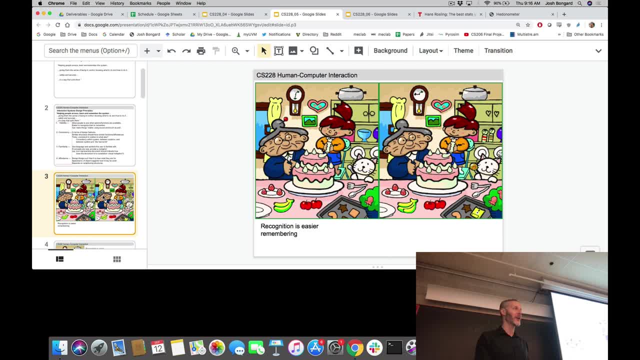 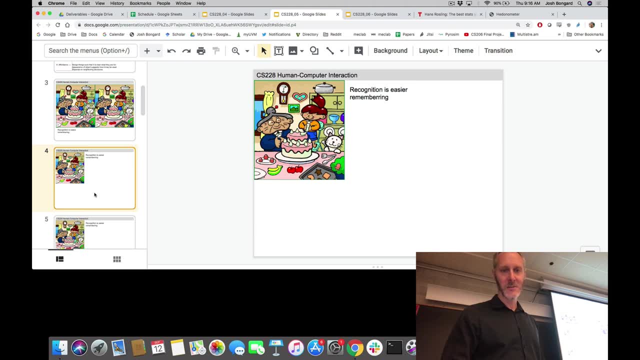 immediate instinct is: draw a circle around. add right, put arrows. put flashing around. add right, put arrows, put flashing around. add right, put arrows. put flashing arrows. add more instead of subtract arrows. add more instead of subtract arrows. add more instead of subtract. there's other ways we can do this same. 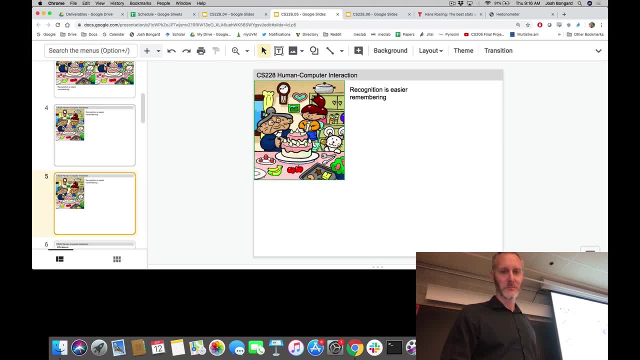 there's other ways we can do this same. there's other ways we can do this same. image how many differences are there. I image how many differences are there. I image how many differences are there. I hear 12, 14, hear 12, 14, 14. 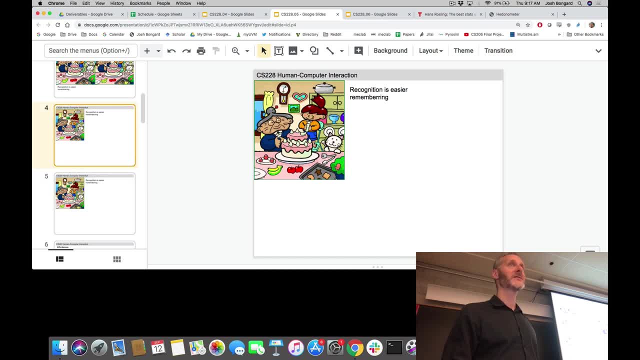 hear 12, 14, 14. when I created these slides and was writing, when I created these slides and was writing, when I created these slides and was writing the text, I made it. I made a. the text. I made it. I made a. the text, I made it. I made a mistake which I didn't see until I then made. 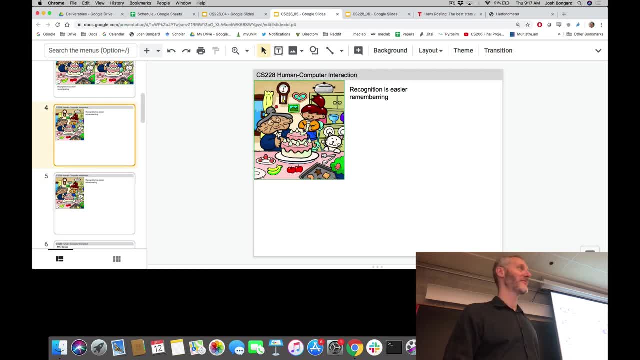 mistake which I didn't see until I then made mistake which I didn't see until I then made these two slides. there's actually these two slides. there's actually these two slides. there's actually two mistakes in the text. did anyone notice two mistakes in the text? did anyone notice? 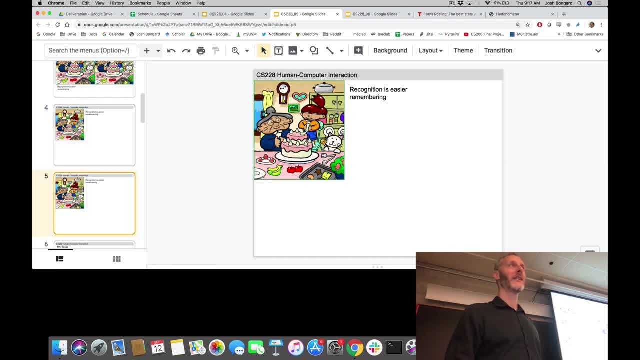 two mistakes in the text. did anyone notice that I misspelled? remembering that I misspelled, remembering that I misspelled, remembering that's one, that's one, that's one. then right, which you don't see because. then right, which you don't see because. 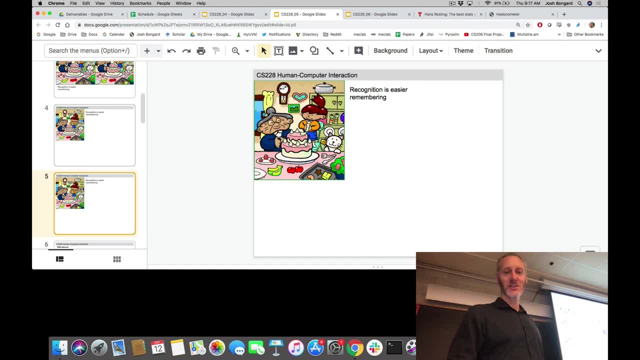 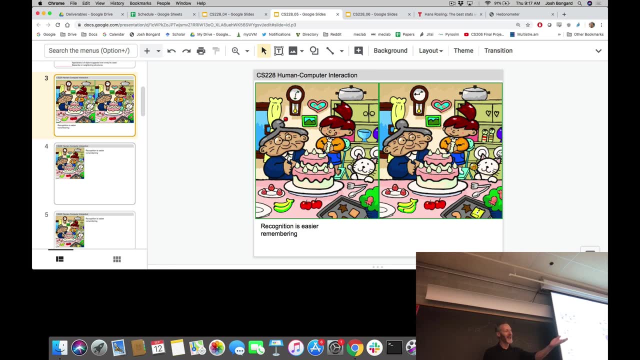 then right, which you don't see because it's the same mistake in both slides. so we can, we can try and present, we can. we can try and present, we can. we can try and present information in different ways. we can add information in different ways we can add. 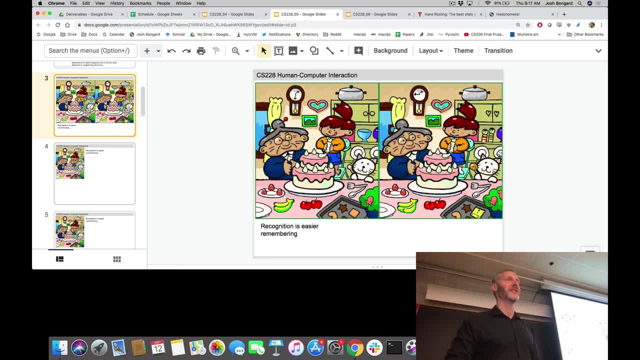 information in different ways. we can add. we could subtract. we could show the. we could subtract. we could show the. we could subtract. we could show the information in a different way and this information in a different way and this information in a different way. and this way is exploiting a particular mechanism. 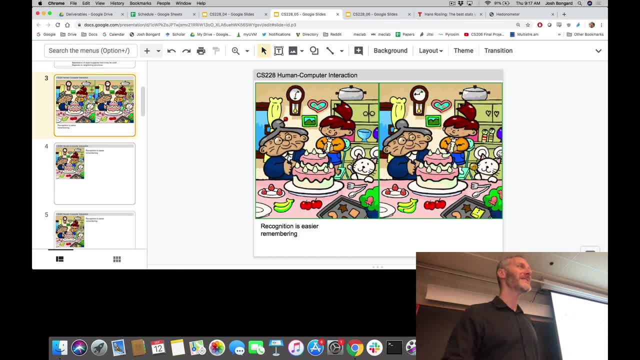 way is exploiting a particular mechanism. way is exploiting a particular mechanism of the human visual system that makes it of the human visual system, that makes it of the human visual system, that makes it easier to recognize the difference, easier to recognize the difference, easier to recognize the difference in details here. what is that detail of the? 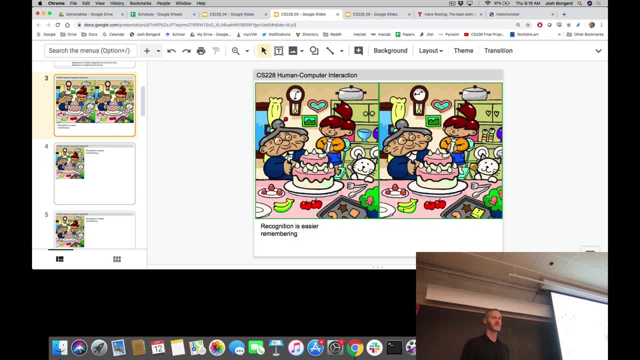 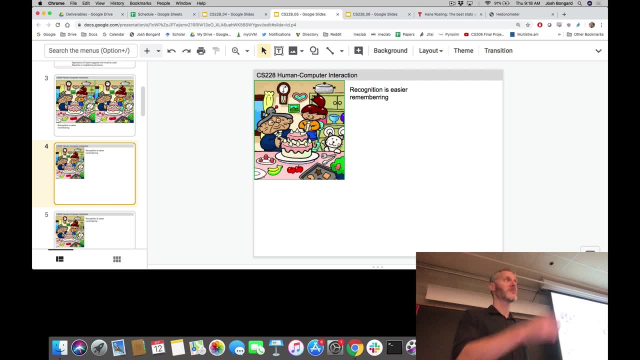 in details here. what is that detail of the in details here? what is that detail of the human visual system? that we're human visual system, that we're human visual system, that we're exploiting persistence of vision, exploiting persistence of vision, exploiting persistence of vision? possibly can we describe it another way. 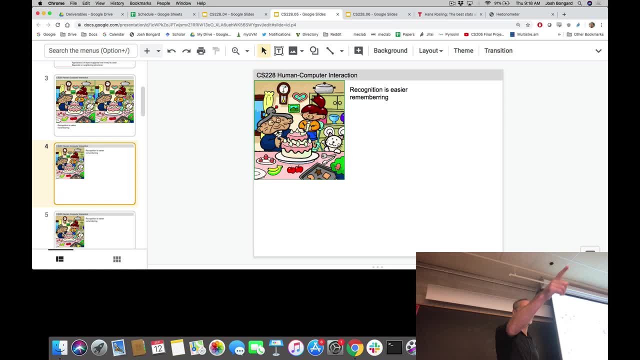 maybe, maybe motion right, maybe motion right. So, for very good reason, the primate visual system immediately attends to movement right or change. You can't help it If I were to leave this up for a few minutes, and I promise I won't. 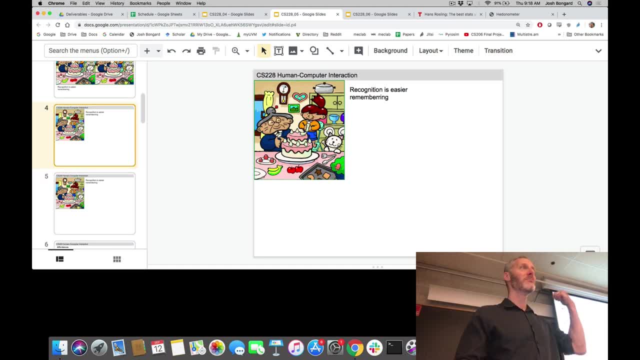 it's very hard to look away or pay attention to my voice. The movement inside the cartoon keeps bringing your eyes back. Your eyes saccade, or they move so that the exact point where the motion was detected lands in the center of your visual field. 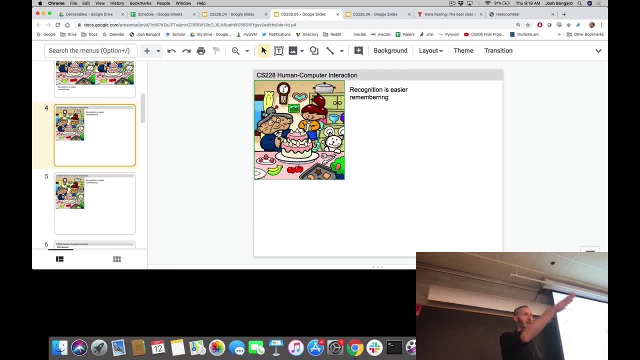 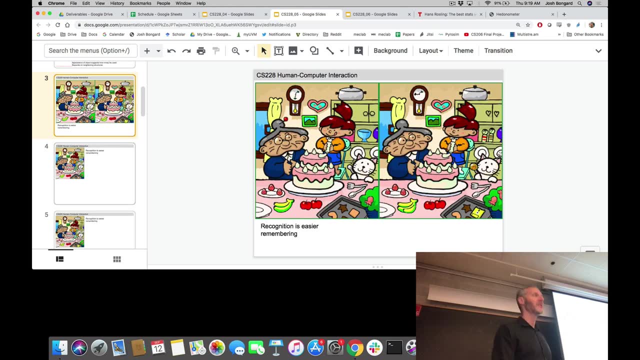 and you're seeing lots of those little localized pieces of movement, so your eyes are rapidly saccading around the image. So, instead of you having to actively search, instead of saccading on this strawberry and then jumping to this strawberry and making sure that there is actually a strawberry there and jumping back, 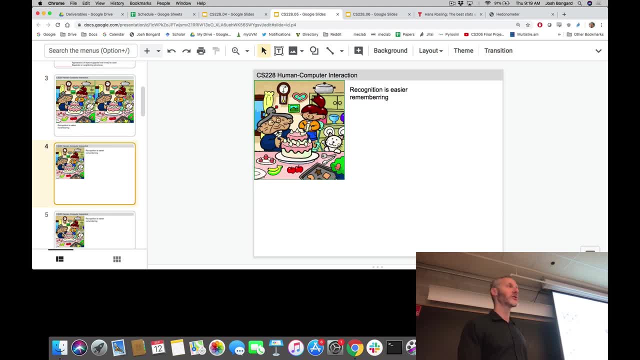 you're forcing yourself to do it. When we introduce the motion, the motion is doing it to your visual system, right, And that can either be annoying if it's an ad where there's someone dancing on the side of some web page that you're trying to read, or we could try and again. 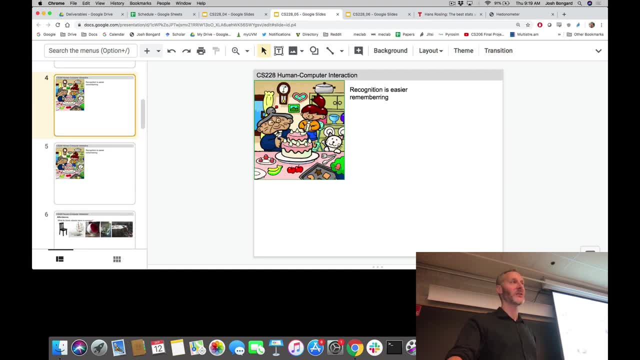 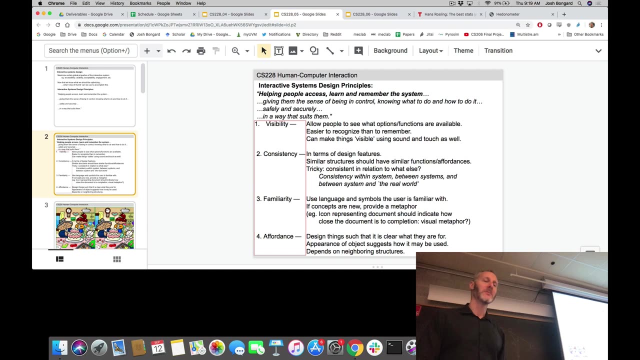 exploit it, because the user is trying to do something which is find these differences, and we can make it easier on them by presenting the information in a different way. Okay, so related consistency is obviously familiar. Familiarity- we've kind of already mentioned this one. 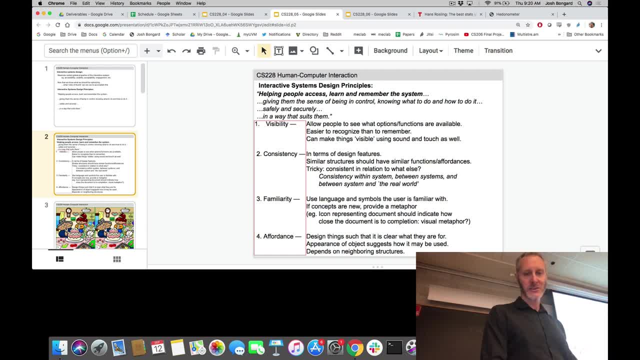 We want to try and use as much as possible, things that the user is familiar with and in cases where things are not familiar, we're trying to introduce some new concept or some new type of interaction with the system. We want to try and use a quote-unquote metaphor. 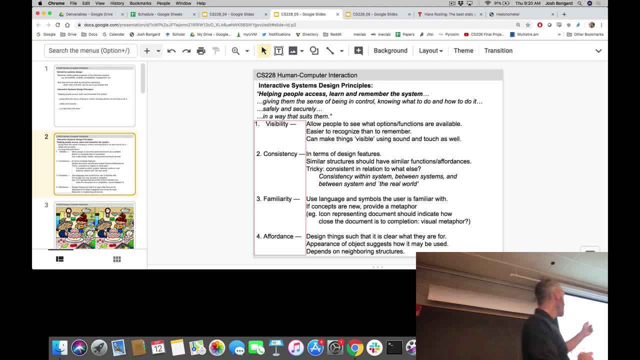 We've already talked about visual metaphors a little bit. Imagine, and this one's kind of dated now, I guess. imagine we have an icon on the desktop and that icon points to a, a form, and you're supposed to be filling out the form. 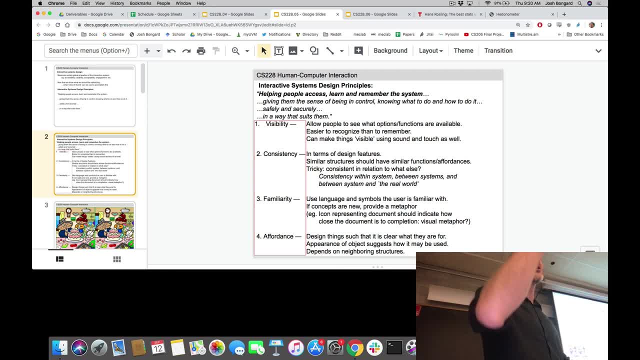 It's a long, complex form, so you fill out part of the form, close it down. there's another icon on your desktop, some other form you need to fill out. You're filling these out. We'd like to help the user step back. look at their desktop. 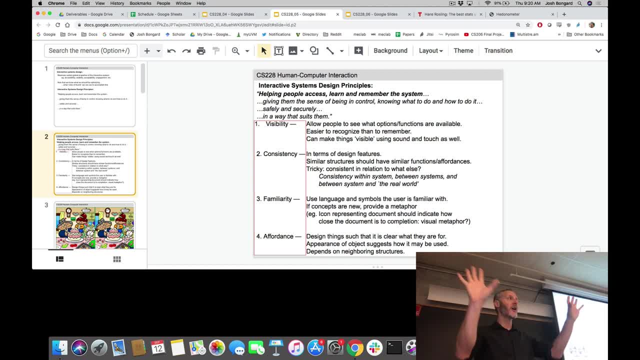 all the forms and get an overview for how far they are in filling out the various forms. How would you draw the icons? What might be a metaphor for filling up a form with, let's say, a word We could fade out? 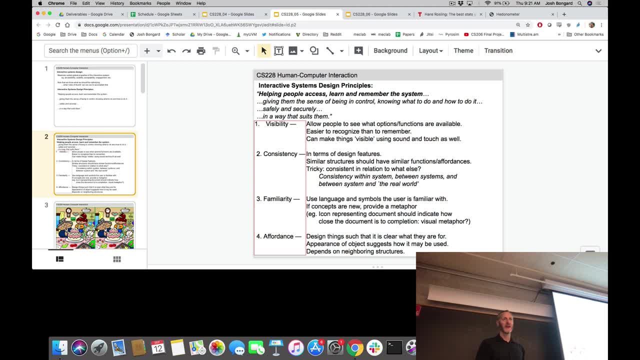 We could fade out the part that's not. and when you first described this, you said filling up and you moved your hand from the bottom to the top. You're communicating a particular metaphor. What was it? Yeah, Yeah, Yeah. 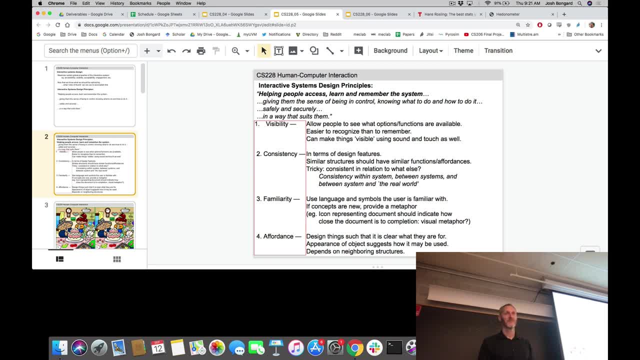 I don't know if that's the right way to do it. I don't know if that's the right way to do it. I don't know if that's the right way to do it, Absolutely right. So if you fill up a bucket with water or you fill up a form, 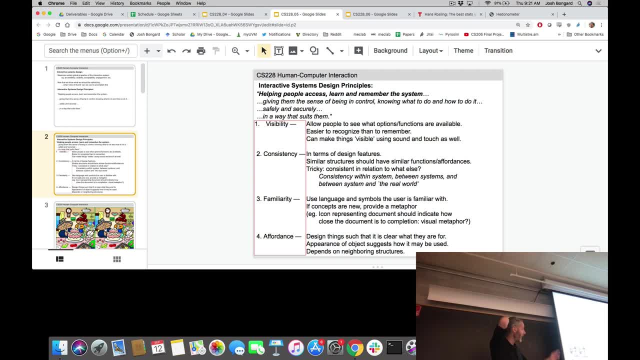 with data. if you pay attention to the metaphor in the language there, you're filling it up right, So we could use that and turn that into a visual metaphor to communicate that information, Whether you'd want to do so or not, I don't know. 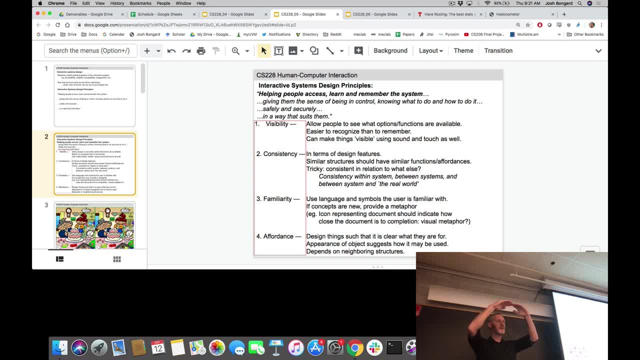 but that's the sort of idea, right? It would be strange. It would be strange if you had sort of an indicator where you're filling in things from the top down. It might be confusing. However, when you fill out a form. 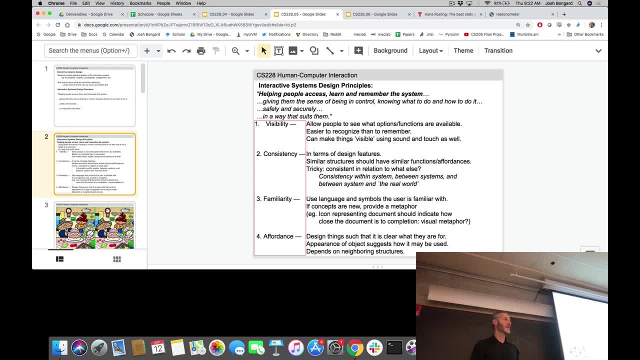 you're often filling data from the top of the form down. It's like the example from the beginning of the course of the series of sign and innovation of first floor, fourth floor, or first floor, fourth floor. How about some other examples of visual metaphors? 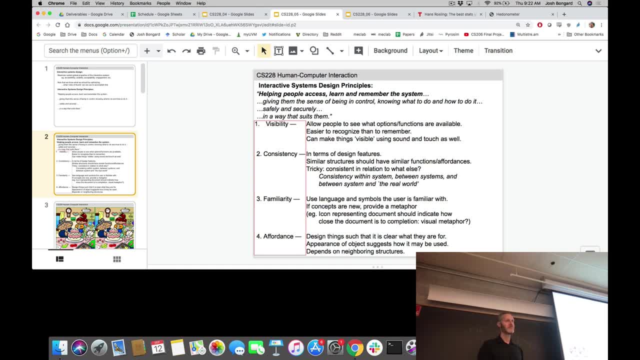 How might you try and communicate something that's unfamiliar With, something that, through a metaphor, becomes familiar? Yeah, I was thinking one of the mentors is like they'll have a little like sound background, like sound is coming out of it. 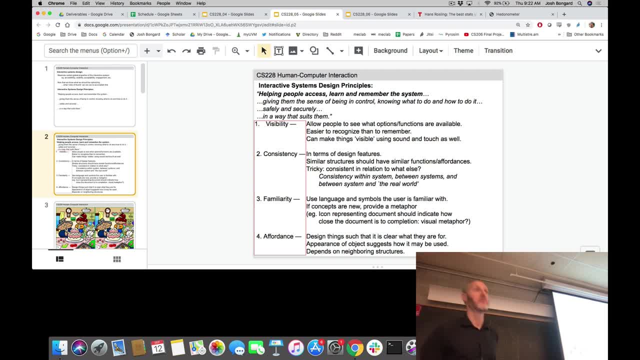 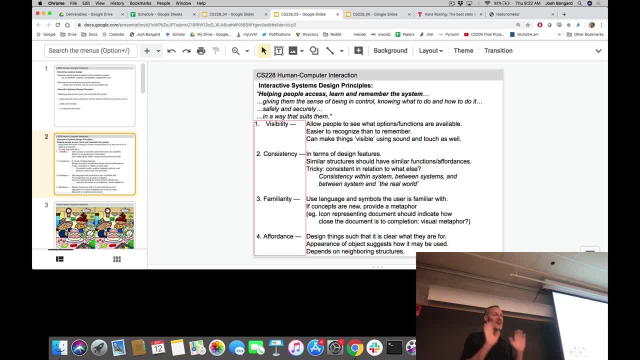 Right, Right, Right, Right, Right, Right. The trash icon. Okay, There's an oldie but a goodie. Absolutely Tricky to get the trash icon right because the when you throw something in a trash bin, you can, in theory, take it back out again. 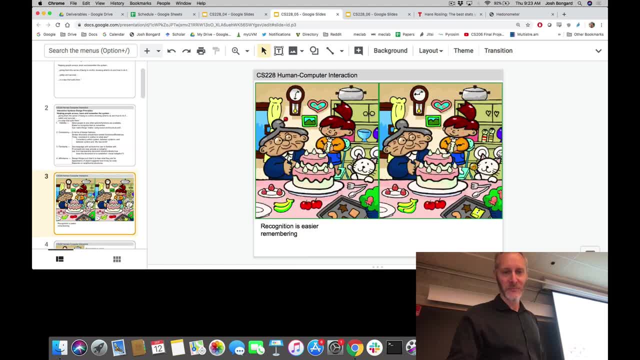 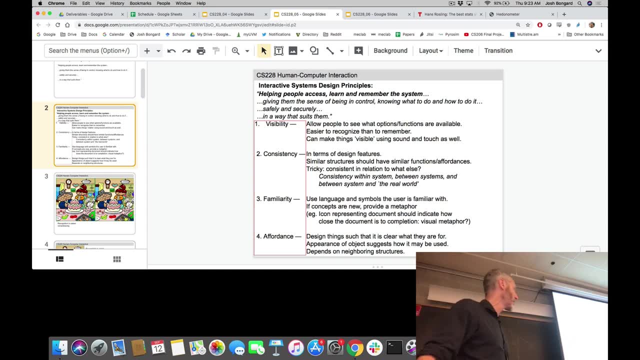 right tricky, okay. last one here again related to familiarity. we're going to talk about this idea a fair bit when we get to the psychology. part of the course is the idea of affordances, and this is an idea that comes from psychology. an affordance is an advertisement that an object projects. it's the object is. 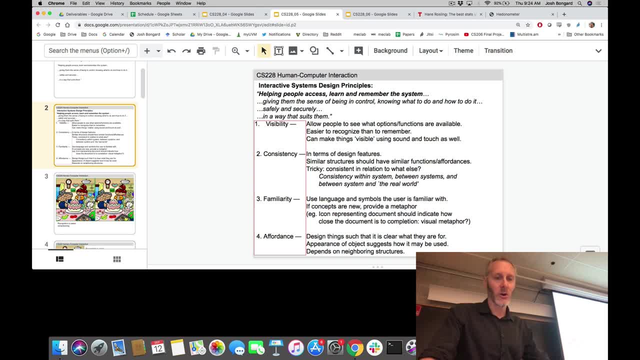 trying to say something to you. so often in HCI design we're designing icons, or the trash icon or the rubber band at the bottom of the screen. we're trying to present something that's communicating or advertising. an image, a little avatar that's looking into your eyes, is projecting a particular affordance which 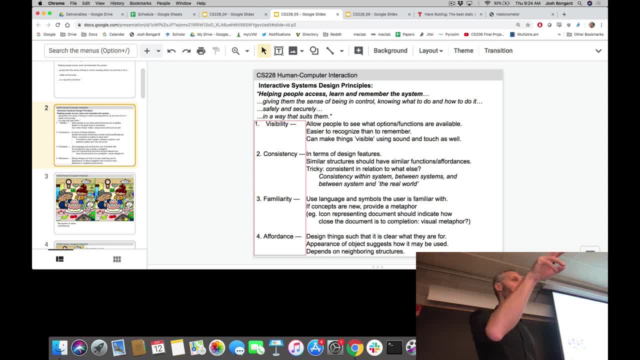 is. I'm paying attention to you and I'm either waiting for you to do something or I'm about to do something and I want you to respond right. so it doesn't matter whether it's an owl or an avatar or a paper clip, it doesn't really matter. 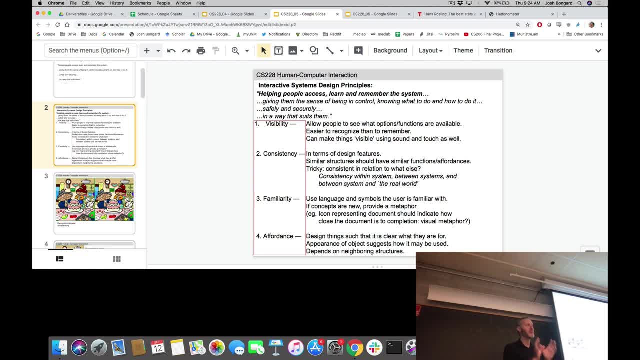 about the shape or form of the thing. it's how the thing behaves. to project or advertise that, uh affordance. so again, in visual design there's often. your first instinct is often to spend a lot of time on the physical form of the object or the icon or the avatar. oftentimes it's not the form itself that's important. 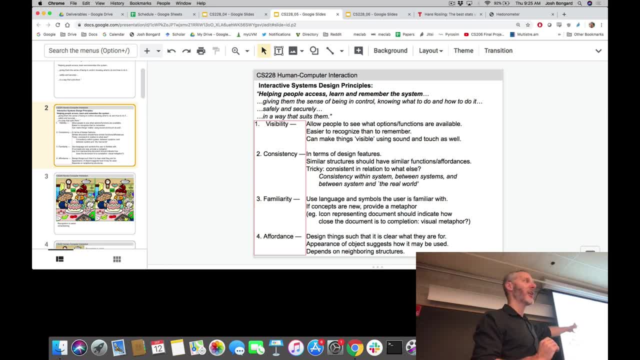 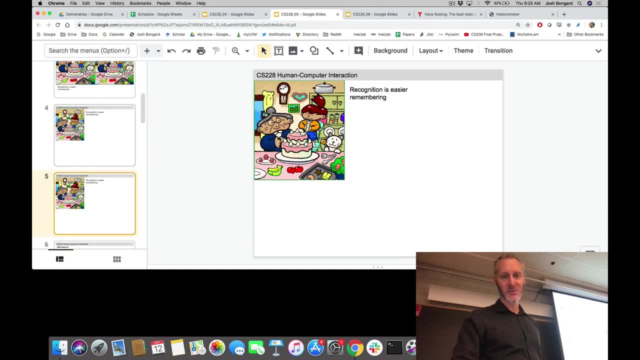 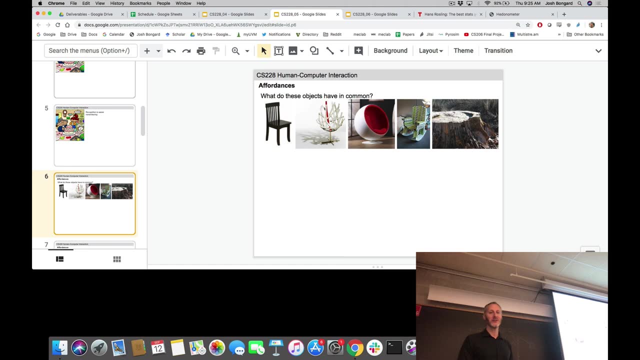 it's how it moves or behaves and matches our expectations that we bring from the physical or social world. so let's have a look at a couple of affordances. we'll start with non-technical ones. here's five images. clearly they all have very different forms. what do they have in common? 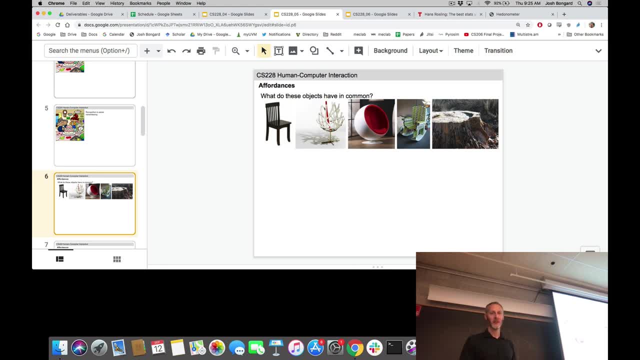 they're all seats right should take you. it's effortless right. we can view that at the beginning. I picked these particular items because they highlight something interesting, not from so much from HCI but the history of computer vision. so computer vision in just the last few years has gotten very. 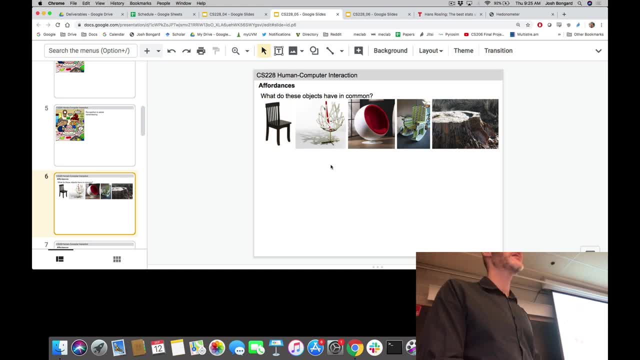 good due to millions and millions of images and some advances in neural networks and so on. but there was also a conceptual hurdle in computer vision for a long time, which is: how do we teach a computer to recognize chairs? well, obviously. obviously, chairs have four legs and a flat area to sit on and usually a back. 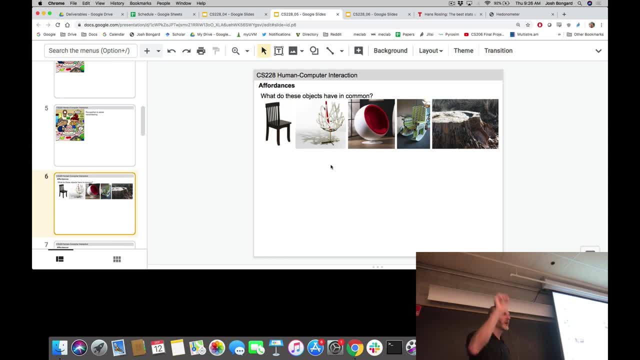 so let's write some code that takes an image and says if there are four long things pointing down and a flat thing attached to the top of those four things, it's a chair. otherwise it's not works great for this example, not so much for this one. so we add another if, then clause inside if it doesn't have four. 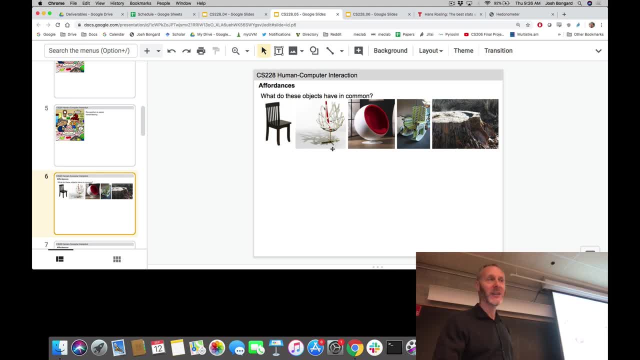 legs but it but it has a Little vertical shaft and then four prongs coming out vertically. then also it's a chair. right, you can kind of see where this is going. computer vision had a hard time for a long time getting going because there was a misunderstanding about how humans visually recognize. 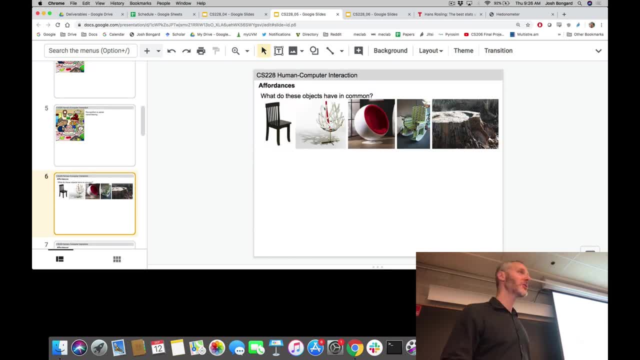 and you're thinking about affordances or chairs. if I were to ask you what a chair is, you might actually start to describe it geometrically. it's got a platforms fortis. are chair requires a- now you'll see, and mizu, that they took at, and a flat seat for sitting on, and so on. and you're giving me the geometric. 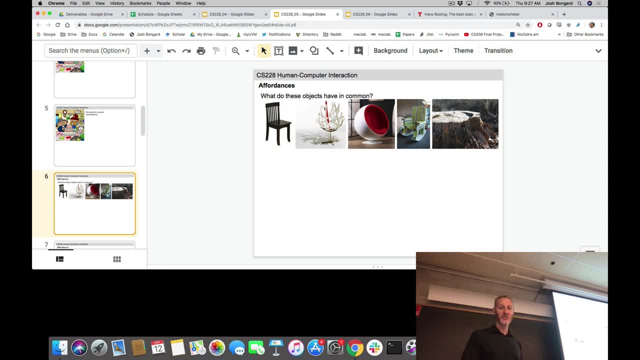 description, but that's actually not what we're doing. you're starting with a geometry, perhaps, but you're projecting yourself, your virtual self, into the image and asking yourself: can I sit in this chair, or can I sit in or on this object? or we can turn it around from an affordance point of view. the object is: 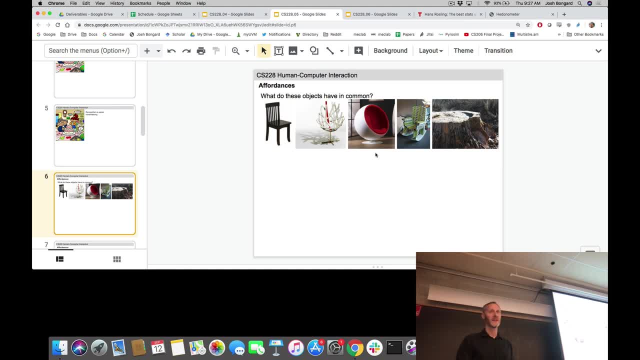 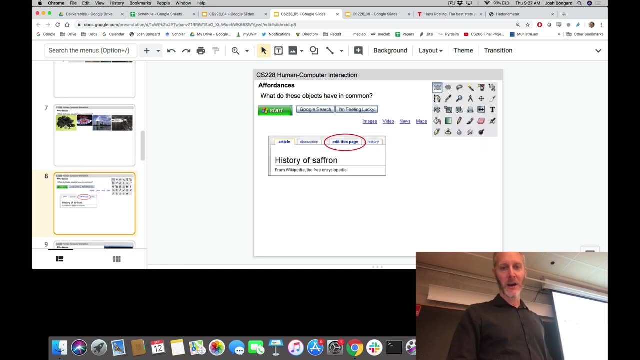 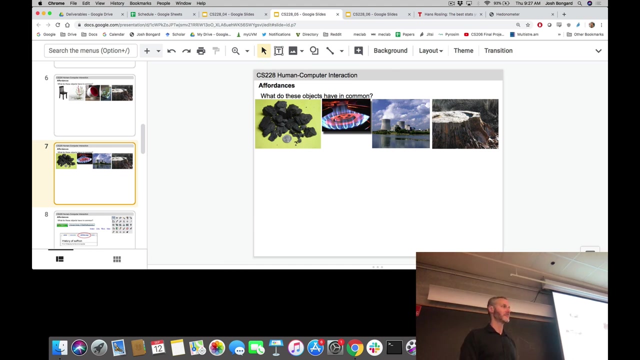 projecting something which is I am suitable. so one way to think about affordances as ad adverbs right, they afford or they provide a particular action which, in this case, is sitting. how about these four images? what's the affordance here? they're fuel, right, they provide heat, warmth, comfort, energy to us, right, and obviously have kept one. 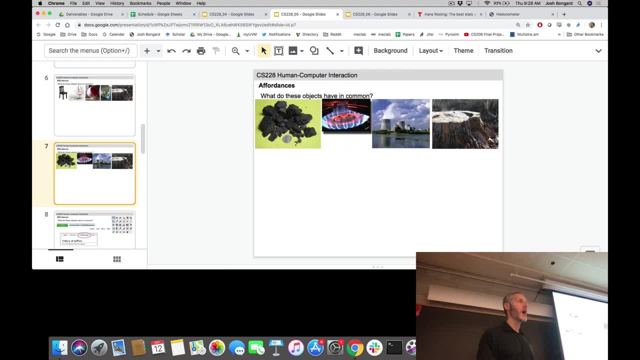 of the images the same. no one object has one affordance. the type of affordance that it projects is a function of context. what else is going on in this case? literally around the image of the tree, stump right, we can have a little virtual owl that's looking out at you on the screen and that's okay. but there's 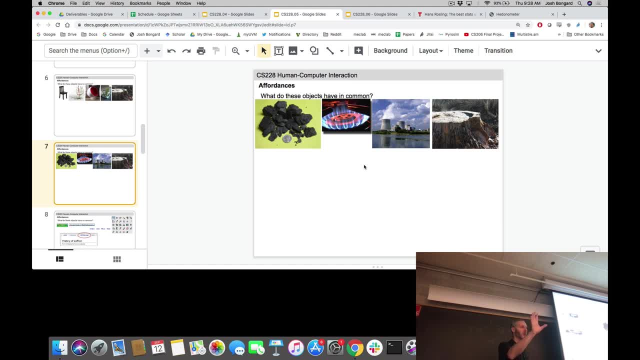 several affordances there. possibly the owl is trying to project the affordance. teach me or show me. it's waiting for something from you or it's projecting the affordance. I'm about to show you something and teach you something. how do you, as the observer, disambiguate between those two affordances? hopefully there. 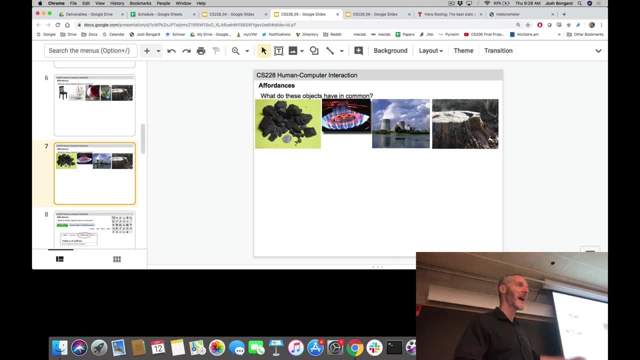 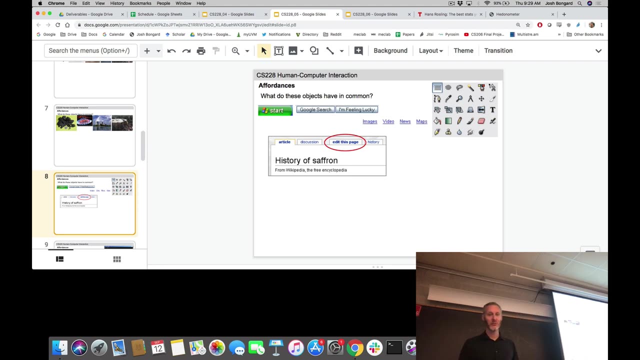 are other things going on on the screen, or things that just happened on the screen, that make it immediately clear what the owl is about to do or what it wants. okay, so now let's have a look at some more HCI related examples. what's the affordance of the virtual object that I've circled in red? it's clickable right. 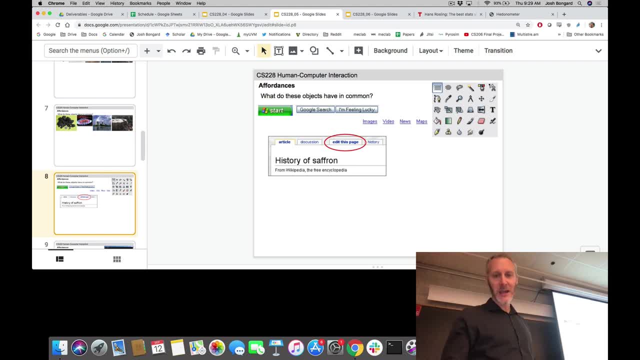 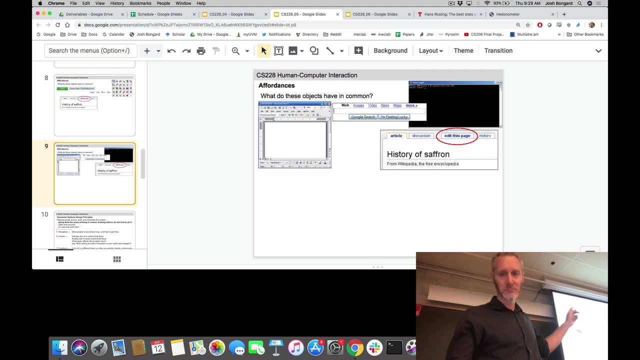 that's it. that's the adverb I was looking for. let's play the same game. I'm going to keep the same. I'm going to keep one of these objects the same. what is the importance? now you can enter text here, right, some of them are. 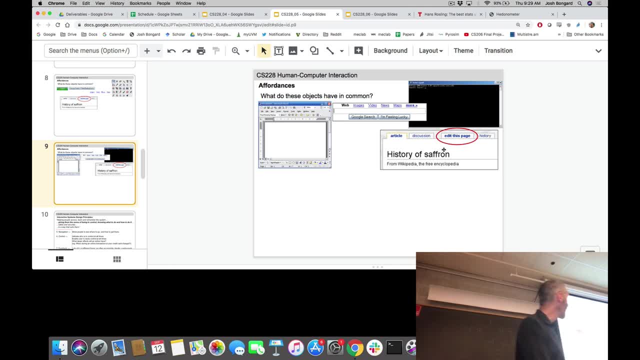 cursors, some of them are buttons, some of them are entry bars. they're all sort of different from an HCI or sort of widget point of view, but they're all projecting the same affordance, which hopefully you realized immediately, because they all have that one affordance in common. right again, the affordance that you see, or the 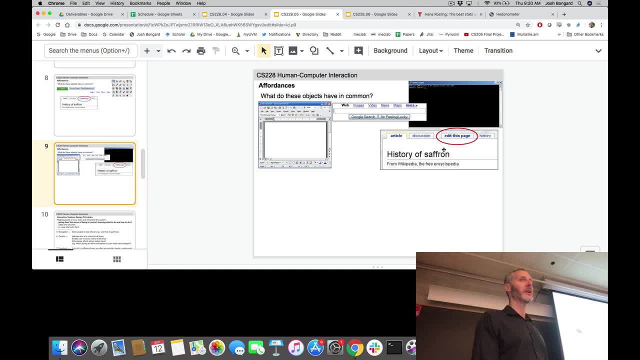 that's projected by the object is influenced by what else is going on around. what are some affordances you might build into your leap motion educational software? how might you show something on the screen which projects your advertises what the user should be doing? I will put a picture of a panel. 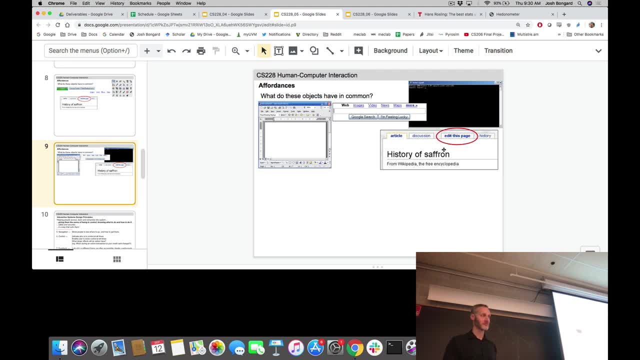 next. so everyone knows that the hand is related to the operating object. picture of a hand, a photo of an actual human hand, a cartoon one? okay, so I see a cart- I never used the leap motion device before, I don't even know what it is- and I see a cartoon hand on the screen. what is the affordance that it's? 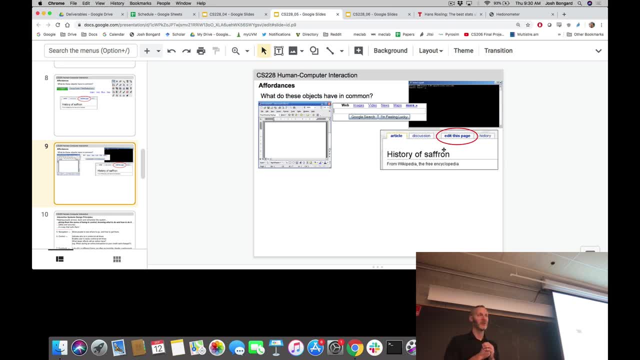 projecting. put yourself in the shoes of this naive user. they see a virtual hand on the screen. they see this cigarette lighter that's sitting on the tabletop. maybe grab it right. so that's so. this is. this is part of the design process. right from the point of view of the user. what affordance is being projected by the? 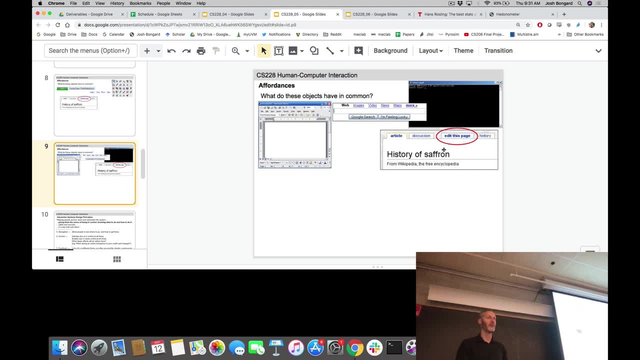 combination of the physical device and what they see on the screen. yes, there's a great idea, right, the Wi-Fi symbol. so most people know that, at least in the western world, this is not. this is not a volcano, it's a wi-fi signal. it means there's something. 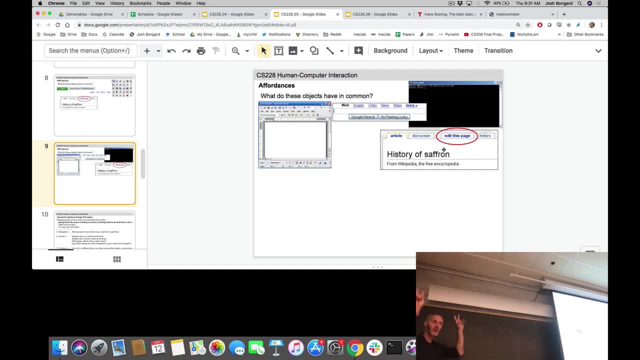 wirelessly being projected from this thing. this thing- quote unquote- sees right, and if you put a little virtual hand over it, ah, this thing will see my hand. i have no idea what it does with that information or what about my hand- it sees, but that is probably an unambiguous affordance. it's a good. 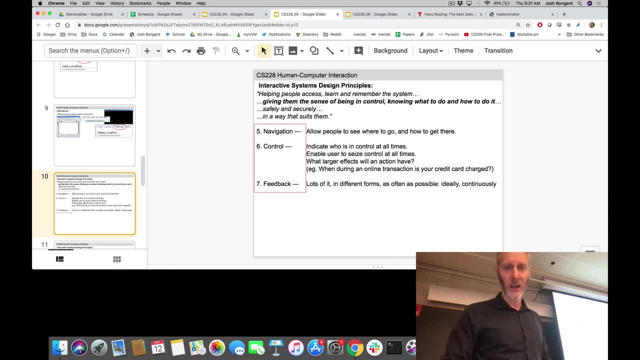 that's a good idea. that's the idea. okay, all right, let's push on. um, we'll spend a fair bit of time next week talking about navigation. right, i'm at this point in the software. where am i? where have i been? where can i go right? so communicating, communicating, navigation. 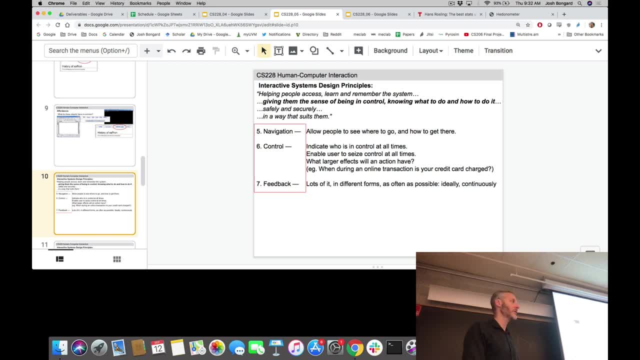 is is can be challenging in certain kinds of software. we can obviously put up, you know, a menu hierarchy here, the options that you have at this point point. or you just got a badge: you passed level K. you can imagine where you're going. next you're going to level K plus one. what are some of the creative ways? 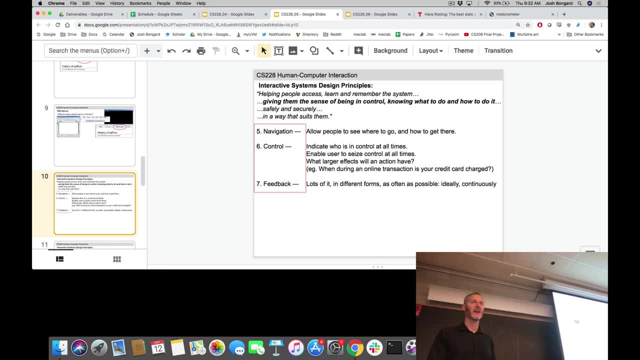 that software systems you're familiar with communicate or give hints about navigation. where you can and can't go: great out boxes right. anything that's great out is not available to you. you get the buzzer right. you did something wrong or that's not. you can't go there. 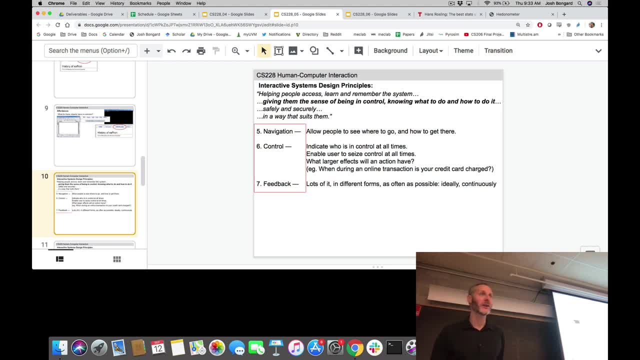 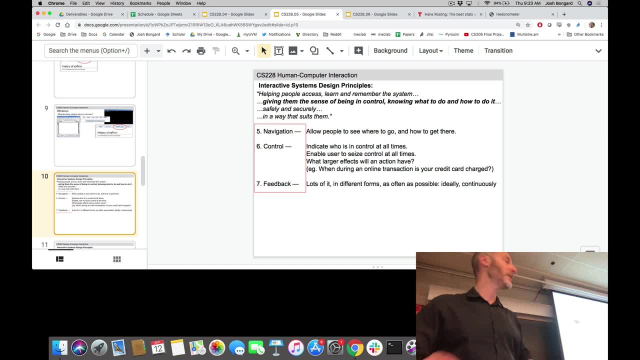 a bowl or you can't walk to there. how do they communicate where you can go and where you can't go in computer games? sorry, can you say that again? okay, okay, absolutely right. so it's flashing red. you're going in the wrong direction, right? that's another important part of navigation. other ideas: 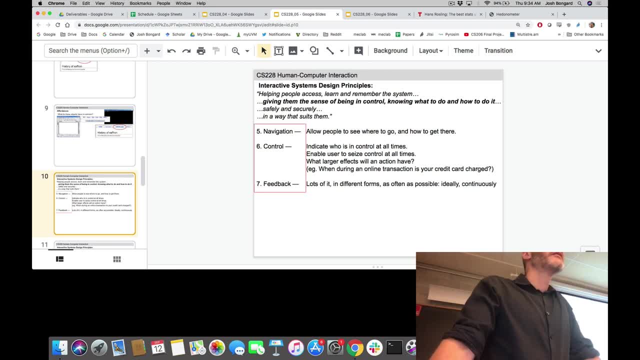 okay, okay, okay, okay, okay, okay, okay. that's right, they make it visible, right. so there's a cliff there, there's a wall, you can't go any further. in the early days of computer games, a lot of the objects had like a, like a light around them, like an aura, they kind of you could. 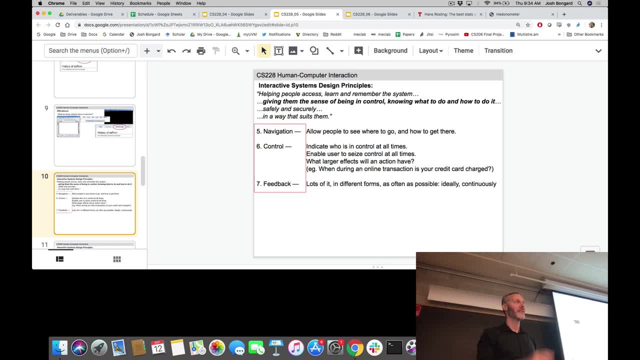 tell that that was different from basically the background art and that was something that you could interact with. wasn't always obvious how you could, but you could right. you could go over there and pick up or inspect that object. that over there is just a pretty picture, it's background art. 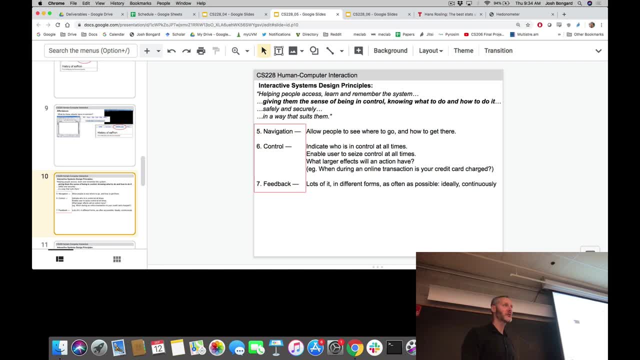 okay, we mention the spinning wheel of death already. control is pretty important. all right, again, it can be very important if it's a real-time system. you're operating something. who is in control? it should be at least visible who is in control at a time, at least the spinning wheel of death. 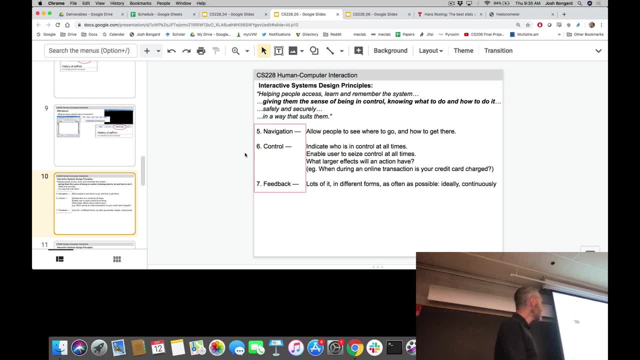 that says it's not you, it's me. right, the worst, the most, one of the most frustrating experiences to have his users. you're not sure who's in control. right, there's a lag in the video stream of the website because why you're not here. then I could die tonight. I know what actually happened because he said: 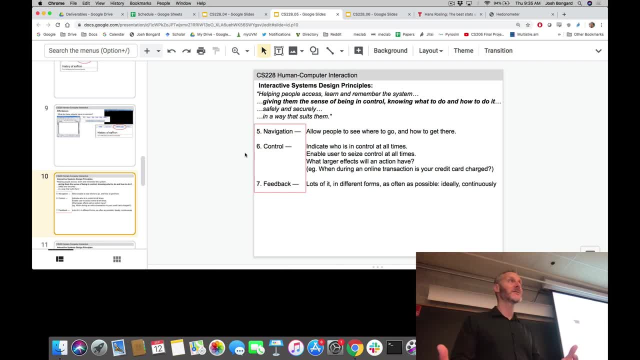 or the website. nothing's happening. should you wait? is it going to start moving again? or do you need to reset or reload or turn off and turn back on? i don't know who's in control. in the early days of e-commerce, you know you were marched through these steps and exactly when was your credit card going? 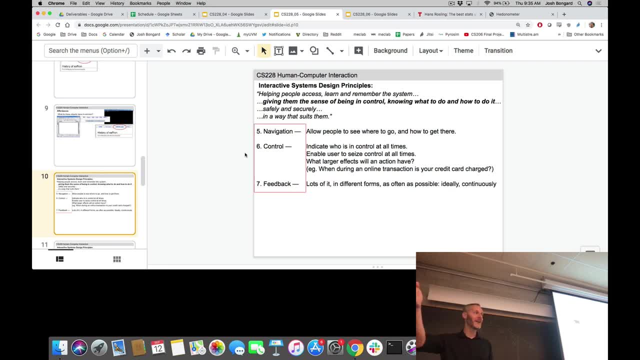 to be charged and as that point is getting imminent, can i turn back? when can i cancel a charge that's about to occur to my credit card? pretty important feedback. as you can imagine, this one's kind of controversial. we want to make the system visible and helpful, so we'd like to 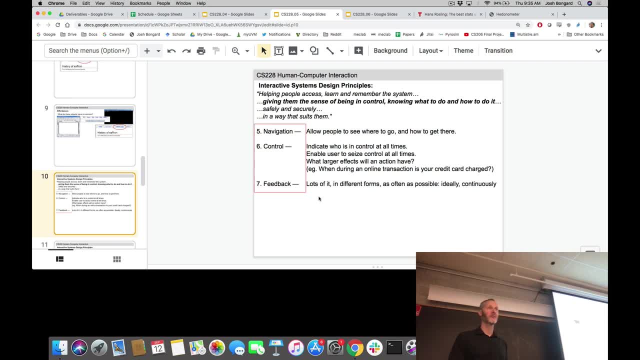 provide lots of feedback in different forms as often as possible, ideally continuously. do you agree, disagree, not too much. how much is too much so? um, there's a really good example of a tweet. i saw you where a flight. you know when your flight is arriving. 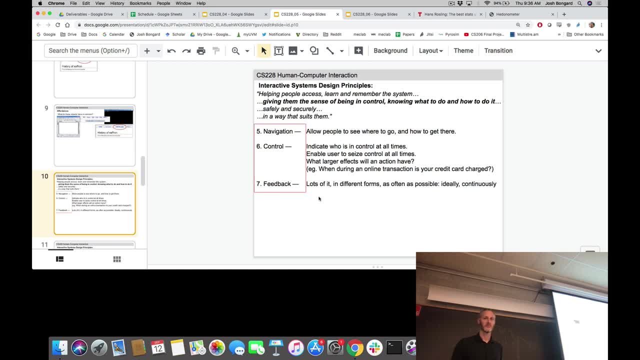 they were busy or they had to change and they're giving notifications, but the particular app gave too many notifications, so it was like 23 within a half an hour. Gotcha, And a user doesn't want that much push notifications. You're trying to get on a flight? 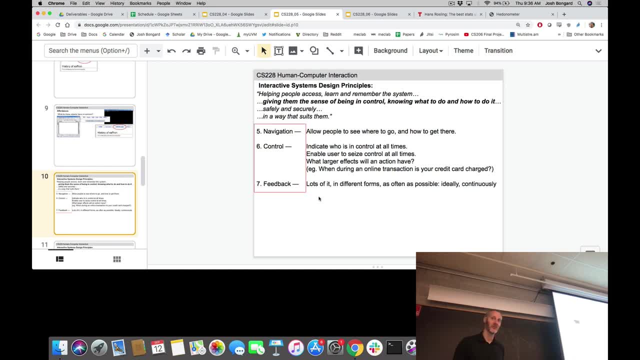 and it says it's been pushed back two minutes, another three minutes, another three minutes, another three minutes, Exactly All right Depends, though I can imagine there's some people that really care, Or it's tricky, right Tricky to get this one right. 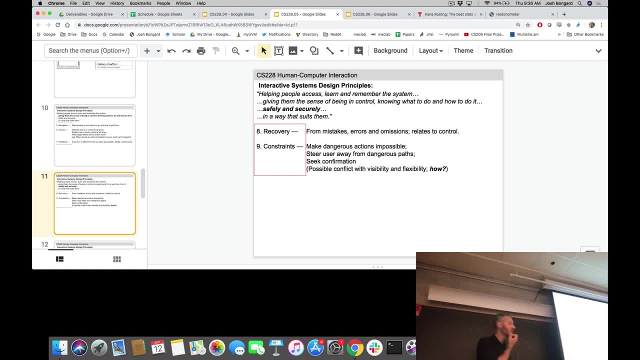 Okay, Safety and security. Safety and security- this one's also tricky to get right in HCI. There's lots of different ways we can try and prevent the user from making mistakes or errors, and we can break them into reactive and proactive approaches. 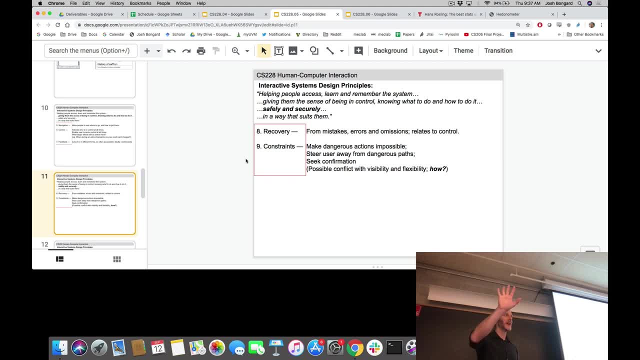 So proactive approaches. we're going to try and add constraints to keep keep people from making that mistake in the first place. There's a virtual cliff. I'm advertising to you up front: Don't go over there. Retroactively, we're going to assume that it's allowable. 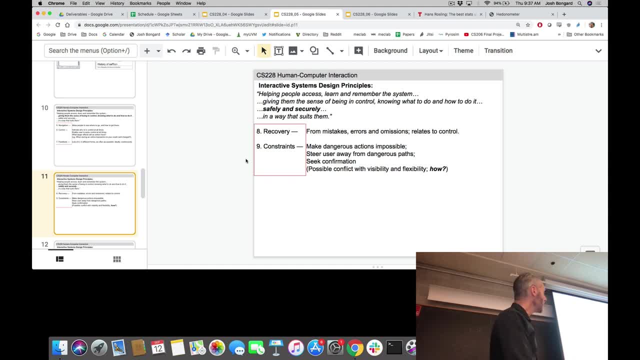 for users to make mistakes, but we'll make it easy for them to undo those mistakes after the fact. When might you want to use retroactive? retroactive safety versus proactive safety? 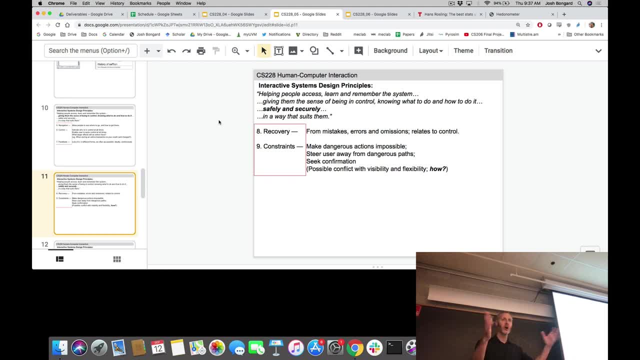 We'd like the user to have a sense of flow. you just go write or fill in what you need to do and, if you want, you can go back and correct things later. right? People have very different writing styles. some people like to write very carefully. 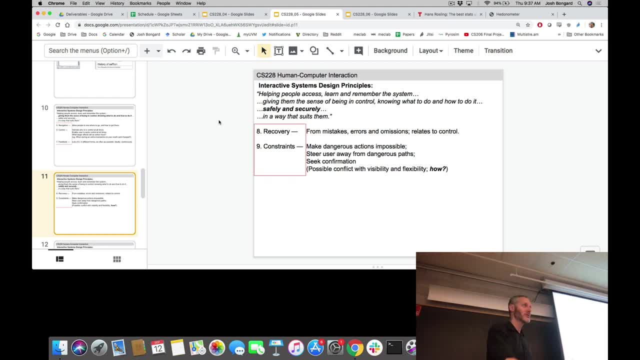 Others prefer, from a creative process point of view, to just write as quickly as possible and fix things after the fact. Imagine a word processing document that the moment you made a spelling mistake, you're not allowed to write any more text until you fix the spelling mistake. 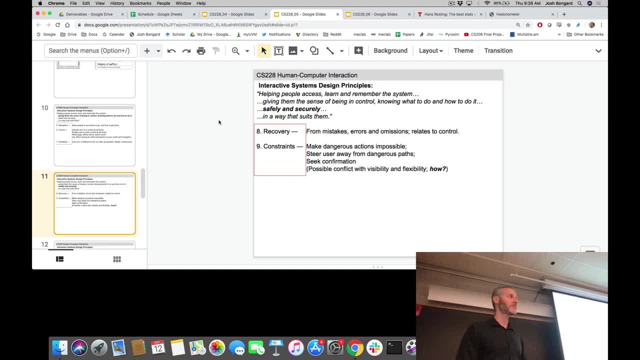 For most people probably not very acceptable. Where do we want to be proactive rather than retroactive? 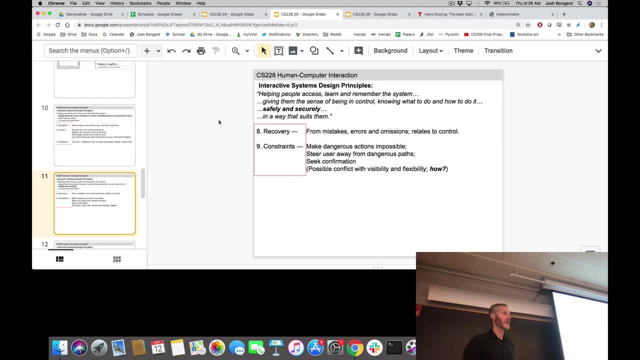 Absolutely. that's a great example. We predict where you're going is dangerous and we're predicting. you probably didn't know that's where you were trying to go. We may be wrong. you may actually want to go there. we're just letting you know. 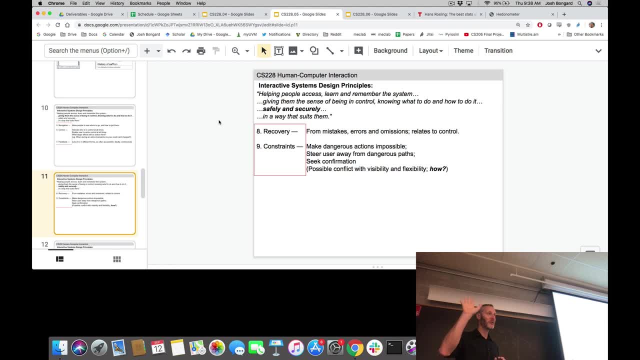 The content might be unsettling for some people. You can't really undo it once you've shown the content. absolutely yeah, oh, that's interesting. so this is teaching coding- a regular typing gotcha. okay, teaching typing. that's an interesting example. okay, so again we 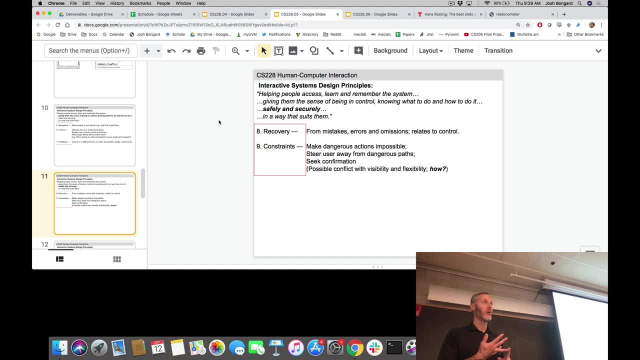 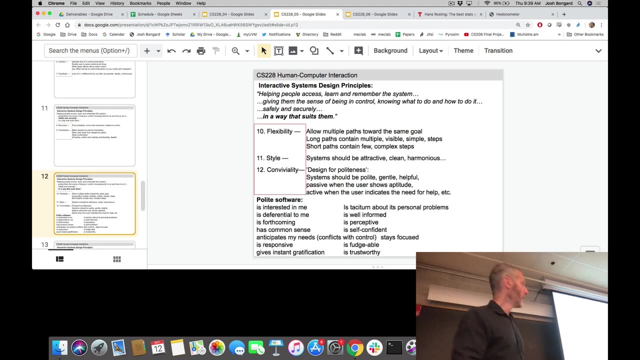 need to think carefully about who's using who's using the system, what activity are they performing and in what different contexts, and that might dictate the way we go about trying to make the system secure or easily fixable, and so on. okay, but last, last three here. we often want to make our system. 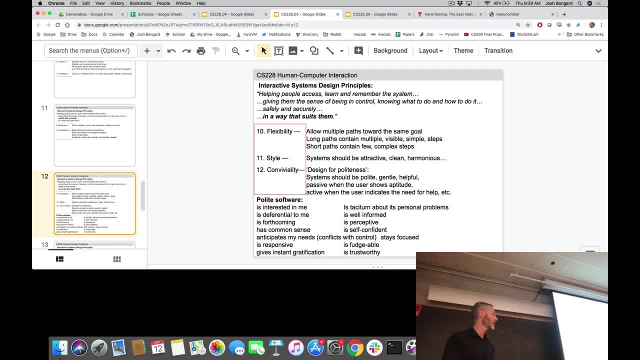 flexible because, again, we're going to have very different users using our system. for the beginners, we might want to create very long pass from A to B. so we have here. we have a system under the code. here we have a system that's actually system, that isn't very efficient. There's lots of steps they have to carry out to get from point A. 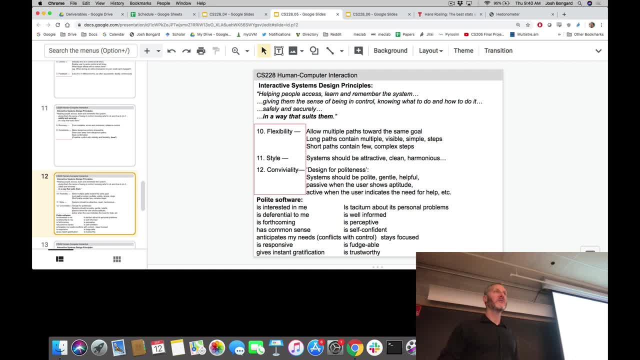 to point B, But each of those steps is very visible, obvious, easy to recognize, easy to learn. So lots of short, simple steps, But for our advanced users, we want to allow large jumps. Each one of those jumps may be complex, but we're going to assume that in order for our system to be. 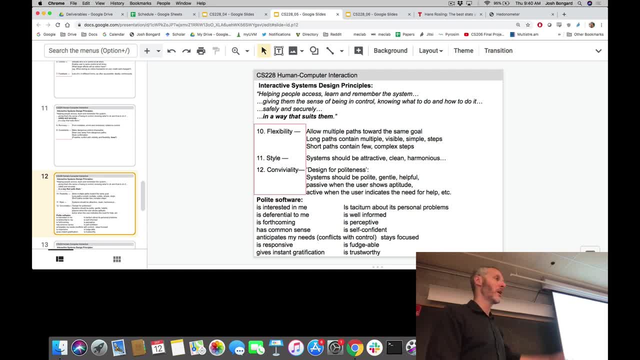 acceptable to advanced users. they don't want us to hold their hand, They want to run ahead. What are some examples of technology that provide those two different kinds of paths, and how do they do so? When you are using the navigation system, there's some voice that guides you to turn left and right. 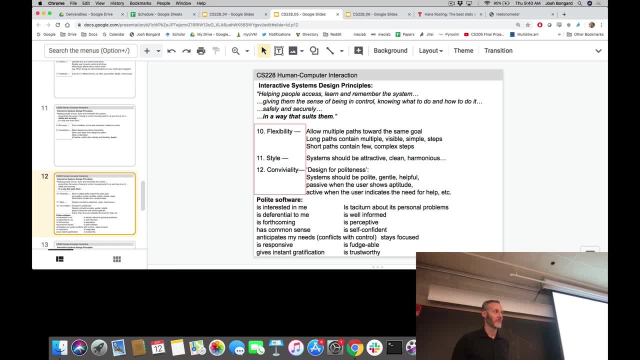 and you can set it. There's none, there's limited, there's normal. For GPS navigation: yeah, When you're driving a car, if you are new, you need a lot of details. Yes, I guess that would count here. That's sort of more. that's about more or less notifications. 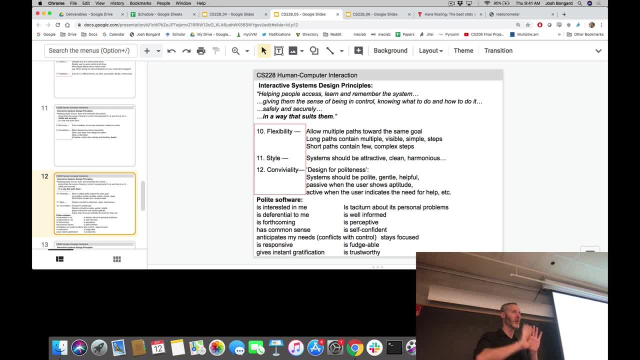 What we're looking at here, where the system gives you lots of small steps or large jumps from one to the next. Well, perhaps when you're looking down the road, I mean, it pops up a tip sidewalk. Okay, And users might like that You can show them more processes for advanced users walking. 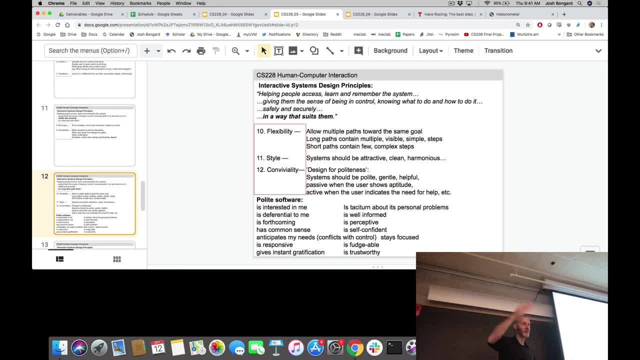 Exactly right. So it would pop up lots of those and say here's sort of the tips about how to get from point A to point B for an advanced user. get rid of it altogether, I know how to get there. Maybe that fits with your example as well. 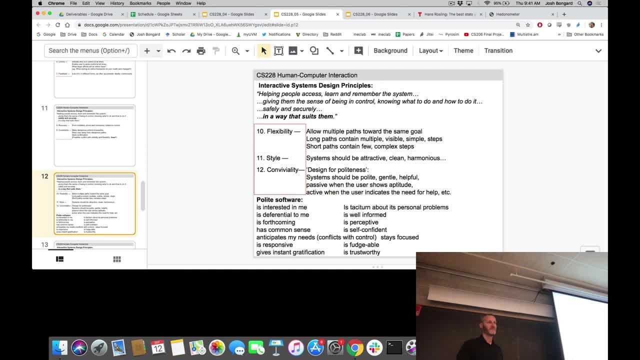 Duolingo again, you know enough of the language. you can jump to wherever you know it and you have to take a test to prove that, or you have to take all the steps going up to Absolutely. So in an educational system like Duolingo it's adapting right. 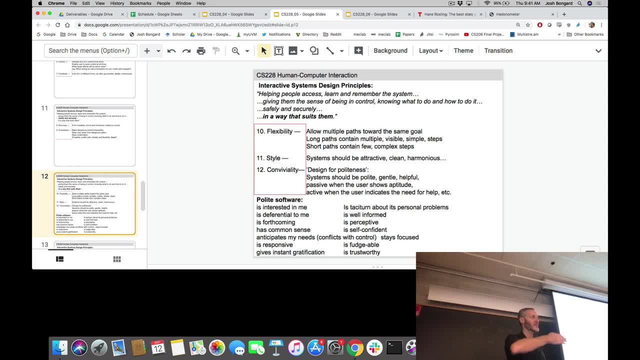 It gives you little mini tests and allows you to jump further ahead if you pass the test. You didn't ask that, Absolutely right. So if you're new to Git, you might want to go to GitHub and click on things and do everything through the website, which takes a lot of clicks. 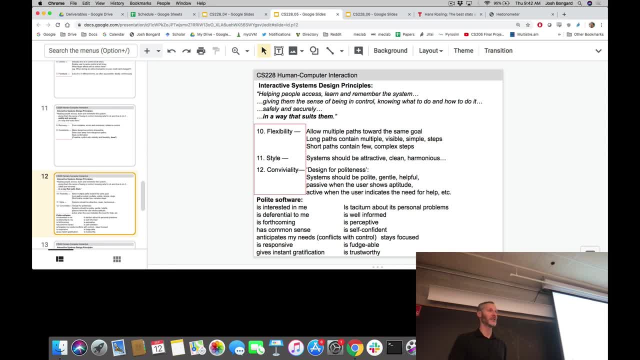 Once you start to learn Git, you can do things locally on your own machine at the command line. That's a good example. Keyboard shortcuts, right Menu hierarchies for the beginners, keyboard shortcuts for the advanced users- Okay, lots of examples there.